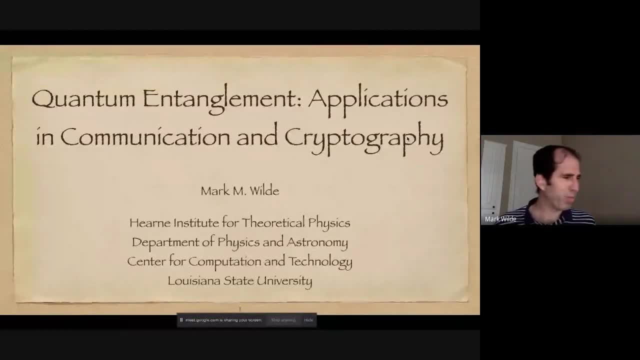 All right, So can you remind me how much time I have? You have around 1 hour and 15 minutes. 1 hour and 15 minutes, Okay, Please keep me on time. Yes, sir, Please let me know when there's 15 minutes left. 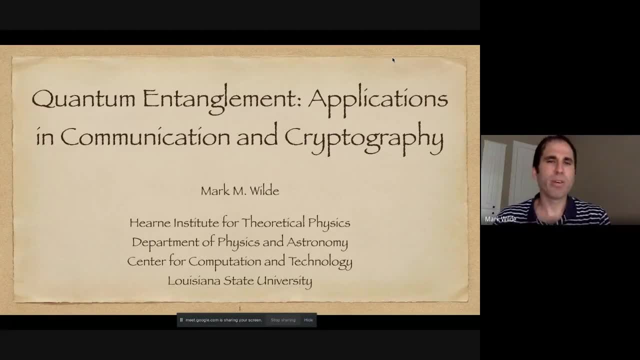 Yes, sir. Okay, So today I'm going to tell you about various ways that quantum entanglement appears in quantum information theory, with one of the main goals being to distinguish between the classical and quantum theories of information. So I'm going to start with. 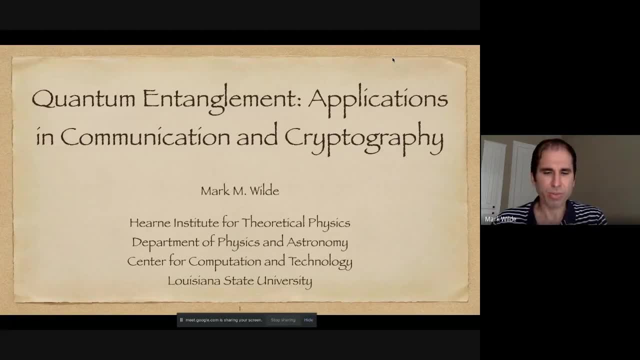 some things that might be pretty basic for some in the audience, but maybe for others it will be new, I don't really know- And then we'll move on to more advanced concepts. Okay, But the goal is to show how entanglement arises in a variety of communication scenarios. 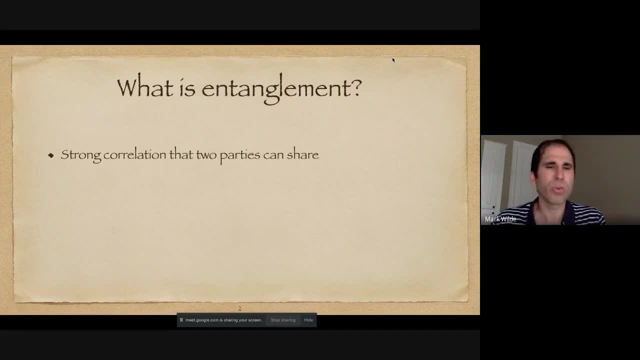 All right. So, first of all, what is entanglement? It's a strong correlation that two parties can share. Indeed, as I said earlier, it's a key phenomenon that separates the classical and quantum theories, And it's something that cannot be created by local operations and classical communication. 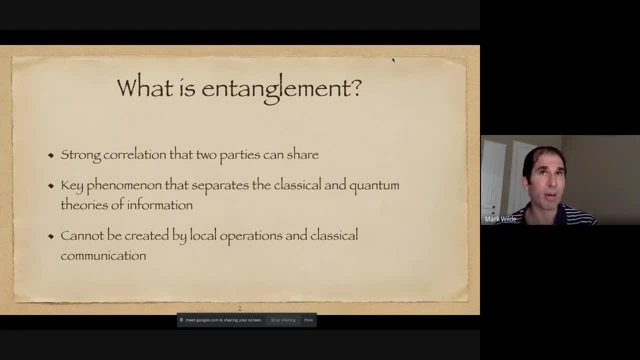 So the scenario we imagine is that Alice and Bob are located in distant laboratories and they each have fault-tolerant quantum computers and they're allowed to exchange classical data, And so if they share some entangled state, to begin with under this class of 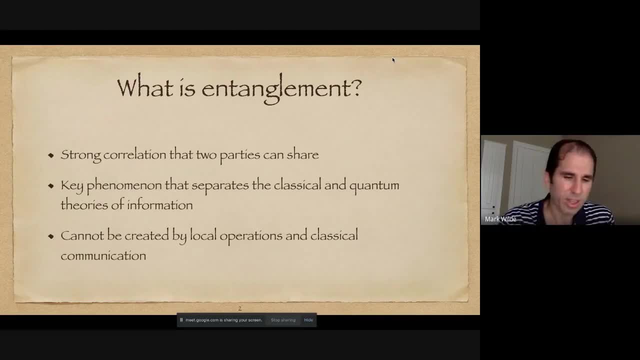 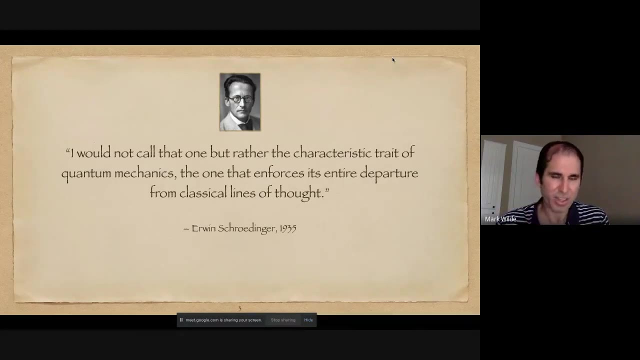 operations, the entanglement cannot increase, And so entanglement is a resource in this sense, and this is the resource theory of entanglement. So this is a famous quote of Schrodinger, in case you might have seen it before, but he considered many years ago the idea that quantum 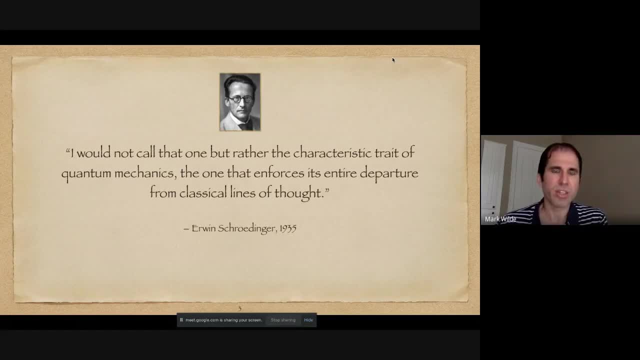 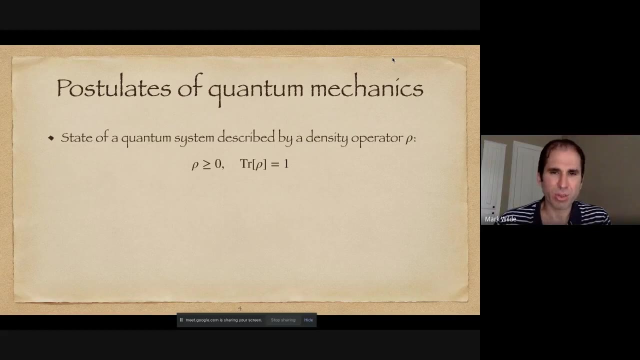 grant was meant to be a distinct trait, a characteristic trait that enforces the departure of quantum mechanics from classical lines of thought. Okay, Just some basics to begin with. What are the postulates we're going to be dealing with? A state of a quantum system is described by a density operator. 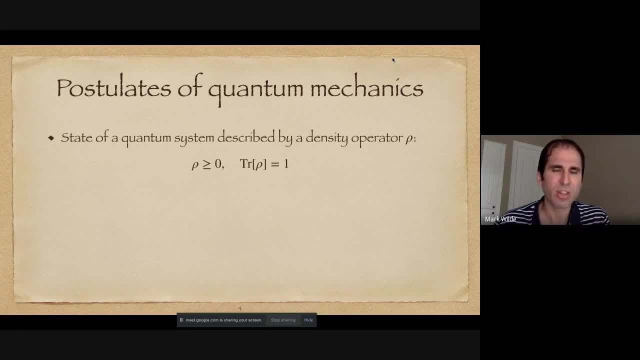 a positive semi-definite matrix with trace equal to one. The positive semi-definite constraint is that all the range has one unit, And so the Poiseux's DC of two is simply one. This is not just two. eigenvalues are non-negative, and the evolution of a quantum system is what we 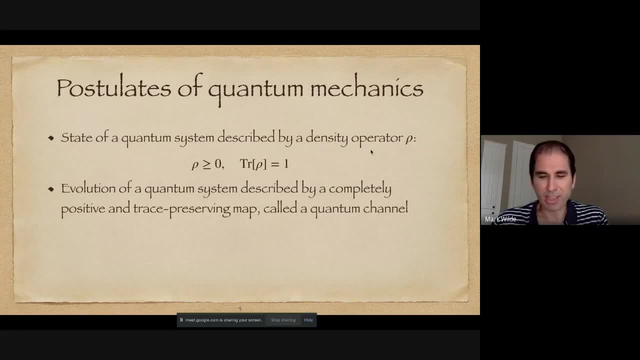 call a quantum channel, and mathematically that means that it's described by a completely positive and trace preserving map. so so the basic requirement is that a quantum channel evolves a quantum state to a quantum state, so it preserves the property of being positive, semi-definite, and it 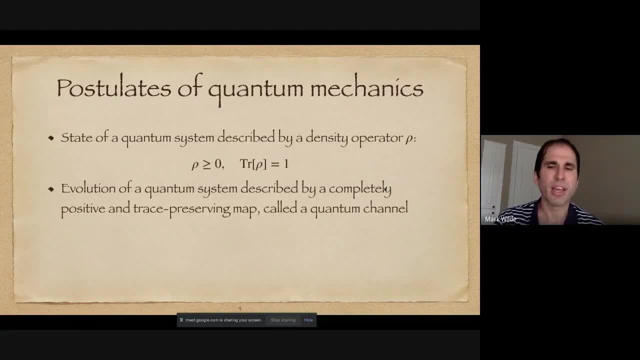 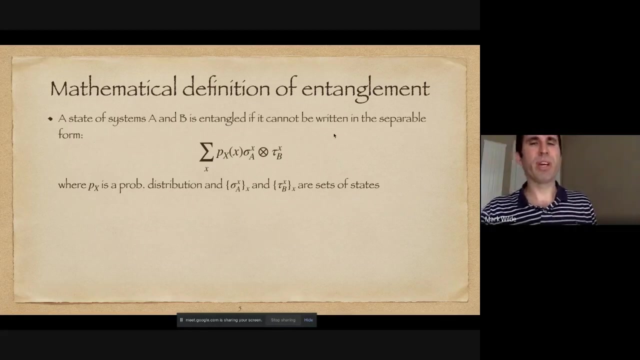 preserves the property of trace being equal to one, and the same is true if the channel acts on one share of a bipartite state. okay, and that's the completely positive. okay. and density operators can act on tensor product Hilbert spaces- okay. what is the definition of entanglement? we define. 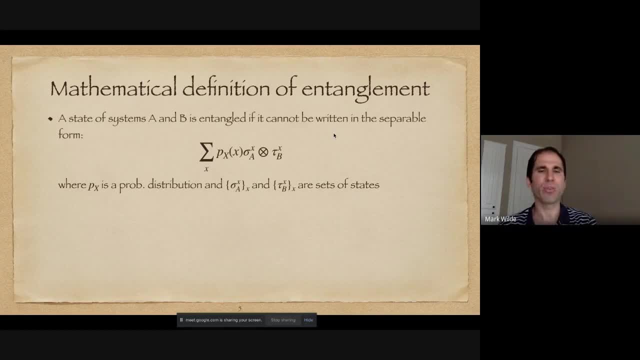 entanglement as a state of a quantum state, and it's a state of a quantum state, entanglement in terms of what it is not. so if a state can be prepared by local operations and classical communication alone, it has this separable form and it's 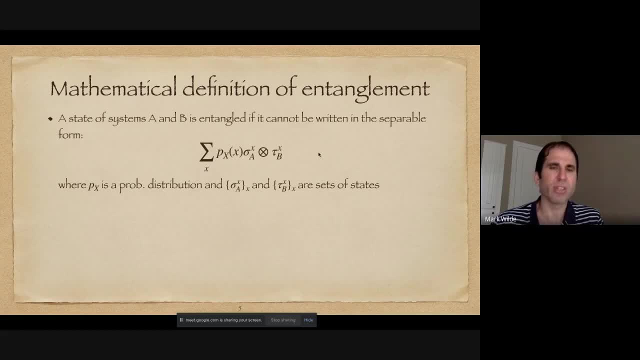 said to be a separable or an entangled state. so the way you interpret this is that in the background there's someone who flips a coin or throws a die. according to this probability distribution, a classical outcome X occurs, and that's what we call a quantum state. and that's what we call a quantum state. 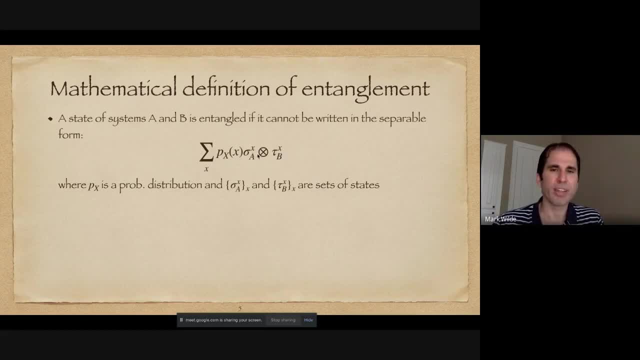 occurs, that gets communicated to both Alice and Bob, who then prepare states locally- Sigma X and tau X- based on the classical letter, and the state that they prepare based on the classical letter is a product state, and if they then discard the classical outcome, the state is a probabilistic mixture of these product. 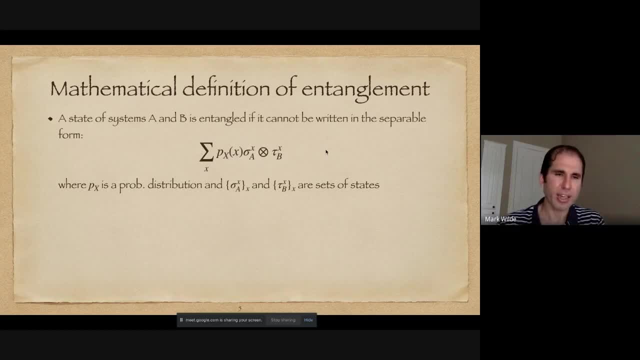 states. so that's a separable state and you know a state is entangled. if we cannot write it in this form, okay. and one thing I'll mention. it's not on the slides, I think, but it's an interesting question in computational complexity theory. if you're given a 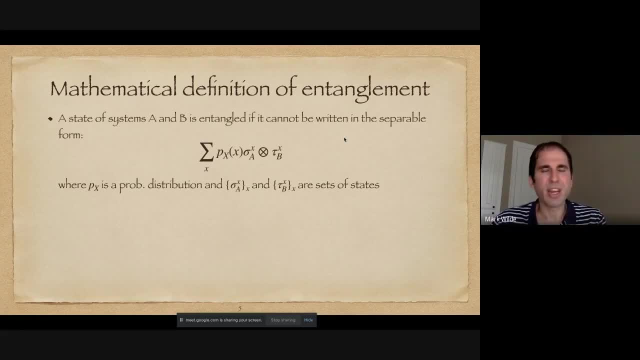 description of a density matrix to try to decide if a state is separable or entangled, and In that sense that problem is known to be NP hard. so it's a. it's a hard problem computationally and that's one of the reasons that entanglement theory is. 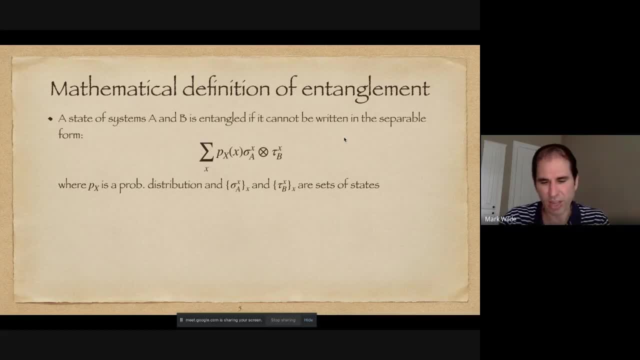 challenging because if we want to actually decide whether a state of separable entangled already, that's a computationally difficult problem. the difficulty extends even if you change the way the the quantum state is described. so if you instead say that the bipartite state is general, no, as opposed to a subject from the quantum state to crisis. instead of the quantum state, you mightănade to actually very often determine that the state can't Soup in status if this property isу. 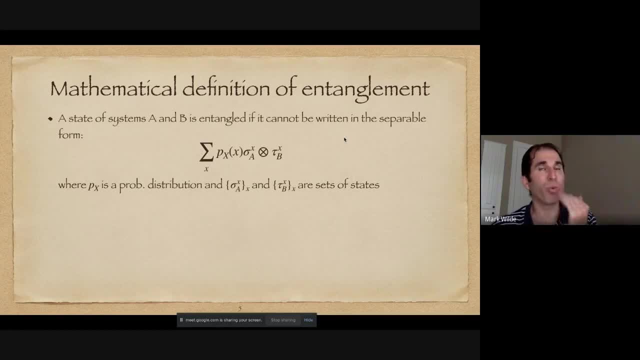 become more Rand. you could just write that this form is rather forbidden in the rest aspect. asu generated by a quantum circuit, and you measure complexity in terms of um, the number of quantum computational gates needed to prepare the state. it's also known that it's it's hard for for this. 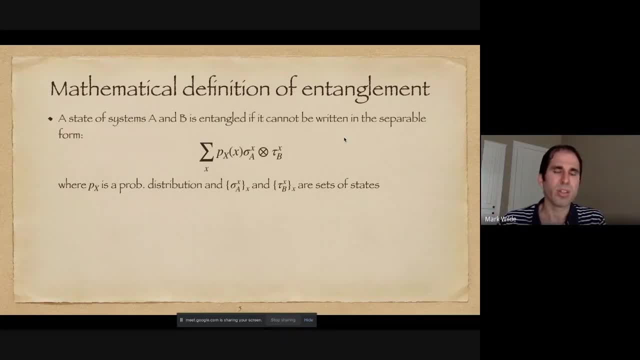 version of the problem. it's hard for a quantum computer to decide if a state is separable or entangled. okay, so those are just some things i'm mentioning in passing which i think are interesting. um, and indeed, these separable states can be prepared by locc and entanglement cannot be created or increased by locc. 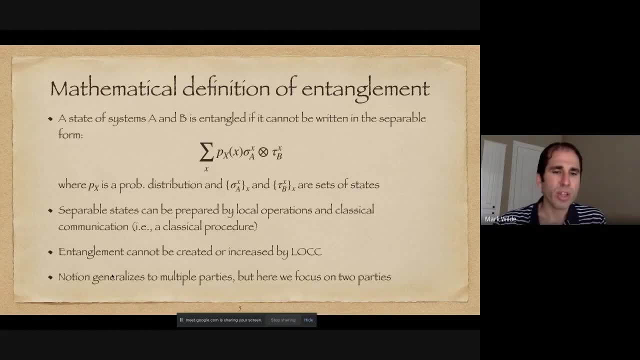 this notion generalizes to multiple parties straightforwardly. so if it's alice, bob, uh, uh, you know. charlie and dan, you know, just pick some random names, then a separable state for a multi-partite- uh, for a multi-partite state- can be prepared by locc and entanglement cannot be created or increased. 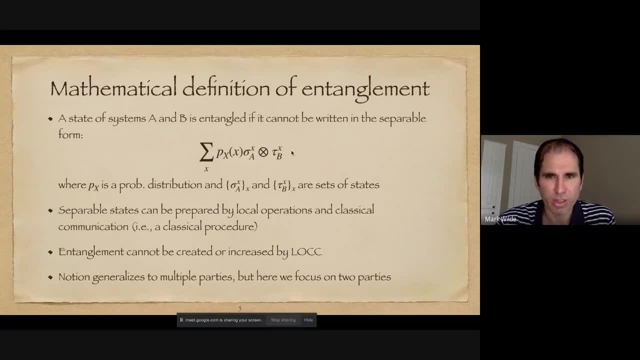 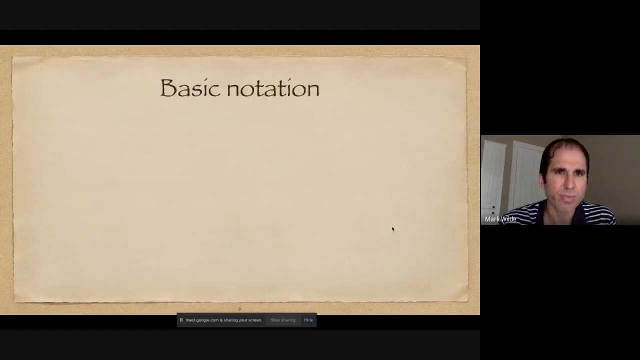 multiple parties would be extra tensor products here, right, like we have a tensor omega xc, you know, tensor uh, rho, xd, etc. okay so, but throughout the talk we're going to focus on the bipartite case. some basic notation i'm going to use throughout the talk. i mean, you probably 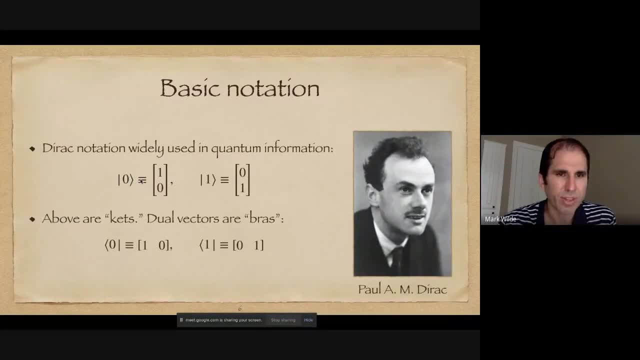 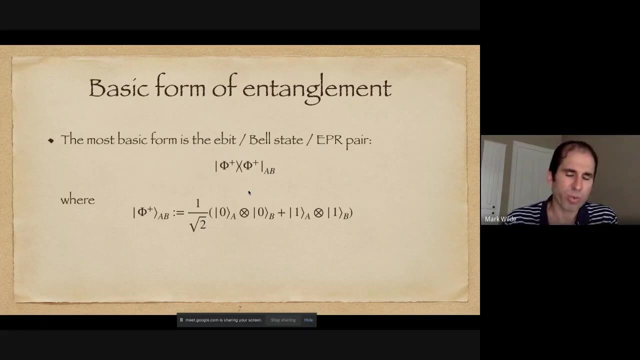 know this: um, the the rock notation. so classical, zero classical one are these vectors and the cats are the. the bras are the dual vectors. okay, so what is the basic form of entanglement? it's the ebit. we. there are different names that it goes by, one of which is the ebit. 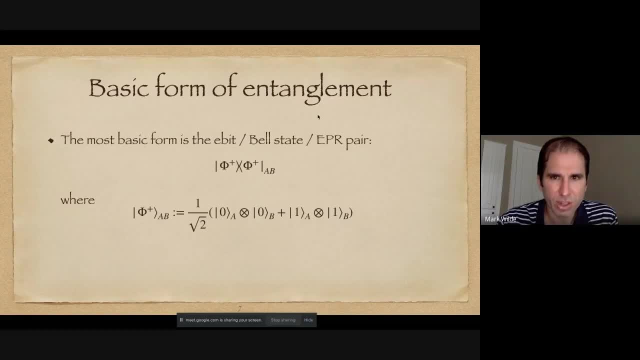 another of which is bell state, another which is epr pair, and it's this five plus. so this is the density matrix for the entangled state. you have to excuse me, there's there's yard work going on in front and i can't do anything about it. i'm sorry about that. 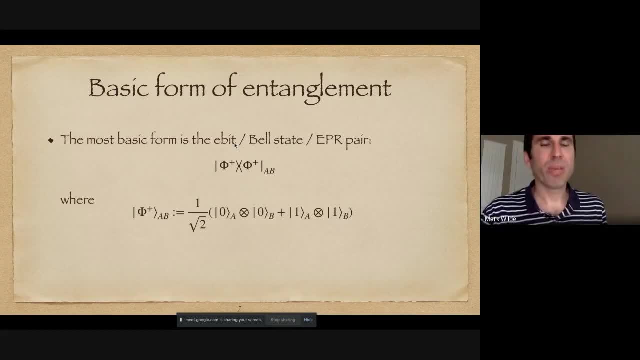 um, okay, so the basic form is this: ebit, this is the density operator. so you, you get the density operator by taking the ket and the bra and gluing them together using the outer product. and um, phi plus is this state vector. so it's this uniform superposition of zero, zero and one one. 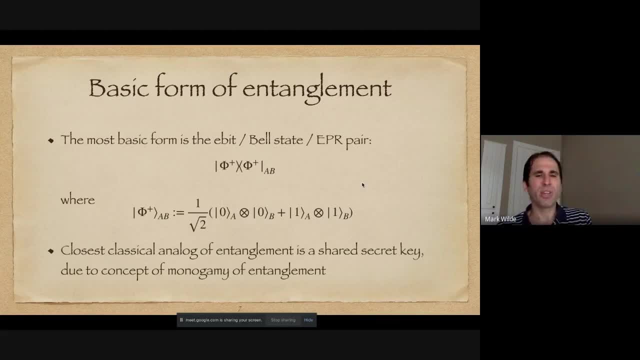 okay, so that's a basic resource. if you're interested in what is the closest classical analog of entanglement. it's arguably a shared secret key and that's due to a concept called monogamy of entanglement. what is monogamy of entanglement? the principle states that if alice 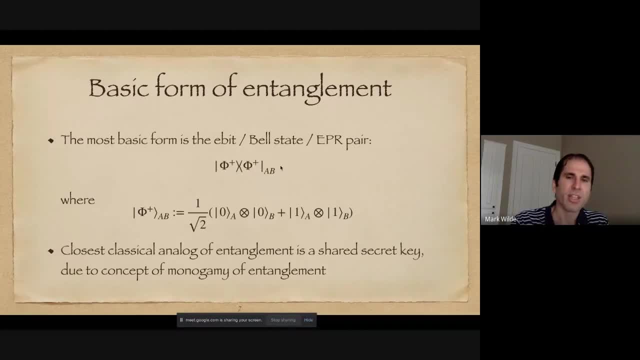 and bob are in this entangled state, then it is impossible for alice to be entangled with a third party like eve. usually we call it third party eve in the context of cryptography for short for eavesdropper. so, um, due to this monogamy, the correlations that, um, uh, alice and bob share are are theirs alone, and 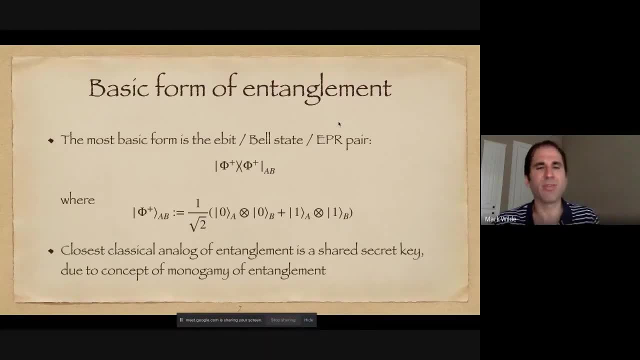 not for any other third party, and so that's the sense of secrecy. and in fact, you know, if this is the case, if in some protocol alice and bob can truly prepare this maximum entangled state, then they can perform local measurements on it to extract the secret key and be guaranteed. 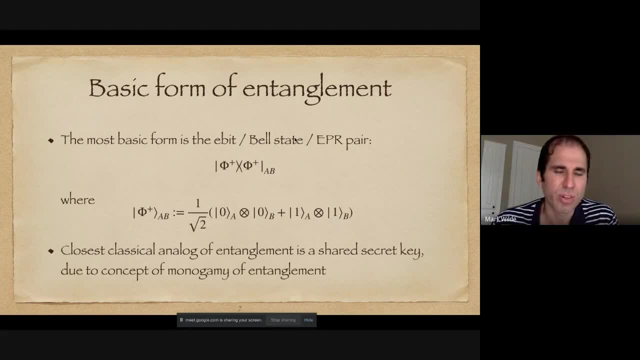 that that secret key will be secret from anyone else in the universe? okay, according to the principles of quantum mechanics? um, so you know, a secret key has those properties, right? so secret key is something that is uniformly random. So if you do measurements on this maximum entangled state, the outcomes will be uniformly. 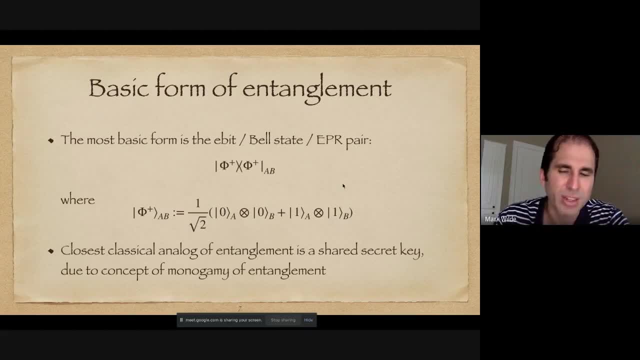 random if you measure in the Pauli sigma Z basis And the outcomes will be perfectly correlated. that's the 0011, the same as what we would like for a secret key And any third party. what they would measure is independent of the measurement outcomes. 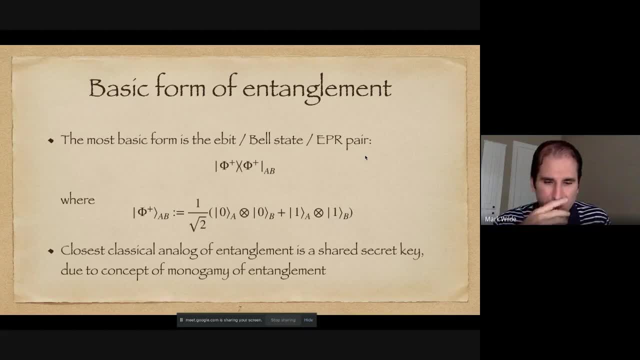 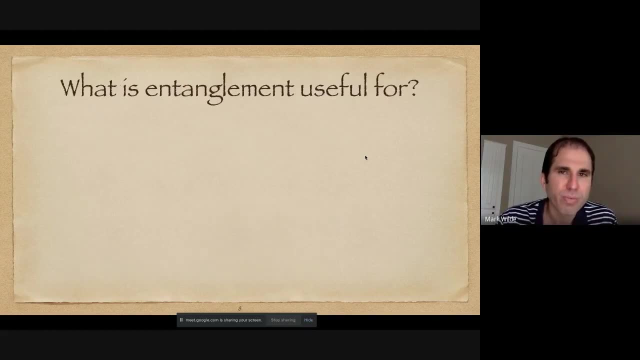 of Alice and Bob. So a shared secret key has all these properties And from a maximum entangled state you can get a secret key, but the opposite is not possible. All right, what is entanglement useful for? I'm going to talk about three things. 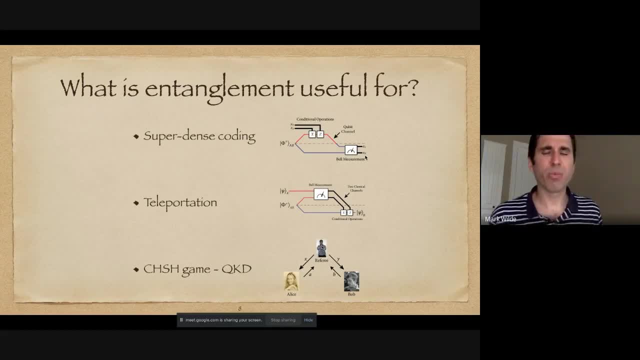 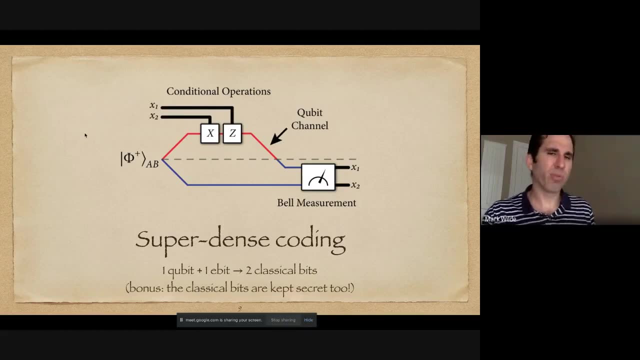 These are basic things you know, just to get us going. You've probably seen these before, So I'm going to spend a few minutes on each of them. Superdense coding: this is a basic protocol that was discovered in 1992 by Bennett and. 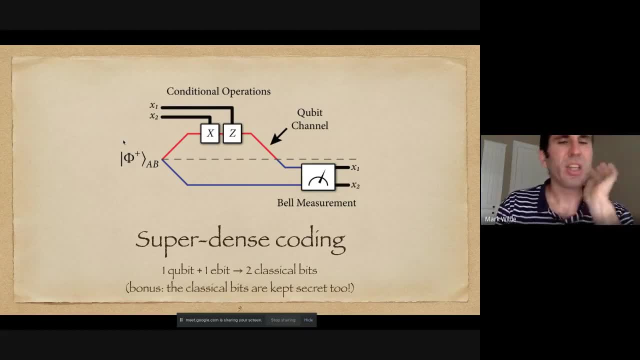 Wiesner, Published in 1998.. Published in Physical Review Letters. And the assumption of the protocol is that this dashed line indicates like a physical line denoting the dividing line between Alice and Bob's laboratories. Okay, And so we assume that beforehand, one share of an ebit is communicated to Alice's laboratory. 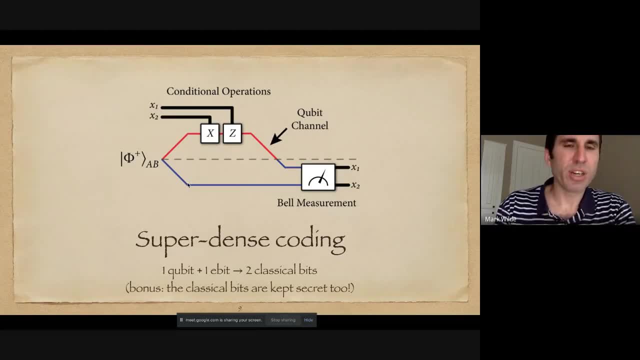 maybe via a quantum channel, And another share is communicated to Alice. Okay, All right, So let's look at some of the other pieces. So if Alice sends two bits to Bob's laboratory, So they start with this ebit as a resource. 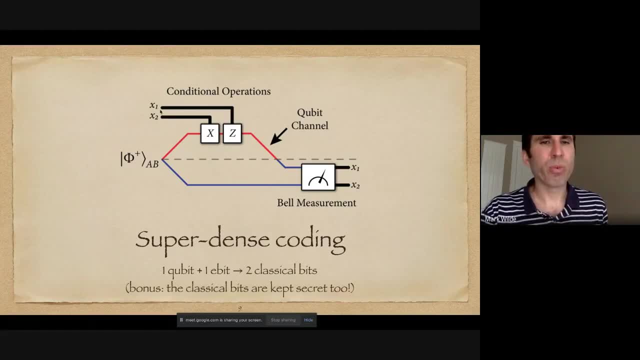 Okay, And then Alice performs. you know she wants to send two classical bits to Bob, So she performs these conditional Pauli unitaries sigma x, sigma z, abbreviated as x and z for short. And what that will do is it will rotate this Bell state to one of the unitary bits. 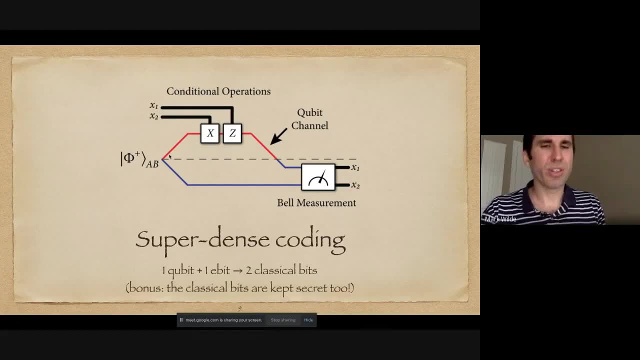 So this is the Bell state of four orthogonal states. okay, and I don't have the notation for those states written on the slides, but I'll just say that they're called the Bell states and they're orthogonal. they have the property that if you trace over one 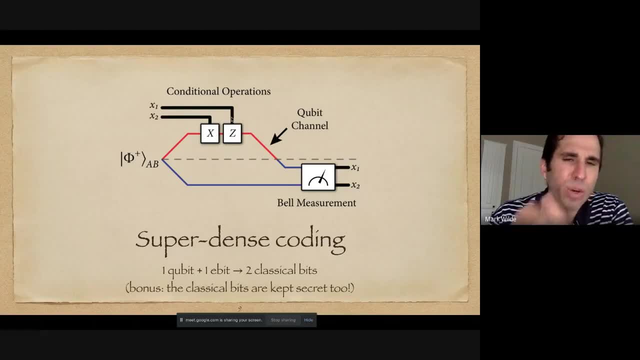 chair of them, you always get the maximum mixed state anyway. so Alice can, by performing these local rotations, change the global state and then if she shares, if she sends her share of the EBIT over a perfect qubit channel, then Bob can perform a Bell measurement to decode the classical messages x1 and x2. so we can. 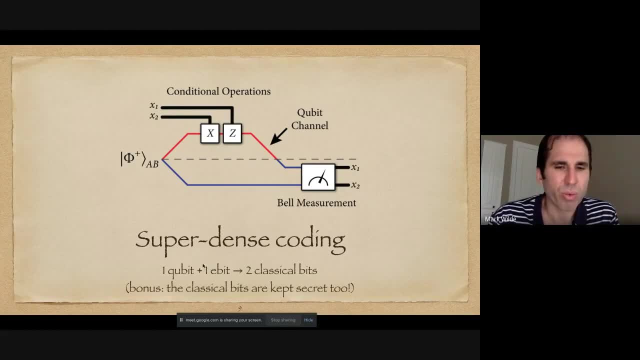 summarize this in terms of a resource inequality or a resource transformation. excuse me, the lawnmower is right in front. okay, now we went away. so the the resource transformation is that, by means of an EBIT and a qubit channel, you can transform these non-local resources into two classical bit channels. so if we draw, 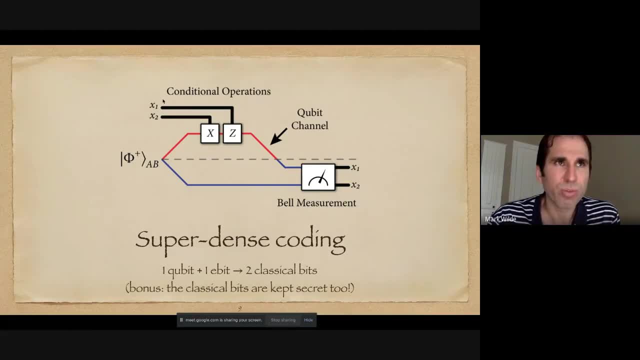 the box around the whole thing. then we have two. we have two classical bit channels. another thing I want to say is that the classical bits are kept secret. there's a sense in which there's a secrecy, property which I don't know. I know people often think about that. so, due to the fact that I stated earlier, suppose 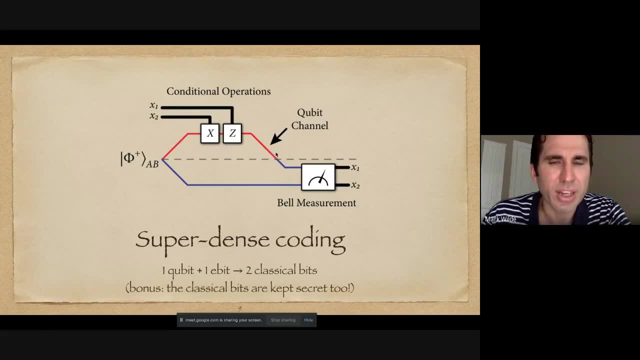 there's an eavesdropper right here tapping the line and trying to figure out which message Alice encoded then when, with access only to this qubit and not this one, no matter what the classical message is, the local state of Alice's system here will be a maximum mixed state, and so it's impossible to figure out which. 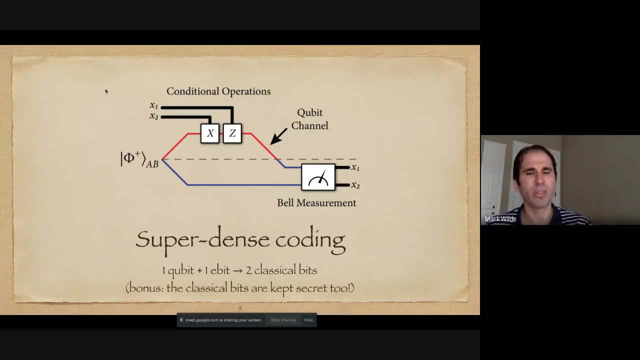 classical bits were encoded into the quantum state. so you have this secrecy aspect as well and you know, one of the things that's going on worldwide, and I think as well as in India, is the goal to build quantum communication and quantum communication networks. right, and so one of the basic things that people are 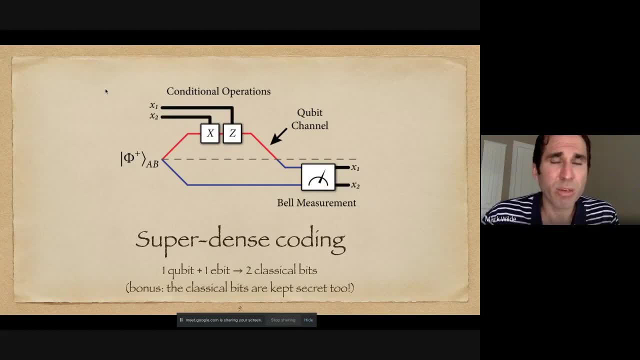 trying to do is to figure out how to distribute entanglement on a large scale, and so then, if you had this entanglement, you would be able to do protocols like super nance coding and you would have this secrecy as well. so you know, that's a. 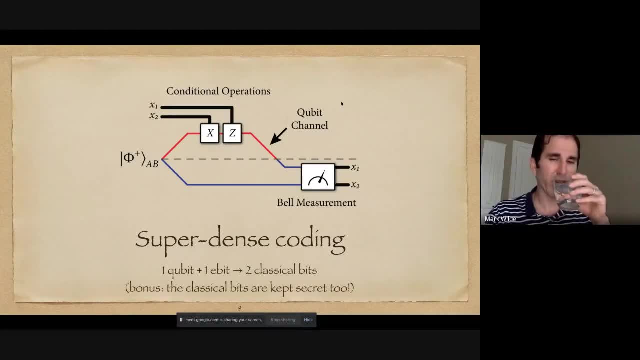 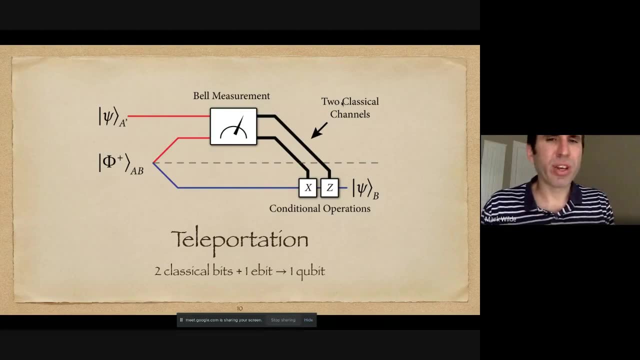 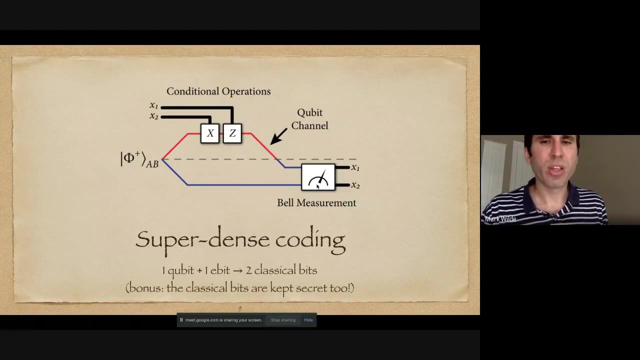 major effort going on worldwide, worldwide, right now. okay, a year after super nance coding was discovered, teleportation was discovered and if you look at this diagram and compare it to the previous one, you see that kind of what we're doing is we're taking what Bob is doing and putting it in Alice's laboratory. 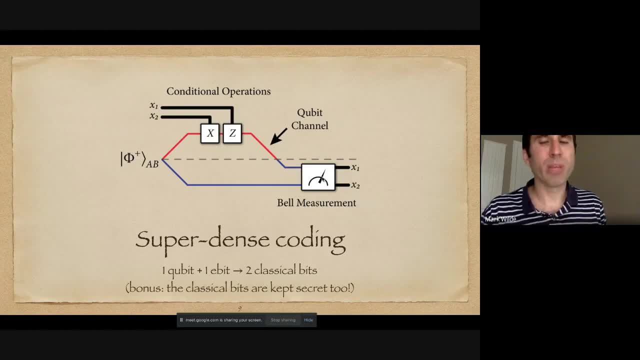 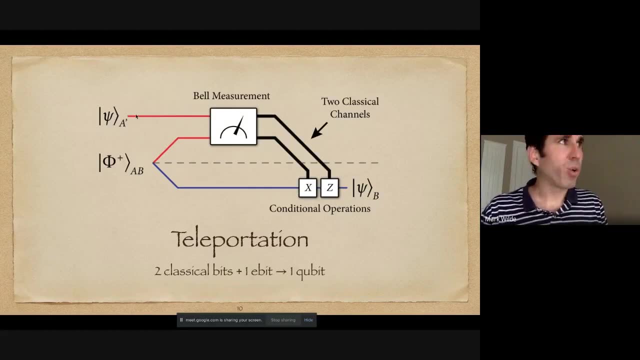 we're taking what Alice is doing and putting it in Bob's laboratory, and so that's teleportation. and the goal of teleportation is to communicate a cute bit over a large distance. it could be a short distance also, but the goal is to communicate it using entanglement and classical communication. okay, so the way. 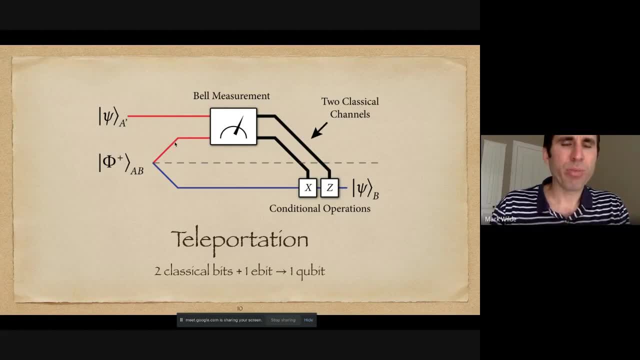 it works is, you know, we assume that Alice and Bob share this ebit beforehand and Alice is trying to send a cubit and then in her laboratory Alice performs this Bell measurements. okay, and I guess in the previous slide I didn't describe what that is, but we talked about how, using 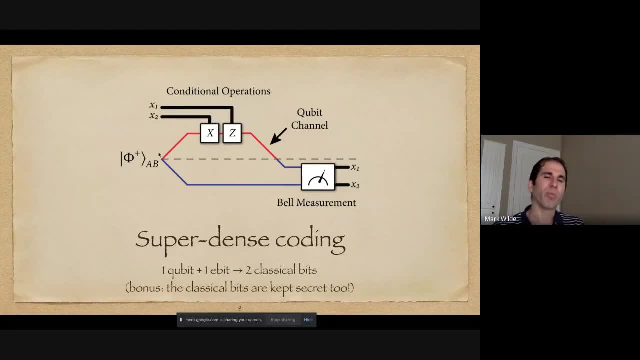 these local operations. Alice can rotate the global states of one of four orthogonal states, and that there you have four orthogonal states in a two cubit Hilbert space, and so those four states can realize a projected measurement, and that's what the Bell measurement is. okay, so the 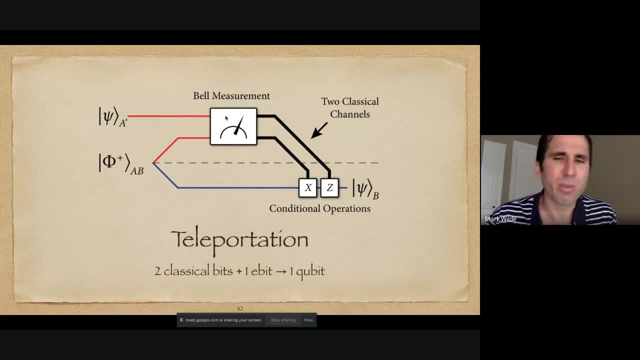 teleportation protocol begins by Alice performing this Bell measurement and then from that measurement she gets two classical bits. she communicates those over classical bit channels and Alice does, Bob does these local rotations. at the end Bob's cubit is reconstructed over here. this is probably the most. 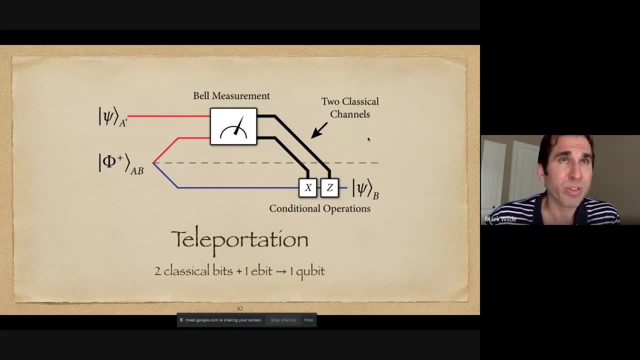 fundamental protocol in all of quantum information and you know this is the basic form of it and there's all kinds of variants of it and you can see that the variants of it there's. there's variants that are used for quantum error correction in fault tolerant quantum computation. there are variants used in 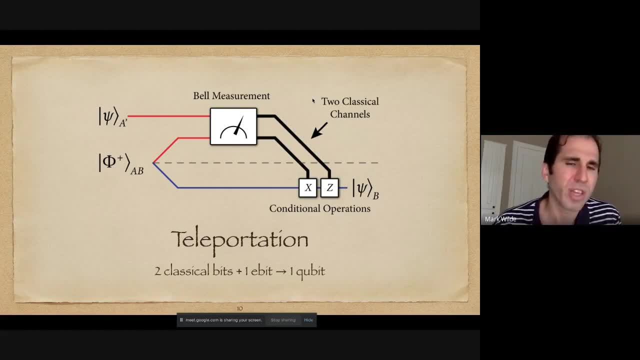 quantum key distribution to guarantee security of communication. there are, it appears, all there are multi-party variants. I've worked with a student here at LSU on a topic called bi-directional teleportation and then the first thing that you can do is you can start asking questions like: well, what? 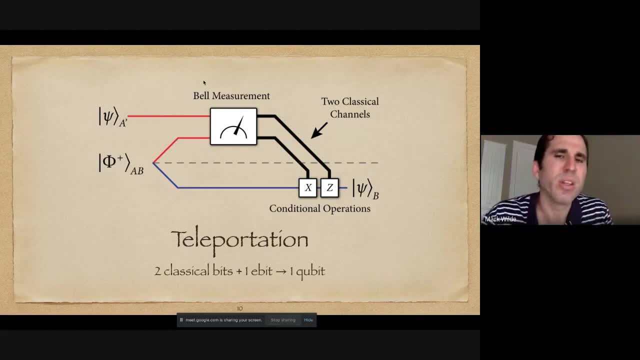 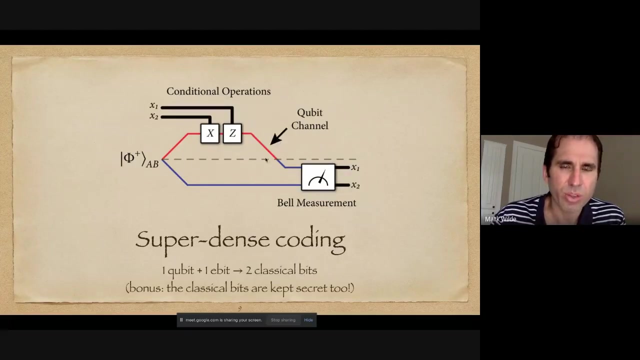 if the entangled resource state is not a perfect bell state, what can you do? you know? so there's been a fair amount of work on that topic and that's that's one of the questions of quantum Shannon theory, right? so in these basic protocols we can look at each of the resources, the bell state, the classical channels or in 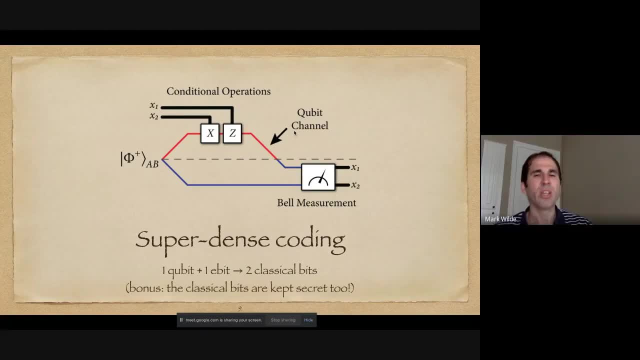 noisy cubit channel, sorry, the noiseless cubit channel. and then we can ask the question: what if we replace the noiseless resource with an unideal noisy one? what then can we do? and then that's where you can start thinking like claude shannon. did you know this is the claude shannon day, so we 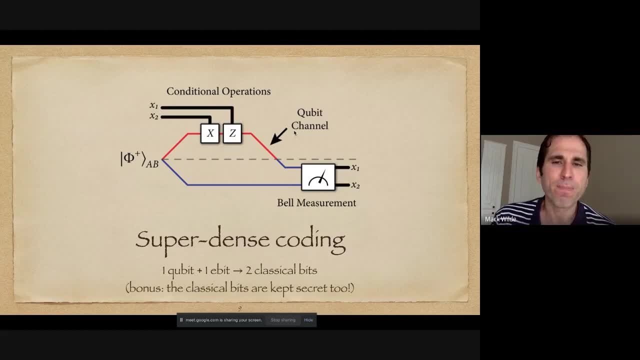 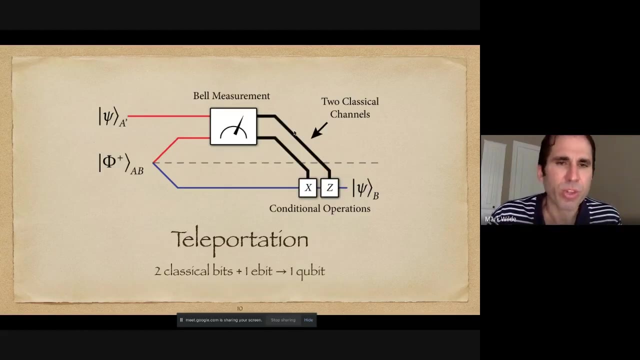 should think like claude shannon did and um and try to figure out like rates of communication, uh subject to uh, communication with a certain error probability. okay, so you know these are basic protocols and then they lead to all kinds of other things, and so they're very interested. 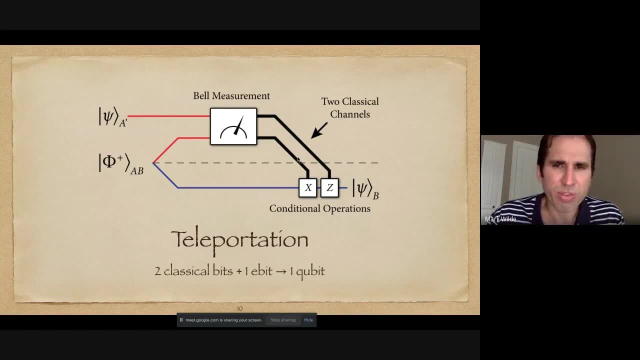 and fascinated. i want to make a remark, like i did in the previous slide, that there's also a security aspect with teleportation. um, if, if there's an eavesdropper tapping the line here and, you know, trying to use these classical bits to figure out something about the cubit being. 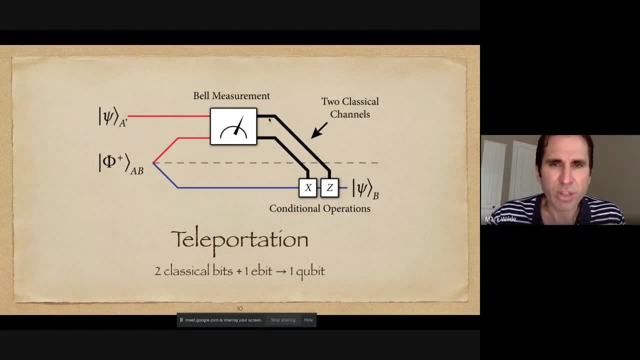 communicated. it's impossible these classical bits- they are uniformly random and independent of the cubit state- being communicated. okay and um. so there's a security aspect that's also important for the operation of the protocol, because if, if the classical bits did have something to do with the cubit state, 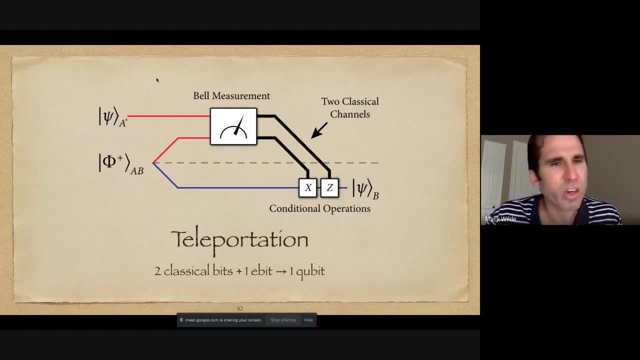 being transmitted, then inevitably you would be learning something about the state via a measurement, and in quantum mechanics there's this ubiquitous measurement disturbance principle, and so if these bits had something to do with the input state, you would be learning about it and disturbing it, and then you would not be able to reconstruct it over here. so that's that's an important point. 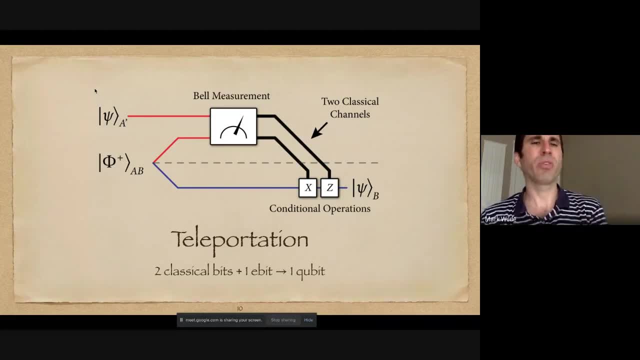 another important point is that, uh, there's a, there's a famous principle in quantum information called the no cloning theorem. so the no cloning theorem says that an arbitrary cubit state psi cannot be copied. and then when you look at teleportation you might wonder: oh, like the state's. 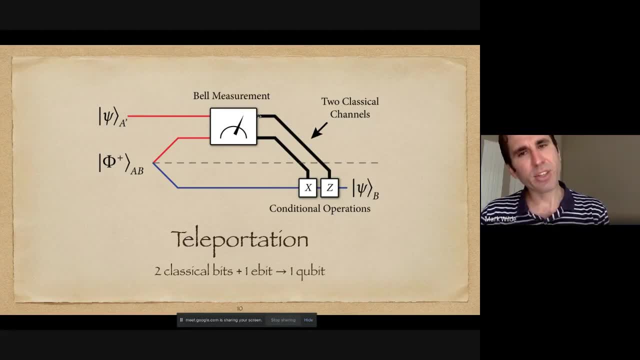 here and they get. it gets copied over here and there's a sense in which that's true, but there's only one copy produced. it's like the state here is destroyed and uh, it's, it's no longer available here and it's produced over here. 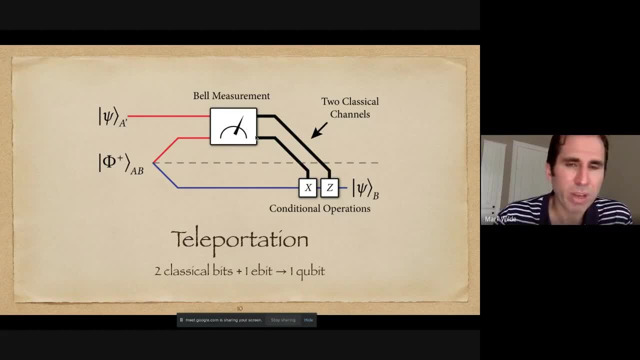 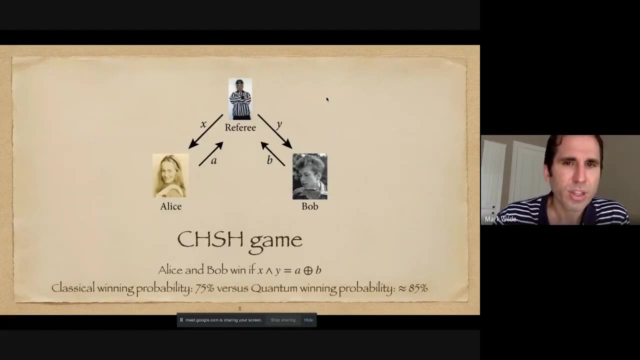 And so what's going on is that, through the interaction of the Bell measurements, the entanglements and the classical bits, you have this property where the psi qubit state is reconstructed over here. OK, So now I want to talk about the CHSH game. 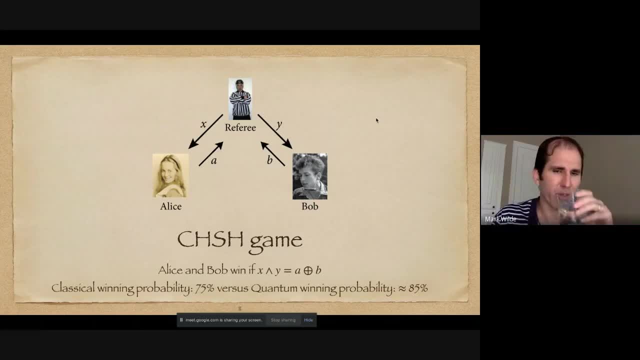 This is another basic scenario involving entanglement, And this is a variant of what Bell himself proposed in- I believe the year was 1964.. The game works like this: There's a referee and there's two players, Alice and Bob. 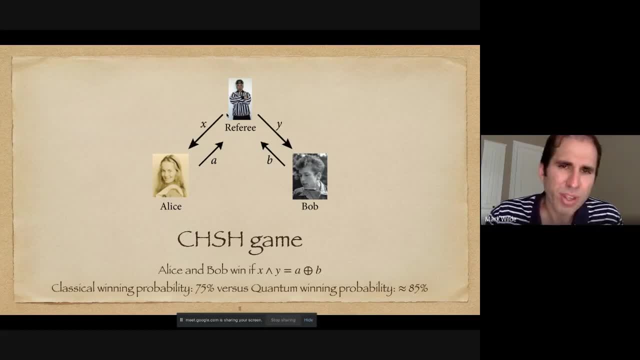 And we assume that they're in distant laboratories. The referee picks bits x and y uniformly at random. OK, Sends x to Alice, y to Bob And then Alice is alone. Alice is allowed to do something locally and sends a bit a back. 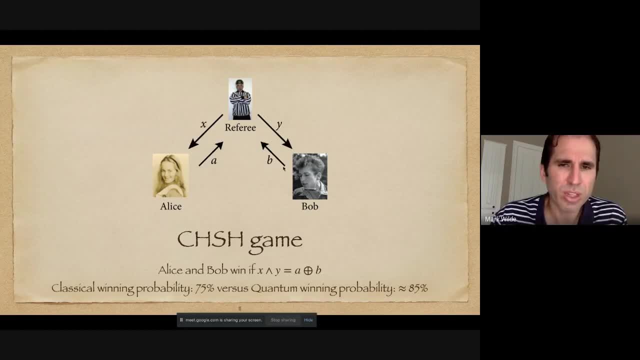 to the referee. Bob is also allowed to do something locally. sends a bit b back to the referee, They win the game. The winning condition is that. well, they win if the logical and of the x and y bits is equal to the exclusive or of the a and b bits. OK, 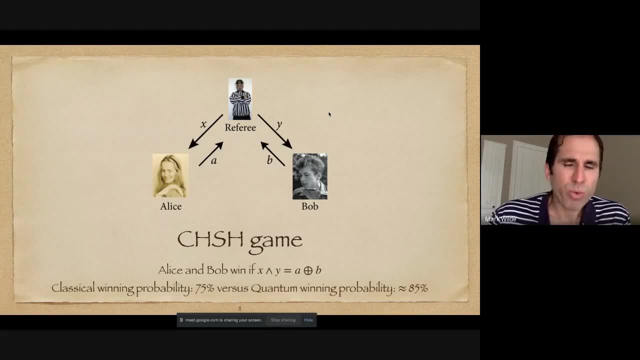 And there are different ways to play the game. One way to play the game is without any resource at all, right, without any quantum entanglement, without any shared randomness or anything like that, And if they do that, their probability of winning 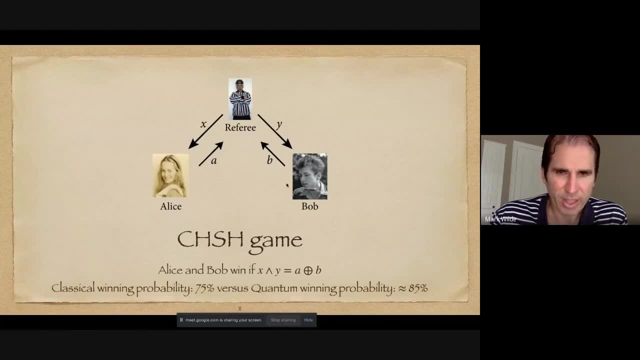 is no larger than 75%. OK, And there's a simple way to prove that I won't get into it. If you look at my textbook that I'm going to use, I'm going to say: you know, it was mentioned at the beginning of the talk. 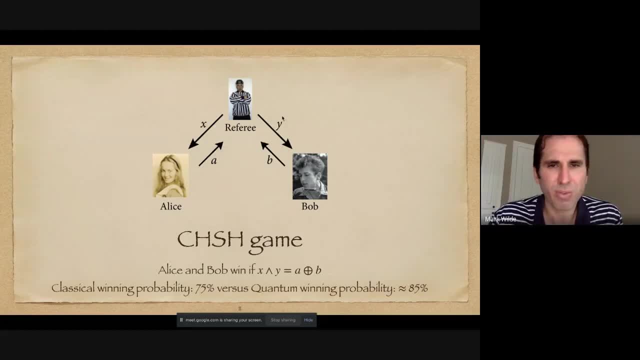 There's a section that talks about this, And actually this figure is taken from that part of the textbook. Another way to play the game is with shared randomness. So what do I mean by that? Shared randomness is like two coins that are correlated. 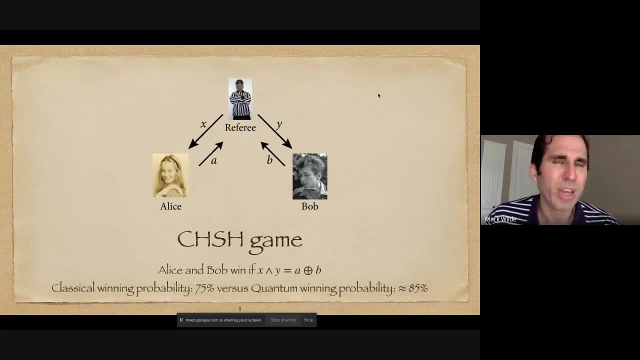 Like, either they're both heads with probability 1 half, or both tails with probability 1 half, So that's another way to play the game. That is a. That can be called a. That can be called a convex combination of classical strategies. 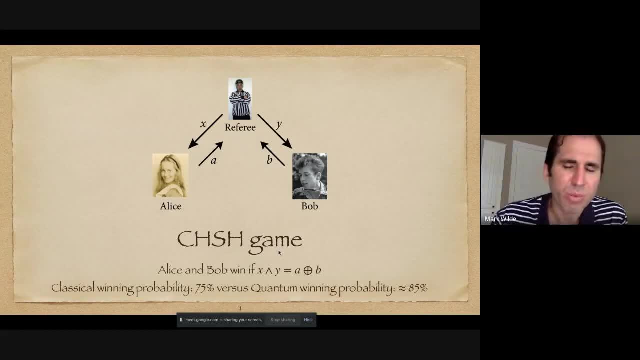 And, due to the structure of the game, it's possible to conclude that randomness does not help in winning the game. Still, the best that they can do is 75%, And I should mention that they can achieve this 75% if they always just report back 0.. 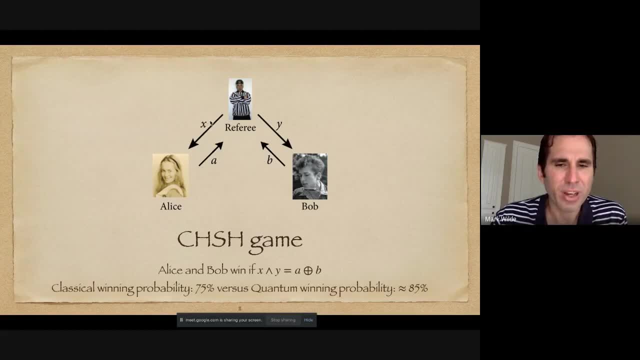 Why is that? You know, If the bits x and y are being chosen uniformly, at random, you'll get 0, 0 with probability 1- fourth, 0, 1 with probability 1- fourth, et cetera, And three of the possibilities. this left-hand side. 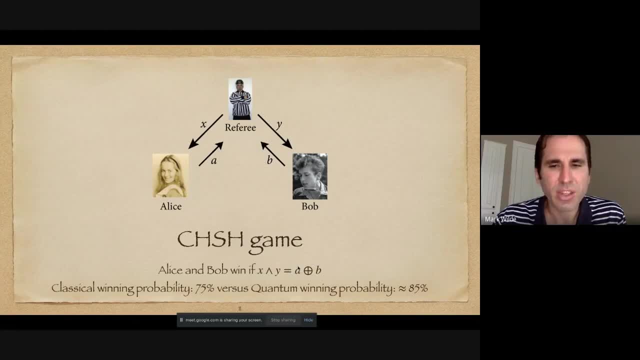 of the winning condition will be 0. And if they always report back 0, then the exclusive order of 0 is 0. And so they would win, Yeah, 3 fourths of the time and lose 1 fourth of the time. 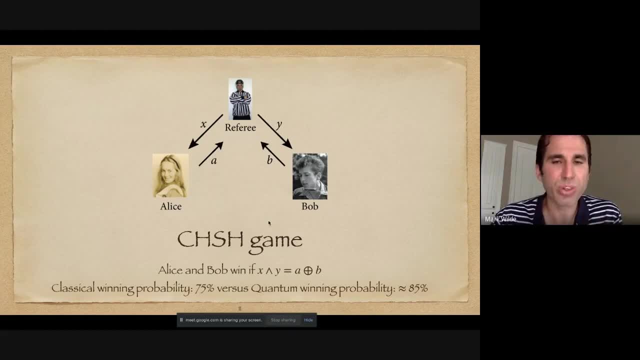 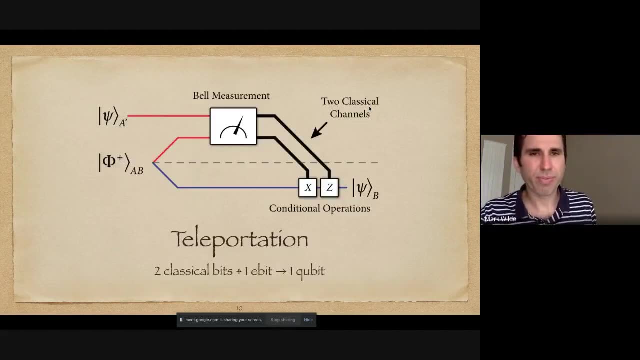 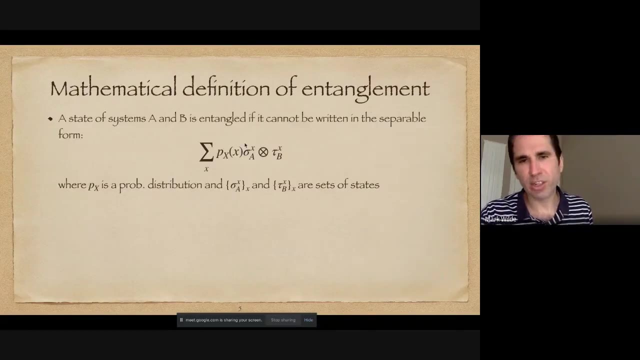 So that's how they. That's a strategy they can use to win 3 fourths of the time. OK, Another possible strategy would be to use a separable state. So that was what we talked about here. You know they could share a separable state and use. 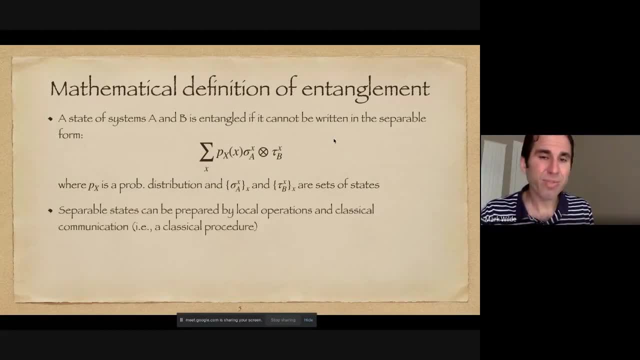 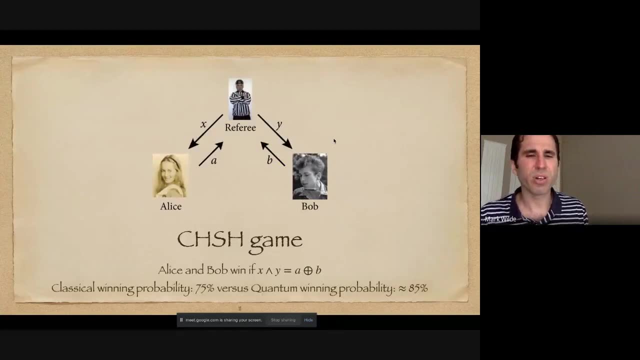 They could be allowed to share the state before the game begins And what's possible to do? It's a show- And I believe this was first argued by Reinhard Werner in 1989- that if the state's separable, then they cannot win. 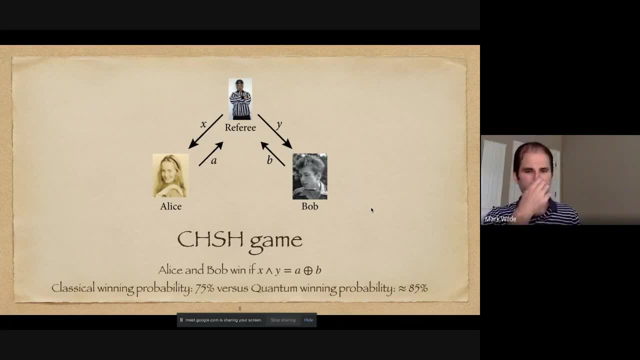 They're still limited by the 75%. OK, But what's also known is that another strategy they can employ is using the Bell state. OK, So using the Bell state and then depending on which bit Alice gets, which value of the bit Alice gets. 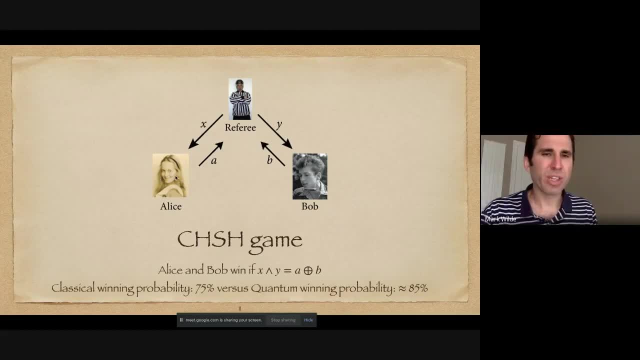 she'll either perform a sigma x or a sigma z measurement And then, Bob, depending on the value of the bit that he gets, he'll either perform sigma x plus sigma z or sigma x minus sigma z, up to a normalization to make it an observable. 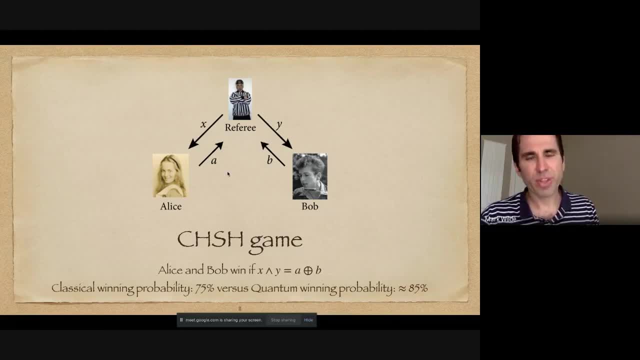 So using that strategy, OK, OK, They can win 85% of the time, OK, I believe. the exact number is cosine squared pi over 8. And so that's a large separation between what is possible with quantum mechanics and what is possible with classical mechanics. 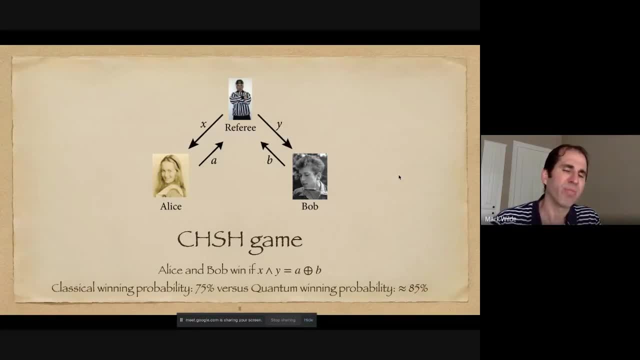 And one can say that this was one of the first examples of a quantum information protocol. OK, And one can say that this was one of the first examples of a quantum information protocol in which a quantum advantage over a classical strategy was predicted. Yeah, 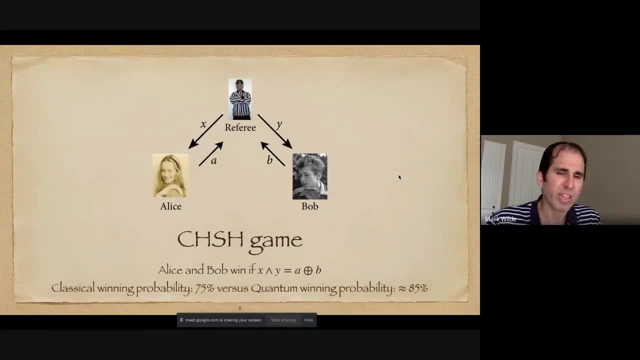 So this is very famous CHSH game is the same as what's called a Bell inequality. This game has been experimentally tested many times now And in 2015, there was a real breakthrough, experimentally. OK. OK, Various experimental groups started. 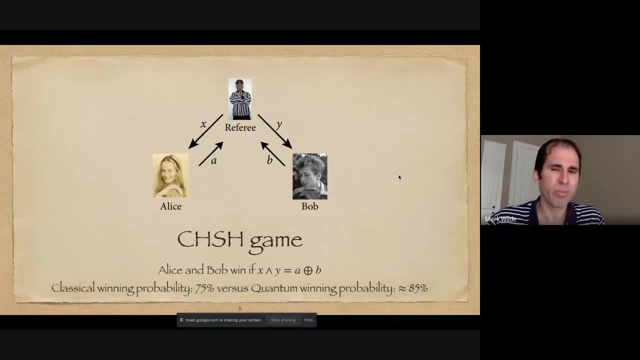 reporting the ability to perform a loophole-free Bell test. What does that mean? If you're doing an experiment and trying to implement this protocol experimentally? there are two and even three major loopholes that need to be considered. The first is what's called the locality loophole. 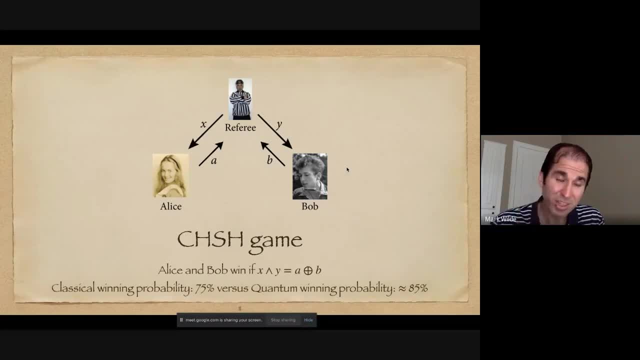 Alice and Bob have to be far enough apart, such that they're going to be able to perform a loophole-free Bell test. They do not have to be in separate rooms, They have to be in separate labs. They're going to be able to perform a loophole-free Bell test. 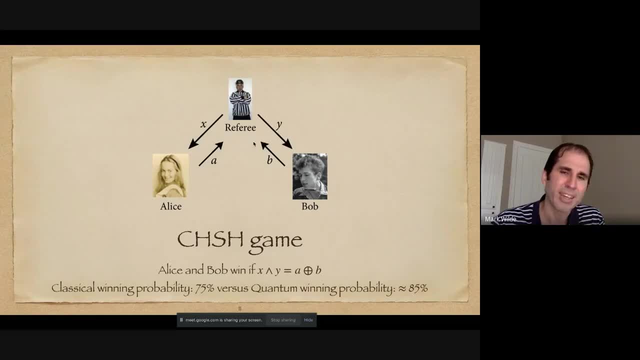 That's basically the first step. So Alice and Bob have to be far enough apart, or say 10 to 2 weeks apart, so they can perform a loophole-free Bell test. Then the second step that Alice and Bob need to do is replace. 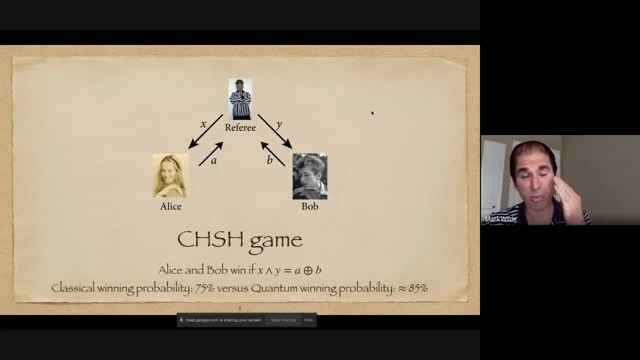 order them with a loophole-free Bell test, And the first step is, as such, to keep Alice from having to get herself into a loophole or maybe another loophole. And if they get themselves in a loophole, they have to. yeah, they have to be in separate rooms. 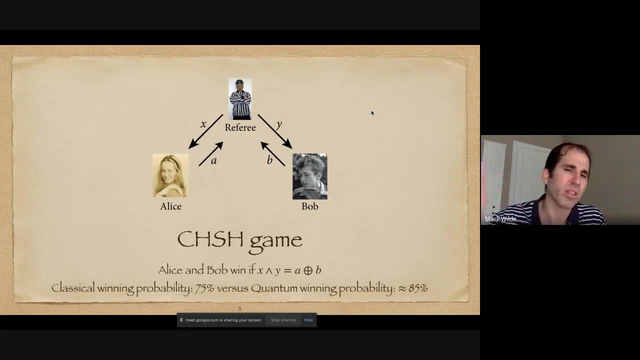 or separate laboratories, OK, And far enough apart, such that, you know, the speed of light comes into play as a limit. So that has to be closed And the detection loophole, that's another loophole, is called the detection loophole. So typically this kind of experiment is conducted in quantum optics. 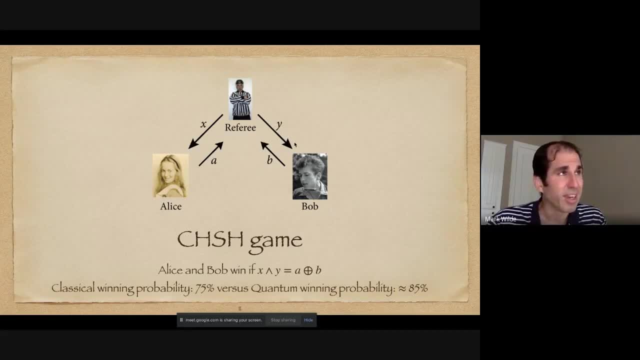 And so they're using photodetectors And they have to be efficient enough, such that, like there's a sufficiently large number of rounds where they're reporting back something and not, you know, claiming too much that there's a misdetection, you know that there were no clicks with the photodetectors. 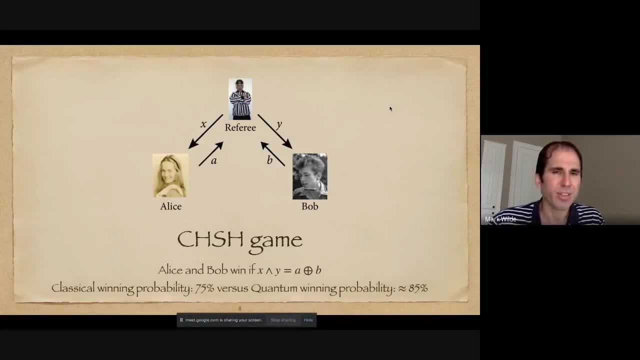 Because otherwise they could be like faking the. you know there's an argument they could be faking, They could be faking the data that's coming back. So those are the two major loopholes And a remarkable, various remarkable experiments were conducted to close both of these loopholes. 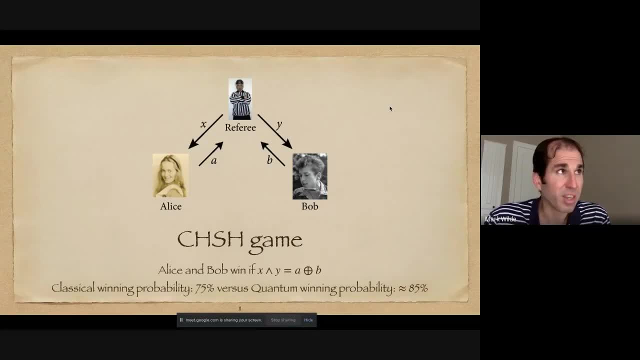 One of which was in Delft, Netherlands, And another was in Boulder, Colorado, I believe. Okay, And there was a third one as well, Okay. Okay, By the way, If there are any questions for me, I don't have a problem if someone wants to interrupt. 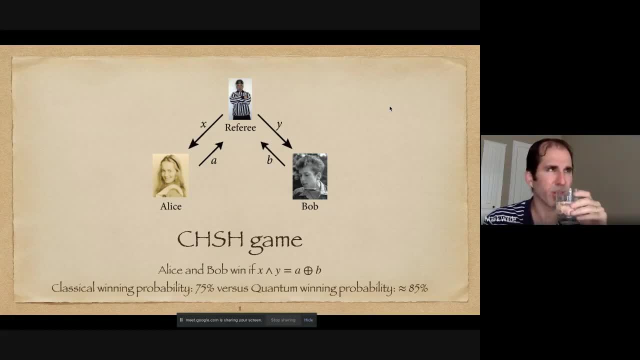 I don't know if I don't know what the structure is of the talk, But it's also fine if people want to wait until the end. We usually have questions to answer. then You're going to, we're going to do the questions at the end. 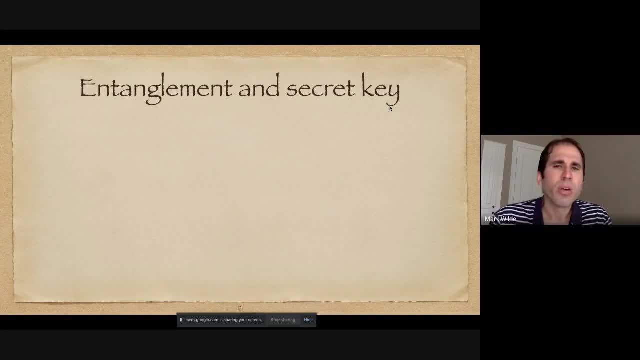 Yes, Okay, All right, Good, All right. So I want to talk more about the connection between entanglement and secret key, And then we're eventually going to get to the Shannon. We're going to get to the Shannon, Okay. 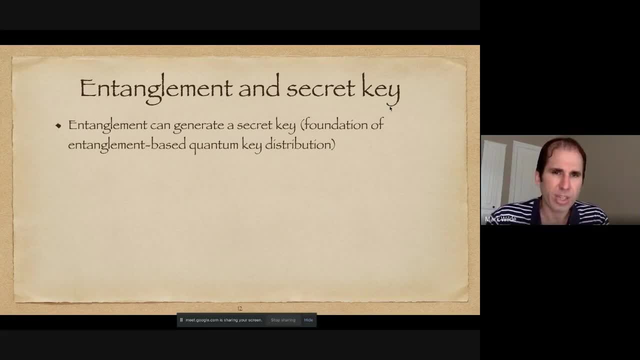 So entanglement can generate a secret key, And we discussed this earlier. I'm going to mention it again. So, and and this fact is the foundation of the whole research topic called entanglement based quantum key distribution, So if Alice and Bob shared this maximally entangled state or this EBIT near the Belvedere, 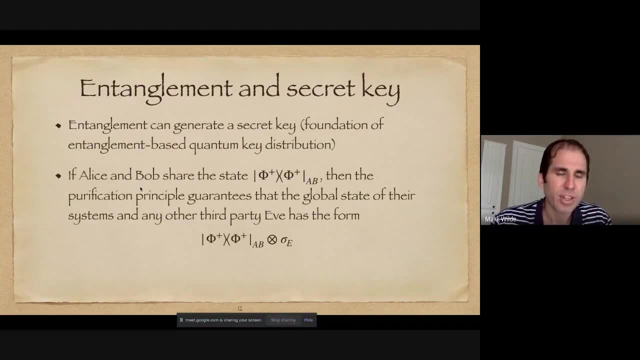 Bell state, whatever you want to call it. Then in quantum mechanics there's something called the purification principle. So it guarantees that the global state of their systems and any other third party, like the only possible extension of the state to a larger Hilbert space, such that 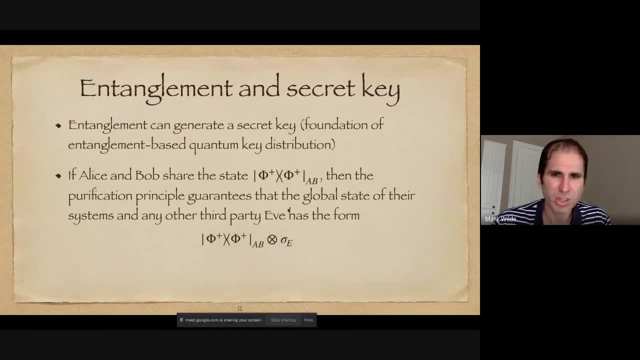 when you discard a system in the larger Hilbert space, you end up back with the same state. The only possibility is a state of this form where Eve, the state of the eavesdropper, a density operator, sigma E, is in tensor product with five plus. Okay, So you know, then they can. 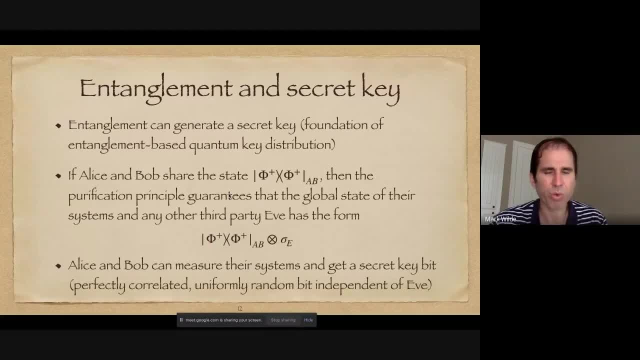 perform local measurements on their systems. They can perform sigma Z measurements, And so what will happen is that if they perform this measurement, Alice will get zero, Bob will get zero, with probability one half, And then they can perform sigma Z measurements. And so what will happen is: 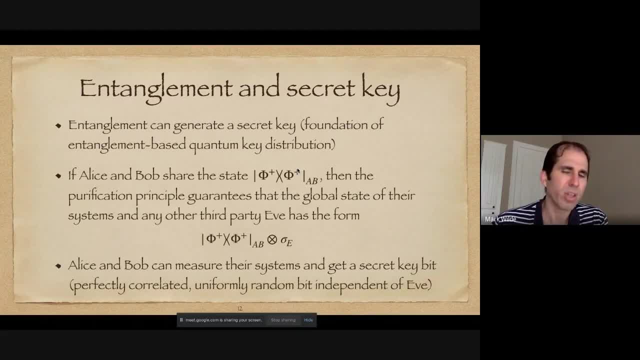 that if they perform this measurement, Alice will get zero, Bob will get zero with probability one half. The other possibility is that Alice will get one, Bob will get one, with probability one half. Okay, And those measurement outcomes will be independent of what Eve can observe. 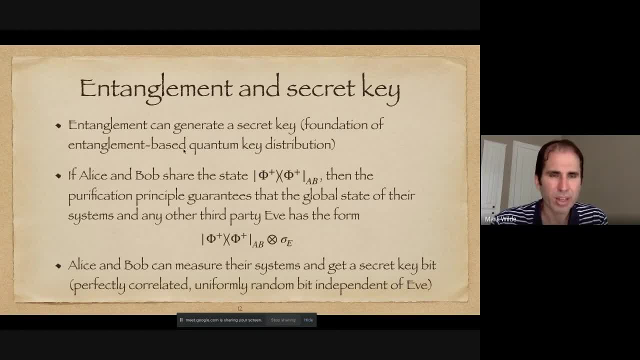 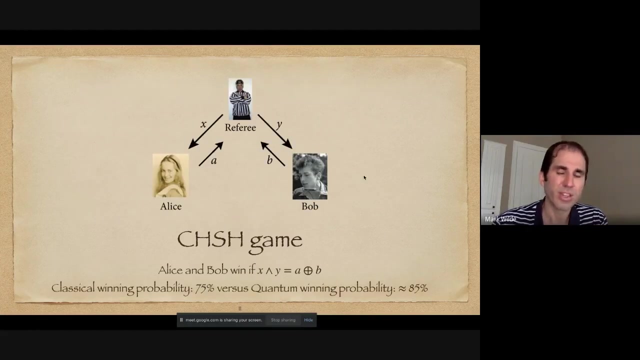 Okay, So the goal of an entanglement based quantum key distribution protocol is to produce a state of this form. Okay, And suppose that you're not sure whether you're making a state of this form, How do you test? for it Turns out that you can use the CHSH game, So you would have. 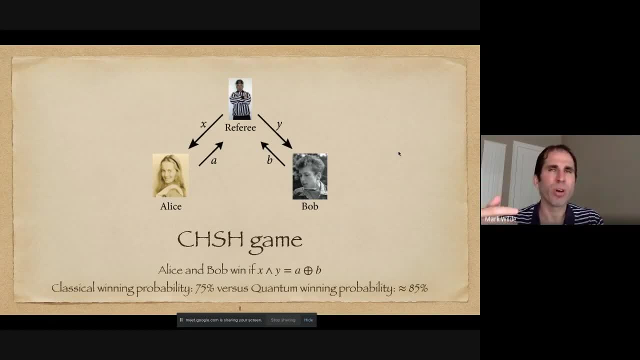 many independent rounds of the protocol where you're using a quantum channel that connects Alice to Bob. That could be like a fiber optic cable or a free space link. So you're using this channel and you're trying to make the bell state with each use of the channel So you can conduct. 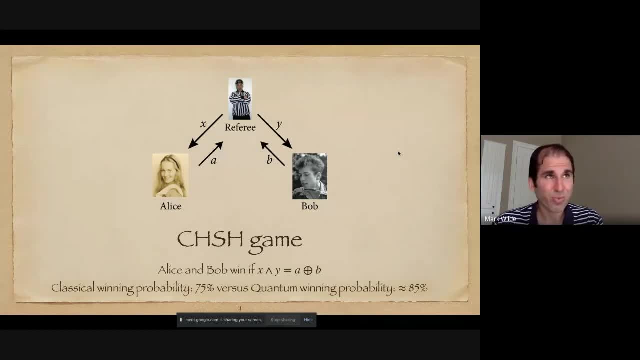 a protocol and on a random fraction of the rounds of the protocol, you can test whether they can win the CHSH game Right, And then if you're finding that they're winning approximately 85% of the time, then you can conclude that via this process they can generate maximum entangled states. 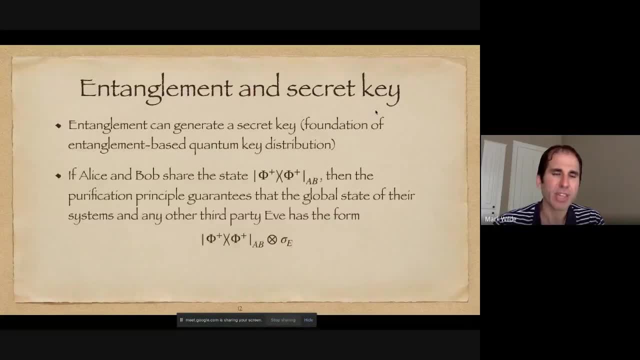 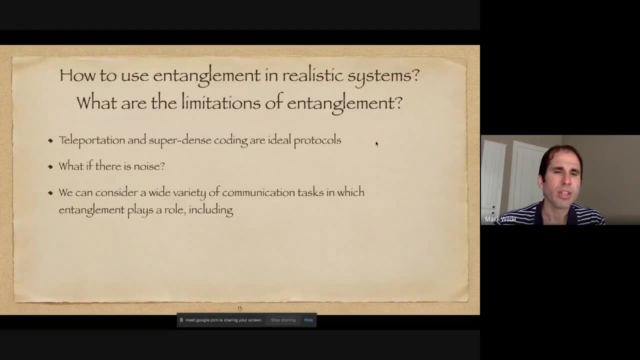 Okay, That's the basic idea of entanglement based QKD- quantum key distribution. Okay, Now let's get to the Shannon theory part of the talk, since we talked about the basics. So we talked about teleportation, superdense coding as ideal protocols, We mentioned how there could be noise like the: 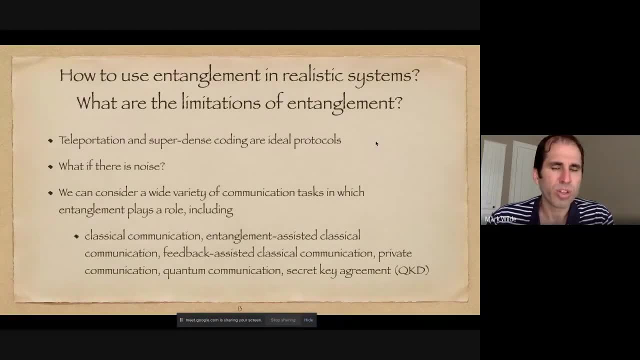 entangled resource state could be noise. We talked about the entangled resource state could be noise. We talked about the entangled resource state could be noise. We talked about the entangled resource state could be noisy, or the channel itself, the qubit channel and superdense coding can. 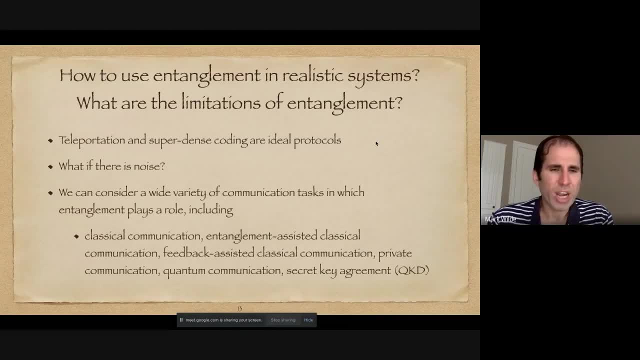 become noisy. And then there's a wide variety of communication tests we can consider in quantum Shannon theory, And so that's what these textbooks are about. you know to to analyze these in a lot of detail, Right, And so today I'm just going to give you an overview of these different protocols. 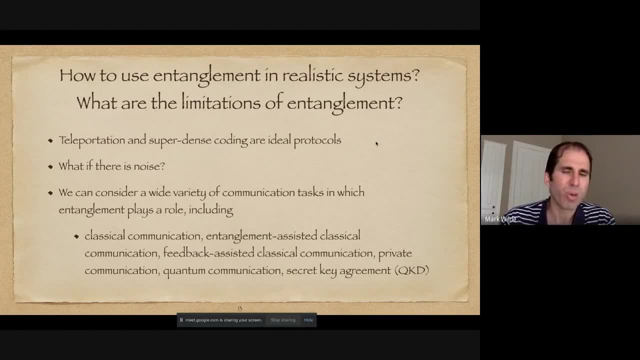 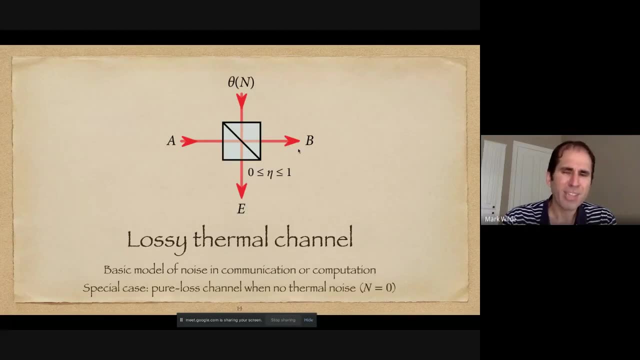 So you can have a sense of the landscape and the kinds of problems that are, that are open, that people are thinking about. Okay, A basic example of a noisy quantum channel that's relevant for experimental practice is what's called the lossy thermal channel And this: 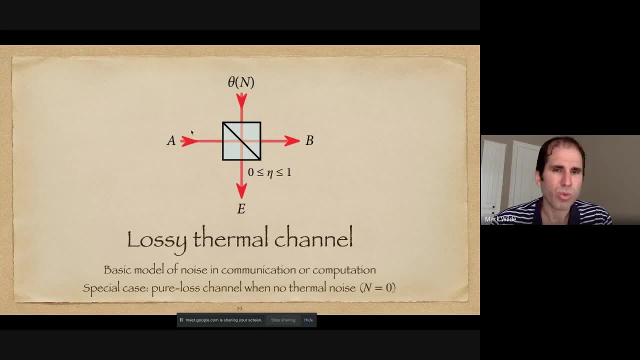 is the model of it. So we imagine that Alice has what's called a mode of light. If you've studied quantum optics, you'll know what a mode is And you can see that Alice has a mode of light. And if you don't know what that is, just think of this as a qubit, Okay. And or you can think of it as: 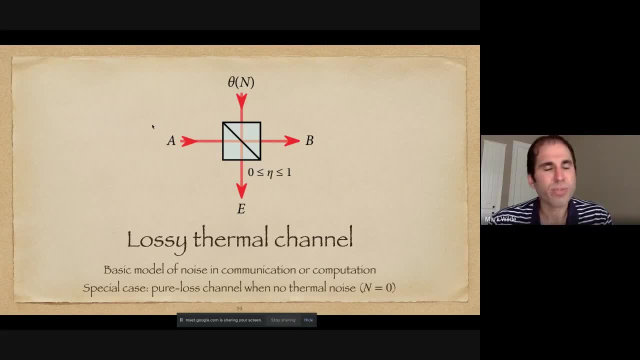 like a. a, a photon that's either in the vacuum or single photon stater could be super positions or mixtures of those. Okay, So Alice sends her mode into a beam splitter And the environment that's inaccessible injects a thermal state. 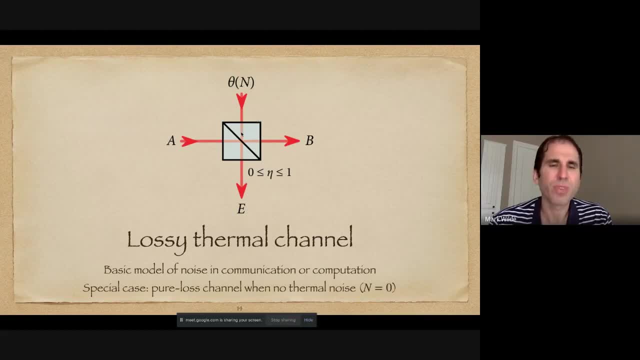 with mean photon number big N to the channel. okay, And so these two modes get mixed at a beam splitter and this is the output for Bob, and there's a fraction eta of the input that goes through and the other fraction goes to the environment and is lost, okay. 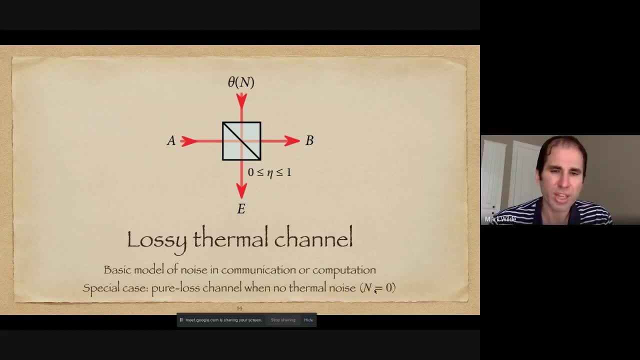 A simple example of this is what's called a pure loss channel, That's when there's just a vacuum state of the environment. but, as you know, in quantum mechanics the vacuum is, it's like, supposed to model nothing, but nothing is always something. 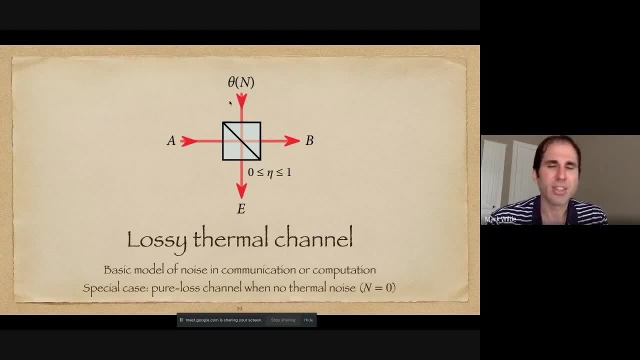 There's always this zero point energy, and so you need a fully quantum description of this to be accurate. So, with the pure loss channel, eta is the fraction of the mean photon number that makes it from the input to the output. okay, So this is a basic communication model. 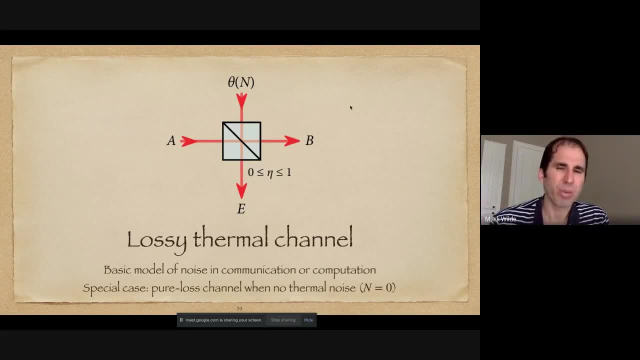 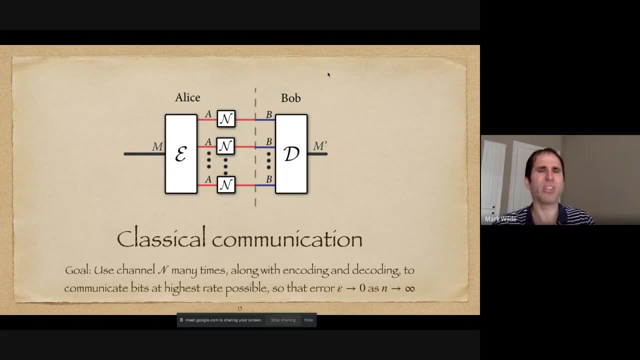 that you can have in mind while we're talking about, while we're talking about things for the rest of the talk. Okay, what is a basic communication task? simply to communicate classical messages, And this is a diagram you can have in mind for this task. 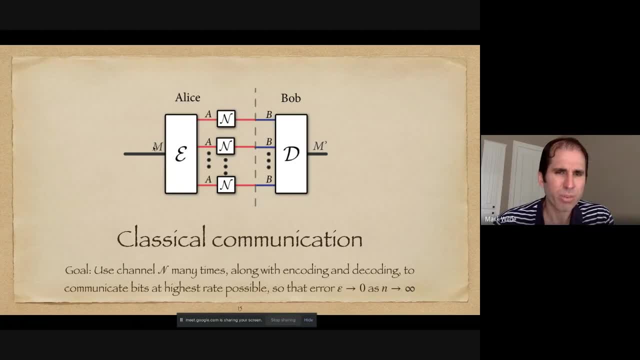 So Alice picks a message m from a message set, encodes that into a quantum state of these channel input systems and there can be a little n of these little n's for the little n channel uses okay. So big N is noisy channel. 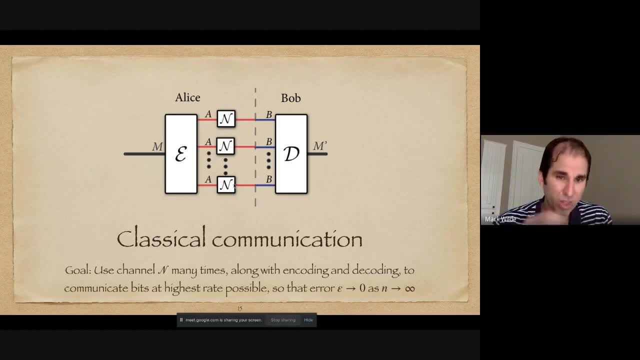 that's what we'll use for the noisy channel, and then little n will be the number of channel uses. So while doing this, encoding, Alice could encode the classical message into a very complicated multi-part type entangled state. in principle, that would be one option. 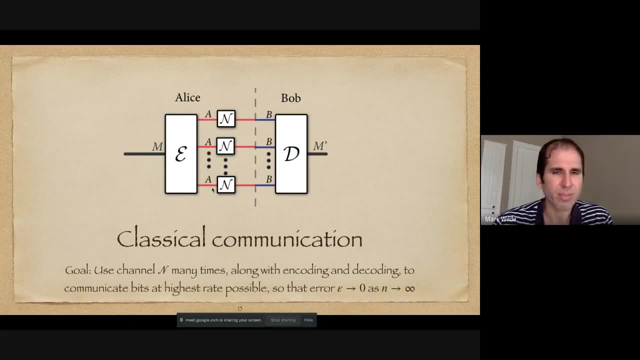 Another option would be to encode in a tensor product state. That would not use entanglement, And so there are questions here. given a noisy channel, what is the best method of doing an encoding? Does it suffice to use a product state or is it better to use an entangled state? 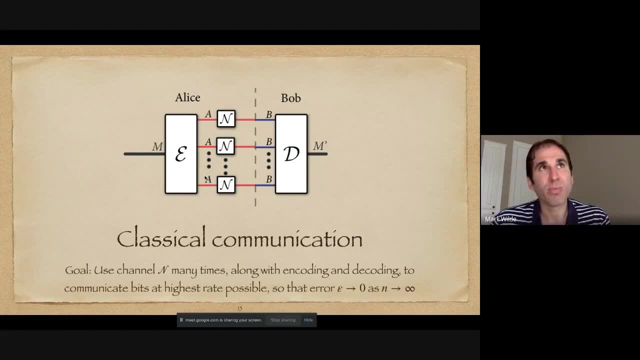 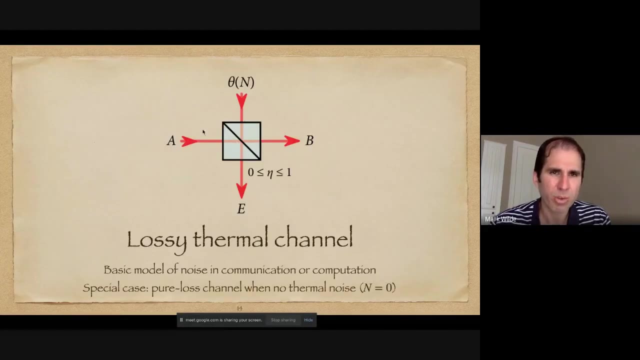 So that's a basic question and we only know so much about this question. actually, We don't know as much as we probably should. So the last question is a very sweet question. So these systems go through the channel and, like we said in the previous slide, 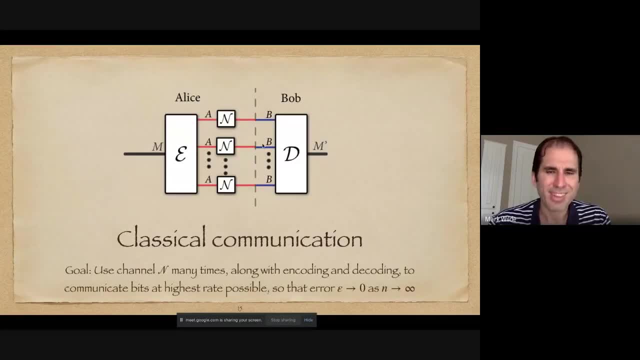 each of these channels could be like a thermal channel, and so something ends up in Bob's laboratory, these little n Bob systems, and then Bob can do what's called a collective measurement on all of these qubits or modes that end up in his laboratory. 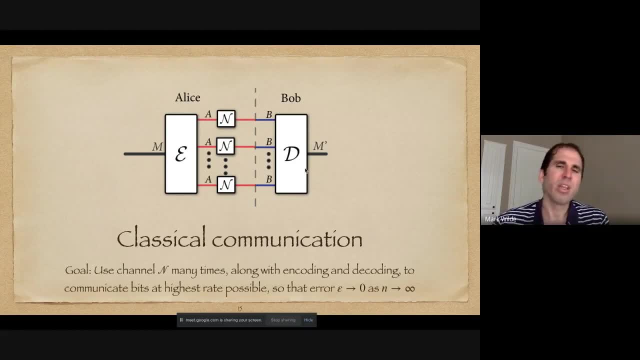 So what is meant by a collective measurement would be: Bob performs a general quantum computation, the general unitary, and then does measurements on each of the cubits to try to figure out the message M that was transmitted, and M prime will be his estimate of the message that was. 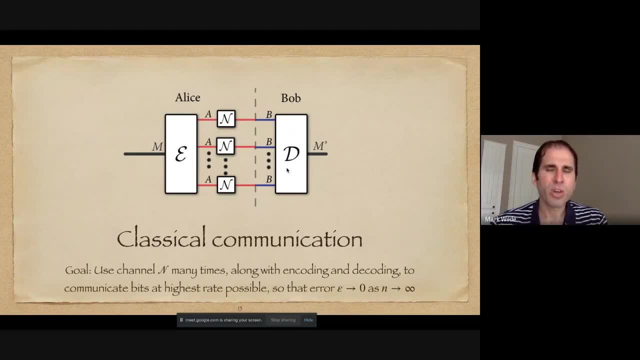 transmitted. okay, so in the decoding- a collective measurement, we said it can be realized by a general quantum computation and that would be a general unitary. if the unitary acts globally on all of these cubits, then if it's used in a different context it might have the ability to generate entanglement from a. 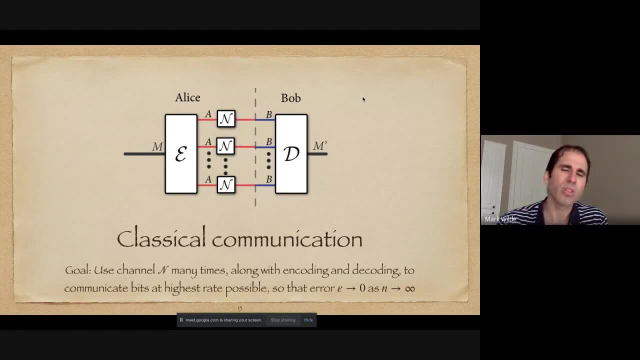 from a product state. okay, so some fun. sometimes people call this entangled measurement. I always use the term collective measurement because it acts collectively in all these modes or cubits. so we see that both in the encoding process and in the decoding process entanglement plays a role. it's there, you know, is where. 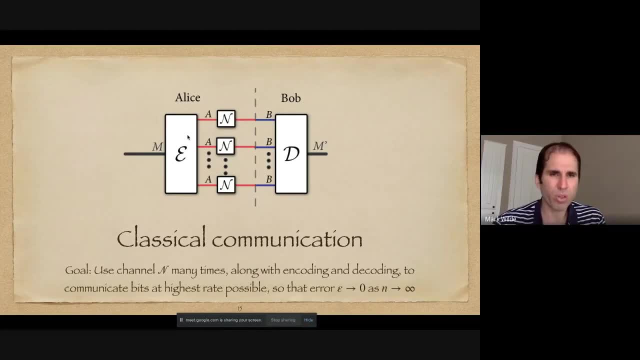 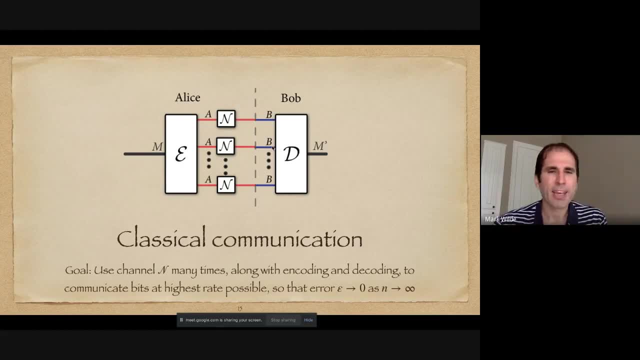 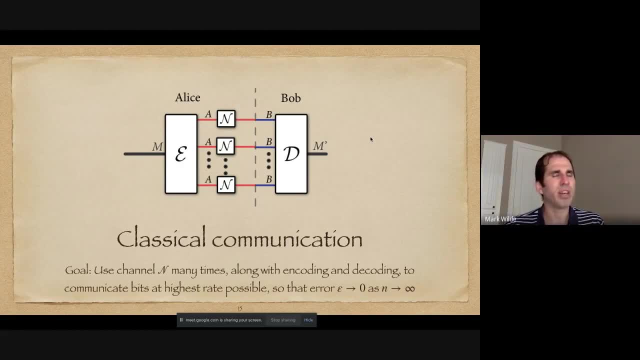 we want there to be a very small chance of an error. so in the shannon theory his idea was: let's focus on rate and let's coarse grain away these other two parameters. how to do that? let the number of channel uses little n become large and then demand that as the number of 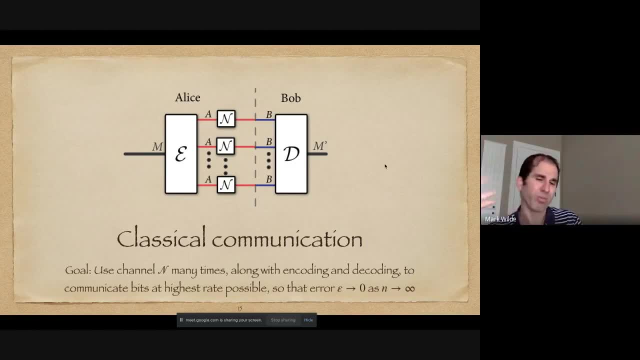 channel uses becomes large, the error tends to zero. okay, that was a very nice idea that coincides with what is of interest in practice. okay, an assumption that we're making, just like shannon did in his original work, is what's called the iid assumption: independent and 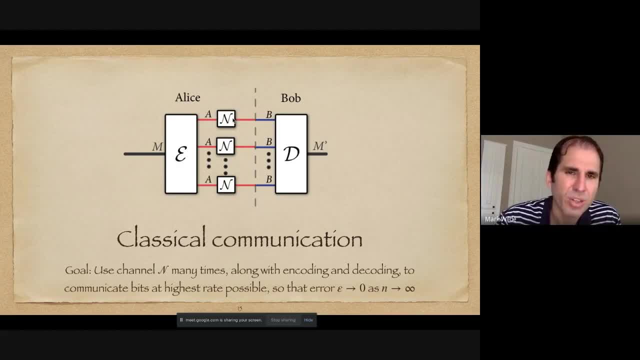 identically distributed, so each use of the channel is independent of the next one and the noise is modeled identically. okay, and so it's a reasonable approximation for many communication systems scenarios, but of course you can question that. okay, so how does entanglement play a role? we? 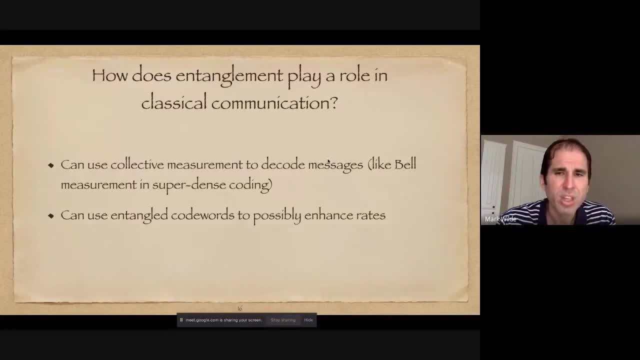 discussed this. you know you can use a collective measurement. what's an example of collective measurement? we saw it in the super dense coding protocol. bob performs a bell measurement, that that is implemented by a small quantum computation involving a controlled- not gate- and a hadamard, you know. so that's a collective measurement. 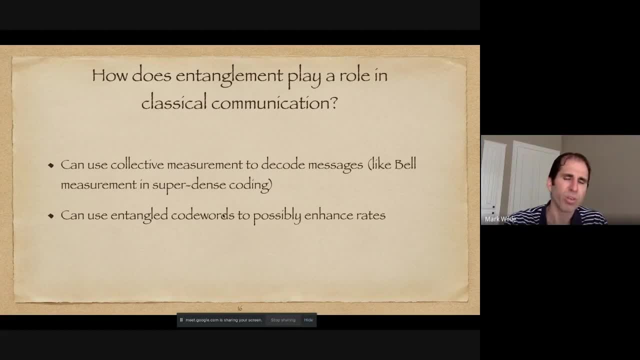 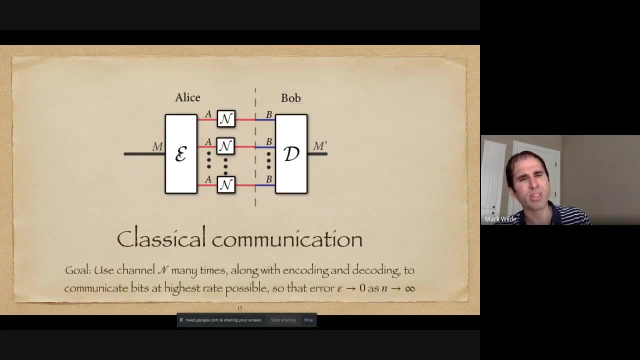 the other way. entanglement appears, we set it. the code words that alice is transmitting can be entangled. and um, both of these. why do we want to allow these collective strategies? well, we can achieve higher rates of communication. so if we limit ourselves to, um, you know, encoding information. 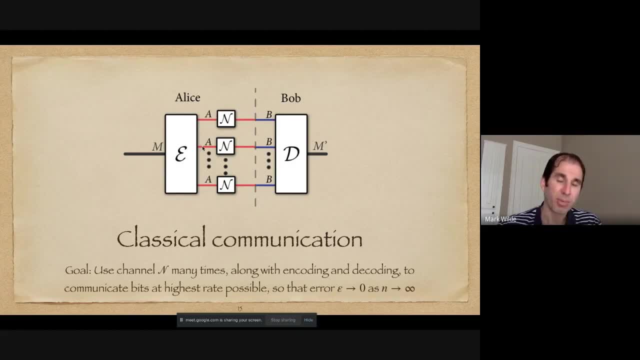 in product states. uh, that's, that's a limiting strategy, and that's that's what's done in the classical theory. and if we don't allow for collective measurements, that's a limited strategy as well, and what we instead allow for is all possible encodings and decodings allowed by the. 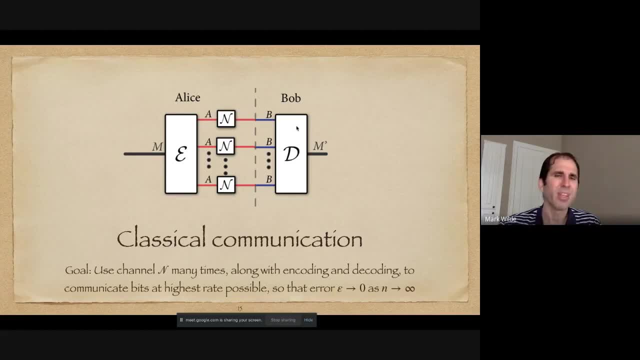 laws of quantum mechanics, and then that's how we define capacity. that's the natural way, given the physical setup. you know, we allow for all possible encodings and decodings. then we want to know what is the fundamental limit of communication. maybe it'll be hard to reach it, but at least we would know it as physicists, engineers, mathematicians. 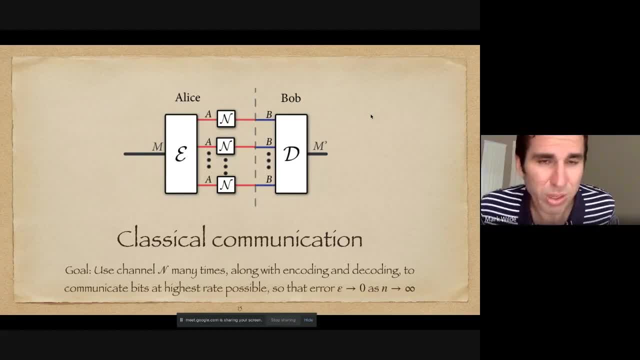 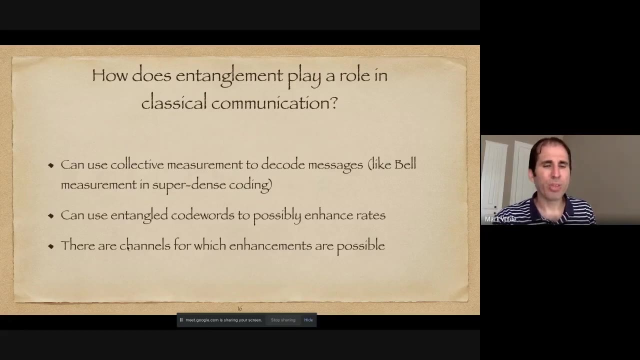 computer scientists. whatever you know, we would know the fundamental limit. so if your goal in life is to know, you know what are the fundamental limits of communication. this is a way to figure out an answer to that question and indeed we know that there are channels. uh, for which enhancements? 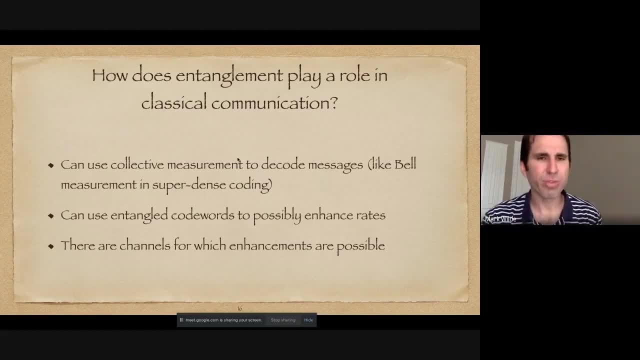 are possible. um, there are many channels we're aware of for which, uh, collective measurement gives a benefit to communication. um, regarding the entangled code words, it's something that we only know kind of in principle. there's- no, there's still no explicit example of a, of a channel for which we know that. 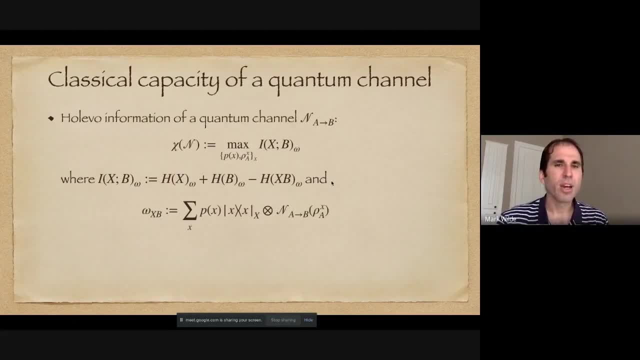 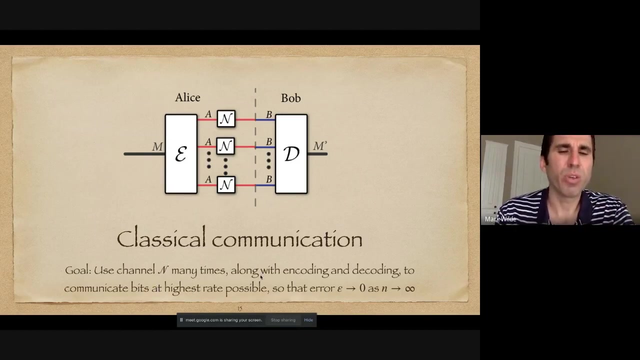 the entangled code words help, um, all right, so i want to get into a bit more math, since we gave a lot of discussion on the previous slide. how can we mathematically characterize the classical capacity? so i don't know if i said it, but the, the classical capacity, is the largest rate in which we can communicate error-free. 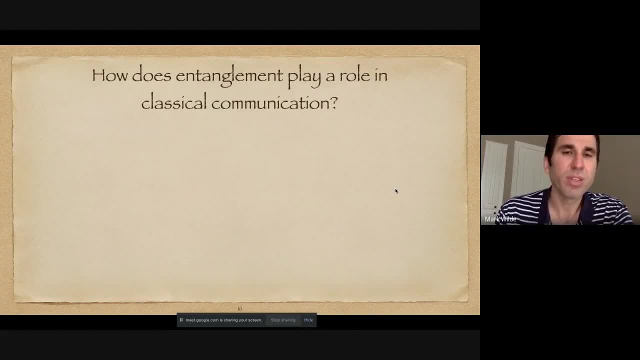 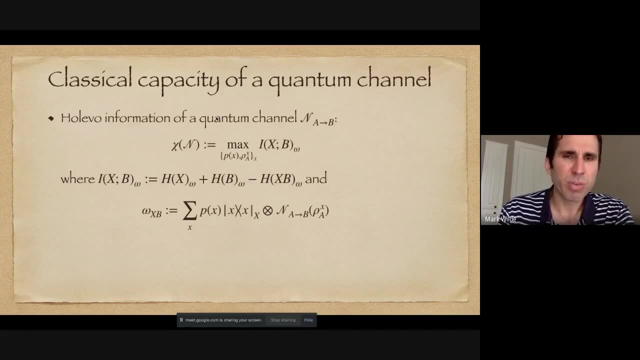 in the limit, as the number of channel uses goes to infinity. okay, and we can define a quantity that's called the whole value of information. this is a generalization of shannon's mutual information. so how do we define it? we define it like this: this quantity ixb is hallevo information, it's a, it's a quantum version. 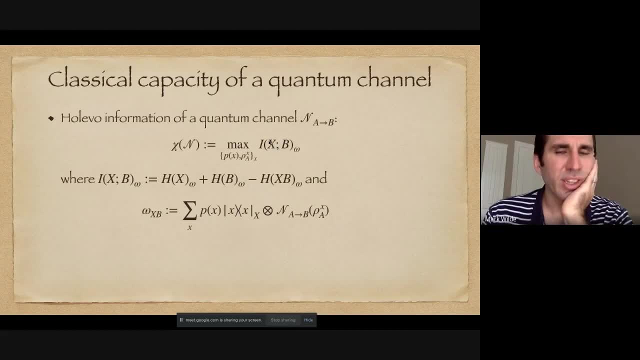 of mutual information in which this system x is classical and this system b is quantum. okay, it's defined as this linear combination of von neumann entropies. sorry, i don't have the formula for this for von leumann entropy, but um, you know it's, it's a well-known thing for a density operator: row. 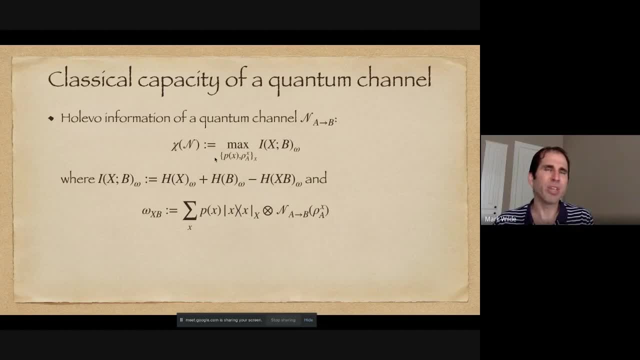 the von leumann entropy is minus trace. rho, log rho, where the log is the binary logarithm. okay, for when we, when we're thinking about shannon theory, we use the binary logarithm, so this notation means um. take the state omega that's has this form. this is a classical system. 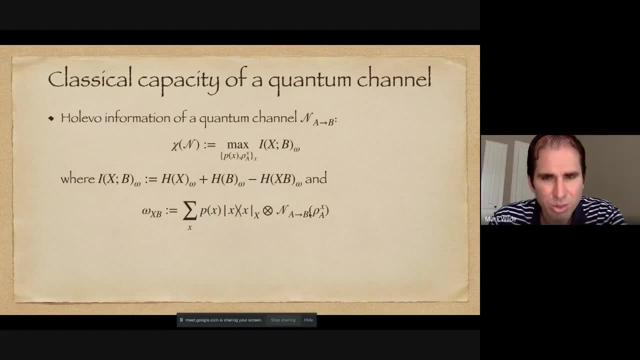 where these are orthonormal states. this is a probability distribution. these are general density operators that can be input to the channel, and then you get a quantum state on the classical system x and the quantum system b. to calculate this entropy, you trace over the quantum system b. 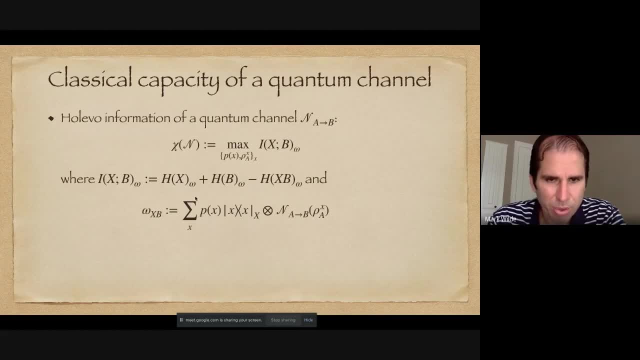 you get- uh, you know this density operator here. just pretend that's not there, and then you evaluate the von leumann entropy. in that case it'll just be the same as the shannon entropy of p of x. to evaluate this one, you trace over the x system and then you end up with the channel acting on the. 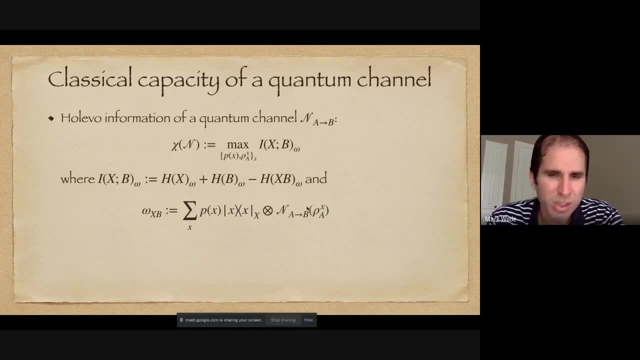 average density operator, the sum could come inside the channel because the action of the channel is linear and you would compute this entropy and then this is the joint entropy of the whole state. okay, this is a measure of classical correlations that can be generated using the channel mutual. 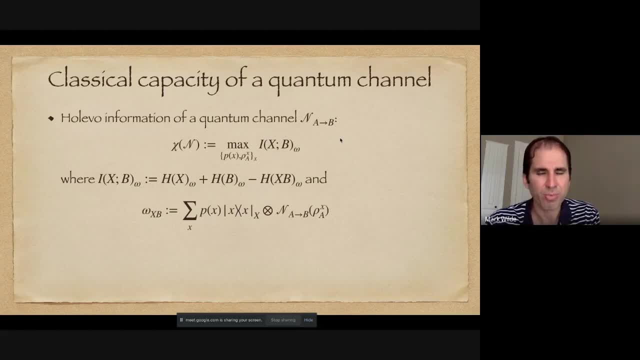 information is a measure of classical correlations. there's also a way to write it as relative entropy of the joint state to the product of the marginals, and so it's like a comparison between the actual state and a tensor product state, and so that's a measure of correlation, you know like how far away. 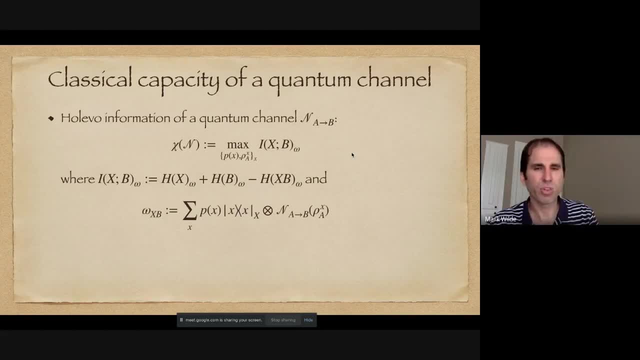 are you from a product state? so it's a measure of classical correlation. we have this formula for some channels. the classical capacity is equal to the whole label information. okay, but in general we need to do this limiting procedure to calculate the capacity, and this expression is called regularized label information. so you plug in. 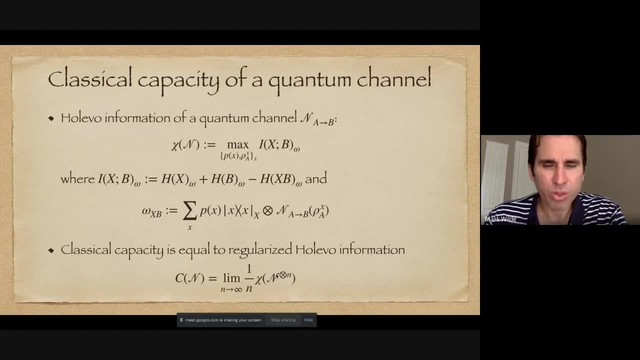 minute a little and then sort of sum in that little. if you plug in a hundred percent it'll add a point, it'll get five percent. if you place this failure ago, basically one, and that's a all subscriptions value which is zero because these are all сумmas, just one plus one plus one, plus all gain by one. 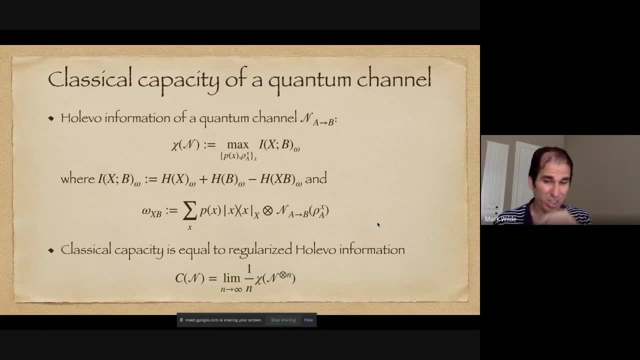 so if i would have one intrigued along with just one product, or if this is traveled sticker means one boils down to. we can't really delve deep into that today, But this regularized procedure. it's allowing for the possibility of using entangled code words in conjunction. 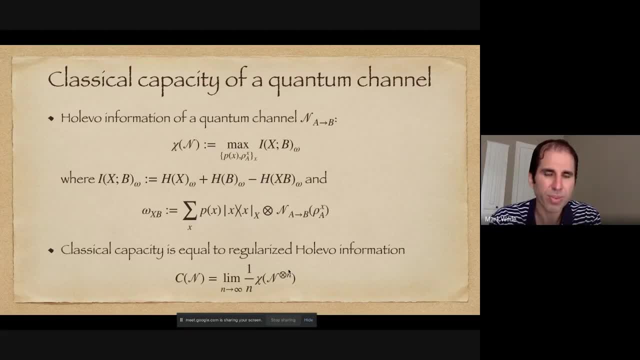 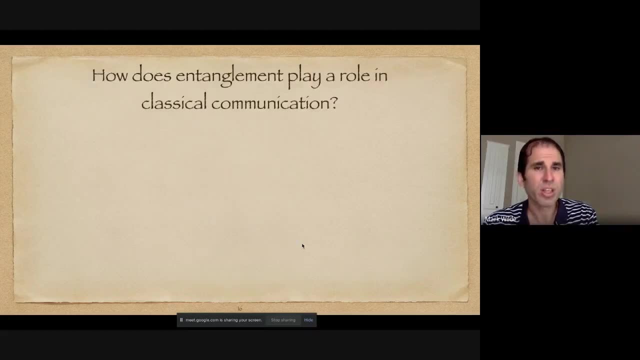 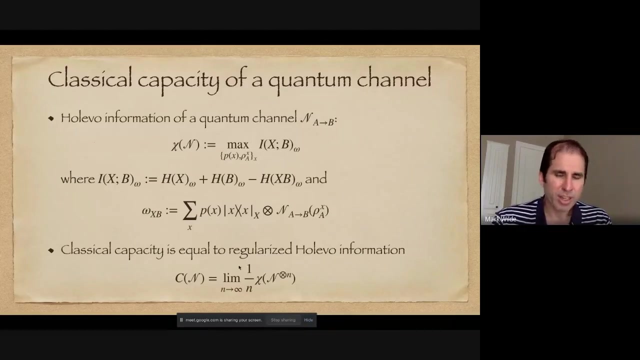 with a collective measurement at the decoder, Okay, and then you could having the limit, as n goes to infinity allows for a general multi-part type, could be very complicated in entangled state. okay, That's the classical capacity. Unfortunately, this is only a formal. 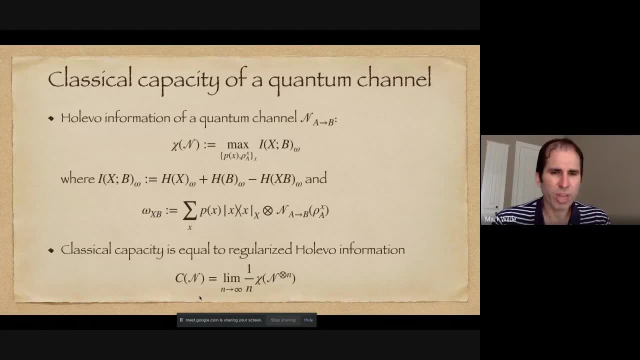 mathematical expression. This does not give you an algorithm to compute the capacity And you can try to approximate it. So there's been a lot of research and a lot of work on finding lower and upper bounds on the classical capacity. The Halevo information itself is a lower bound. 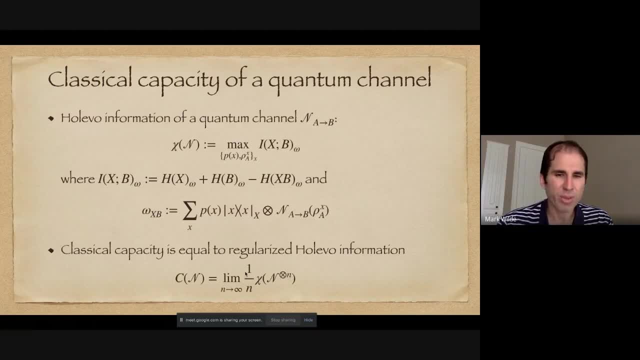 You can prove that you can evaluate this expression: for little n equals one, for little n equals two, for little n equals three, et cetera. You can prove that the quantities monotonically non-decreasing with little n okay. 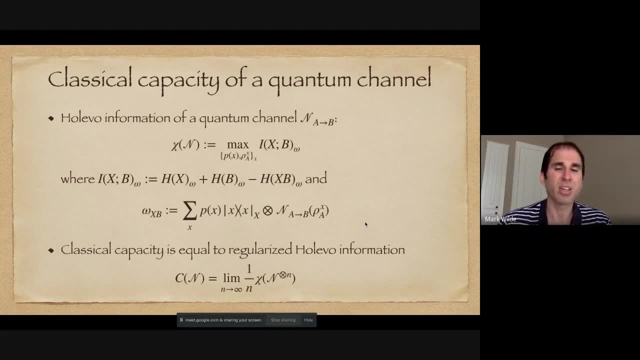 The limit does exist. You can also prove that it will converge to a finite quantity. for finite dimensional quantum channels, For infinite dimensional quantum channels, you need to place an energy constraint on the channel inputs. We're not really gonna get into that today. 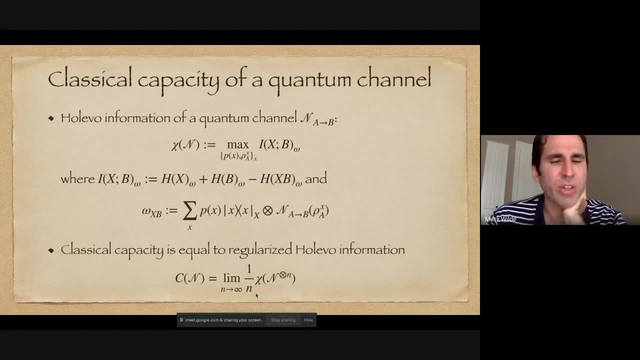 But the point that I wanna stress is that this regularized expression is only a formal expression. It does not give you an algorithm that's going to be able to compute the capacity of a large and a big, open and challenging question is to prove that it's uncomputable. 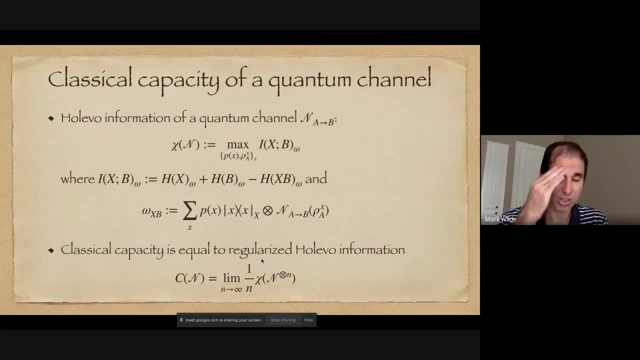 to try to figure out the capacity. So this is in the theoretical computer science sense of Turing. you know, If you, you know, is there an algorithm that will stop in just a finite amount of time? Is there an algorithm that will stop? 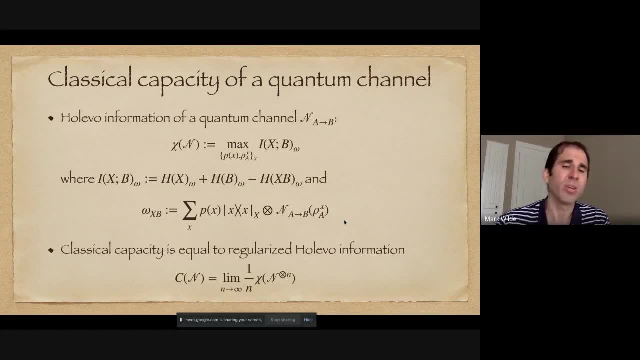 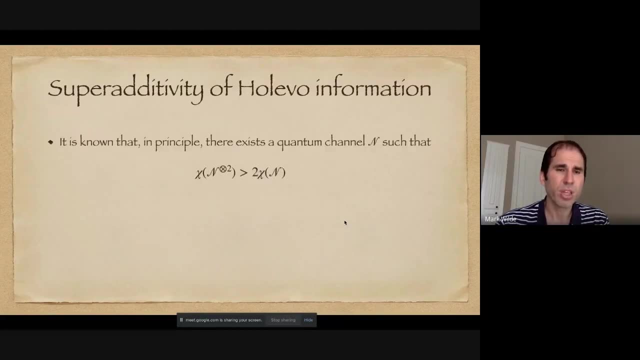 in just a finite amount of time to calculate this quantity. Even that is an open question, you know that has not been answered. So that's an interesting question. Okay, Let me talk about this super-additivity. So there's a result of Matt Hastings. 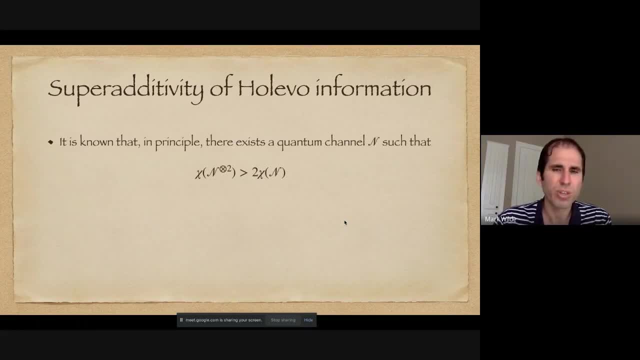 following on work of Patrick Hayden and Andreas Winter. They proved that in principle there exists a quantum channel such that this inequality holds strictly right, So we can divide both sides by two, and then you would recognize that as an instance of this expression here, right? 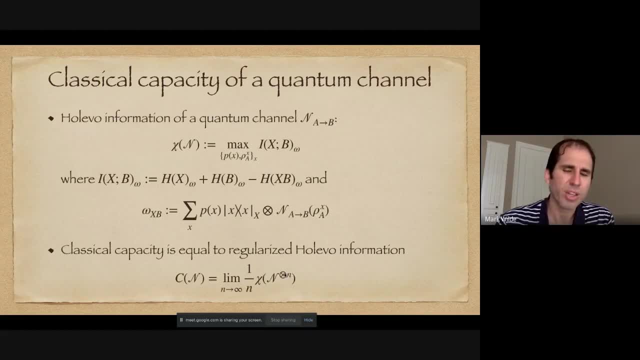 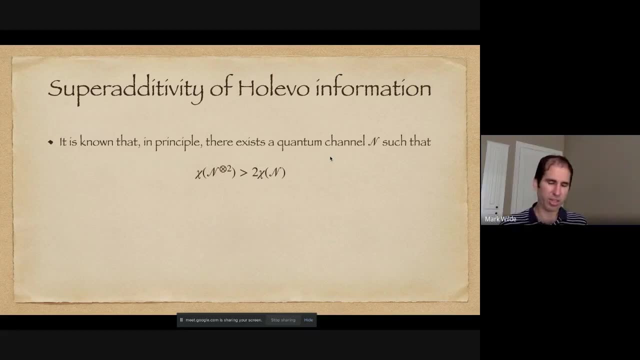 When n equals one, it would be the right-hand side. When little n equals two, it's the left-hand side, right. So they proved that there exists a channel such that this inequality holds strictly, And the conclusion of that is that entangled code words. 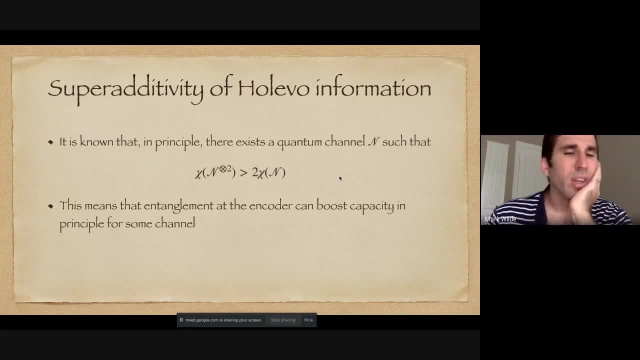 that the encode word can boost the capacity. Why do I say in principle? the way that the argument went is it was a probabilistic argument. They picked the channel at random and then argued that among all the channels generated randomly in this ensemble, 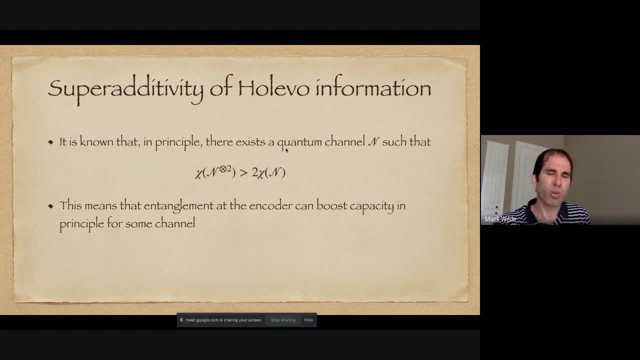 there exists at least one for which the strict inequality holds. So what remains open is to find, you know, to find an explicit example of a channel. This is a major challenge. I believe there was progress on this problem from Pranab Sen, who is in India at TIFR Mumbai. 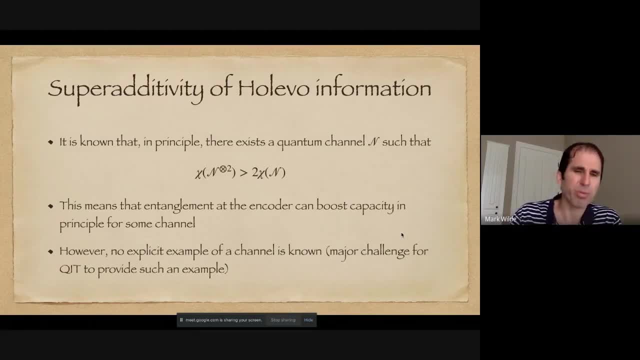 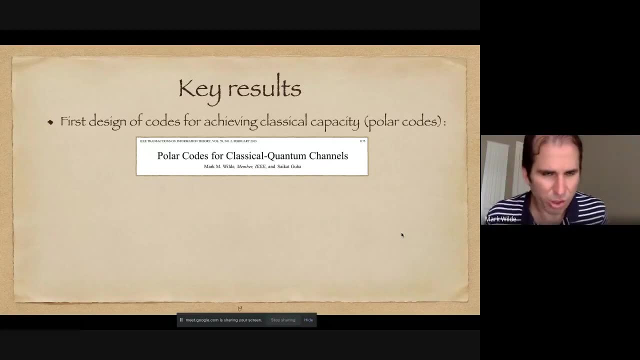 If you look him up in the archive, you'll see a fairly recent paper about this. Okay, so I'm gonna tell you about some things that I've done to contribute to the topic of classical capacity. So far, we were just talking about codes. 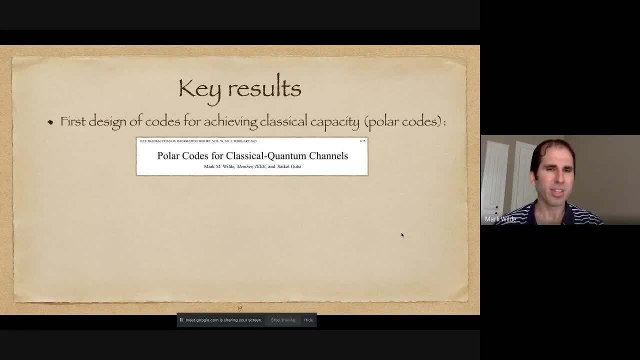 We were talking about capacity, right, And there's a question of like: well, how do we achieve the capacity? And there's a method that my colleague, Saikat Guha and I- Saikat is from Patna originally, but now he's a director for the Center for Quantum Networks- 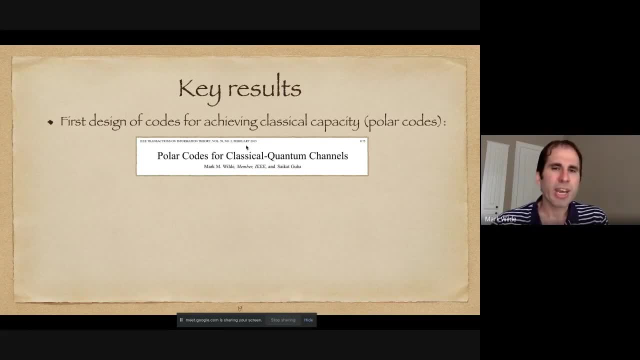 at University of Arizona Back in 2013,, we designed what are called polar codes, following on the classical theory of polar codes, which- the classical polar codes- are now being used in the 4G standard. So we used a lot of those ideas to design polar codes. 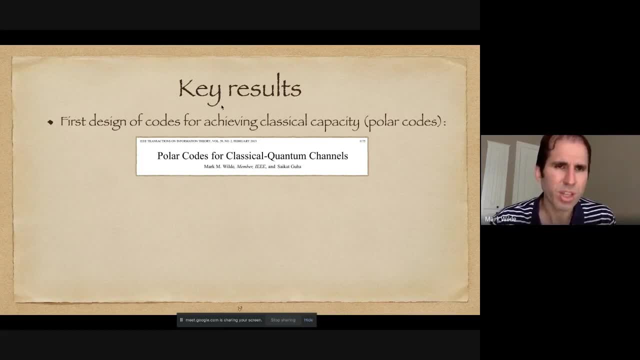 for communicating classical information over quantum channels, And we proved that these codes can achieve the classical capacity. So it was the first of its kind. There are questions about how to implement the decoder efficiently, So if you look in this paper, you'll see that that question is mentioned. 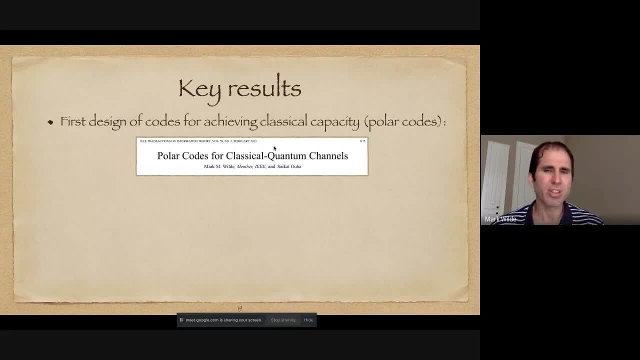 I would say that's a very important question for practice. Saikat has recently been working with Kaushik Sesadrishan, who's a former PhD student with me at LSU, and the late John Dowling, And so they had a paper where you know. 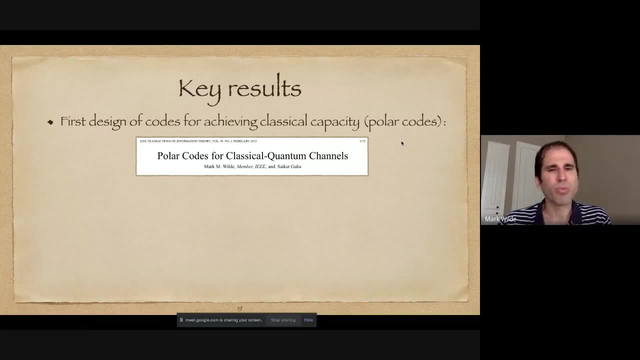 they had a computer where they were trying to implement decoders for polar codes on an ion trap quantum computer. You know, back in 2013,. I never would have thought we would be doing that now like programming quantum computers, but the progress has been so rapid. 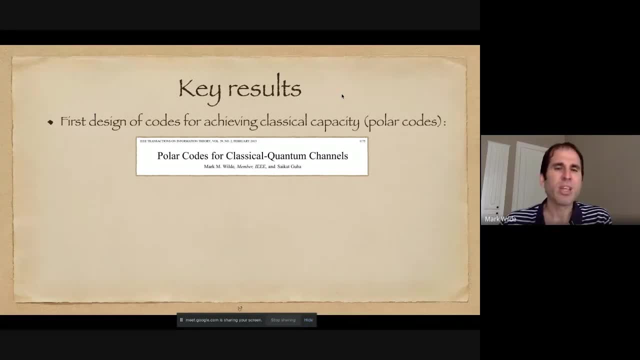 that there's all kinds of possibilities available now, And so they programmed the ion trap quantum computer to try to implement. So you know there's a lot of things that you could do. So you know there's a lot of things that you could do. 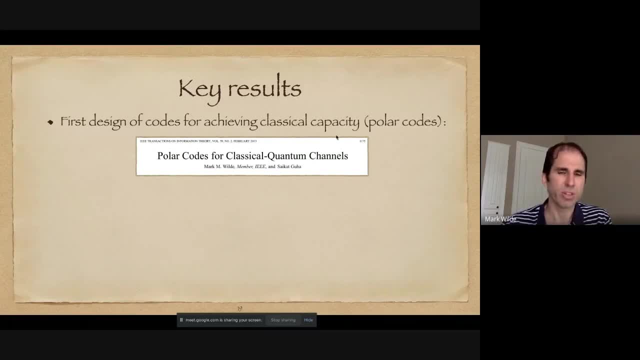 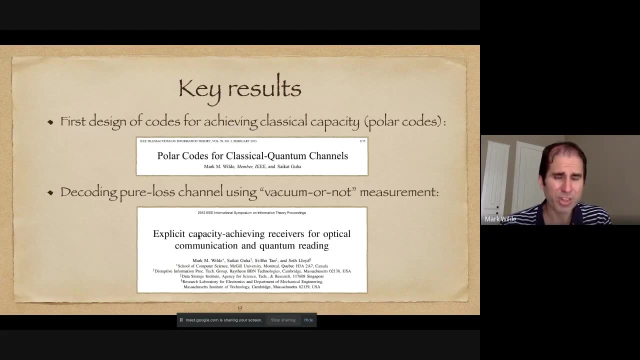 So you know, there's a lot of things that you could do, So I think this is a decoder for error correction. Okay, Another result I want to mention is for the pure loss channel. That was what we mentioned earlier as a special case of thermal channel. 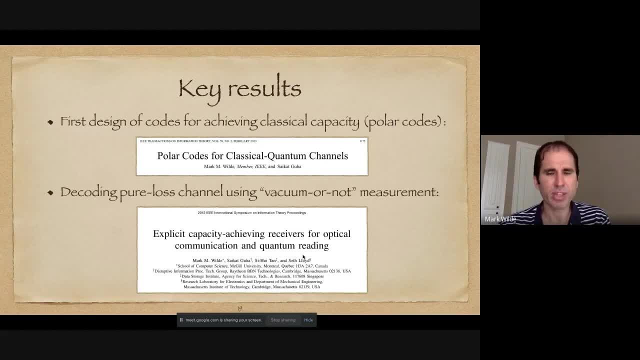 in a paper with Saikat back in 2012 and Seth Lloyd and Seth's former student, C Hui Tam, we showed a particular quantum optical design of a decoder that, in principle, could achieve the classical capacity of the pure loss channel. 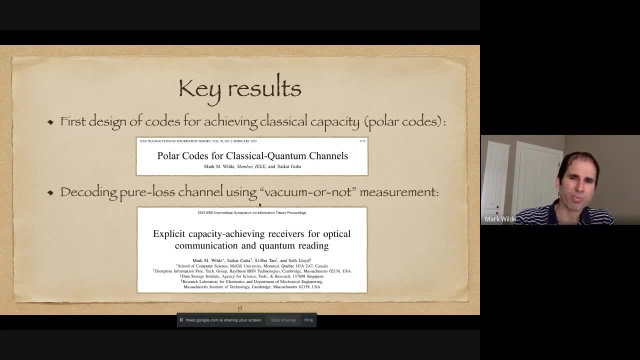 And a critical component of this method was what we call vacuum or not measurement. So this is a measurement that – it's a two-outcome measurement. Either it projects into the all-vacuum state, the tensor product vacuum for N modes, or it projects into the orthogonal complement. 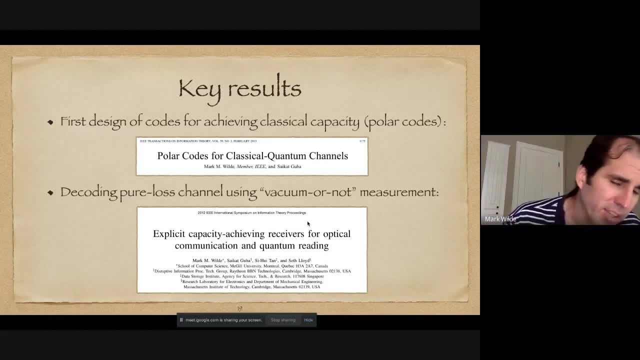 What's very important, related to the measurement disturbance principle, is that the projection onto, not vacuum, the orthogonal complement of vacuum, the resulting post-measurement state, should be the original state with the vacuum subtracted out. Okay, And so that's very hard to do experimentally. 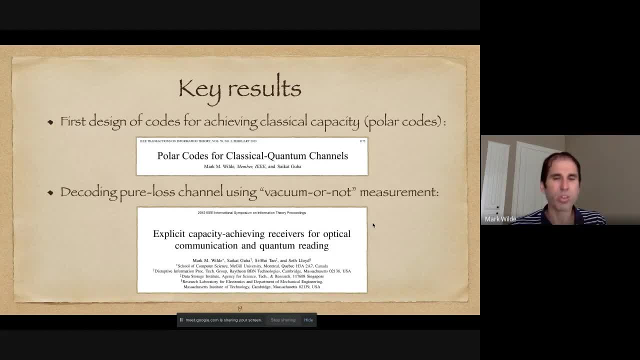 and I would say an important open question is to come up with designs for how to implement this vacuum or not- measurement. There was a proposal back in, I believe, 2012,- 2013.. If you look under the archives, the paper was called: 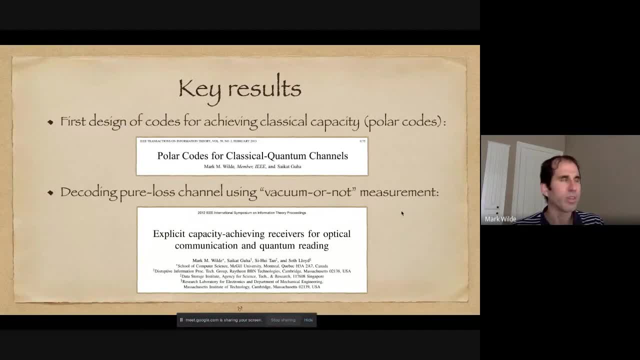 Measuring Nothing. You know it's kind of a joke title, but it was about measuring the vacuum, right? So that's why I called it Measuring Nothing, And I believe the editors of Physical Review Letters made them change the title. 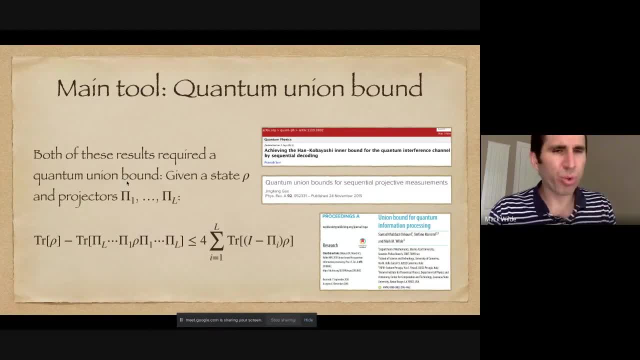 Okay, Something I want to mention is a tool that we used, and it's seen a lot of different refinements. The first instance of this tool was by – I don't know if you've heard of it, but it's called Measuring Nothing. 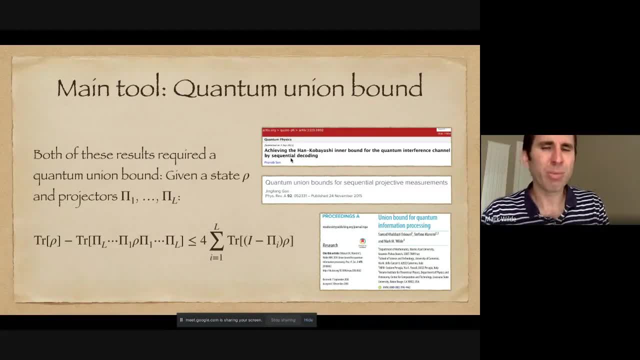 And I believe the editors of Physical Review Letters made them change the title. Okay, Something I want to mention is a tool that we used and it's seen a lot of different refinements. Okay, Something I want to mention is a tool that we used and it's seen a lot of different refinements. 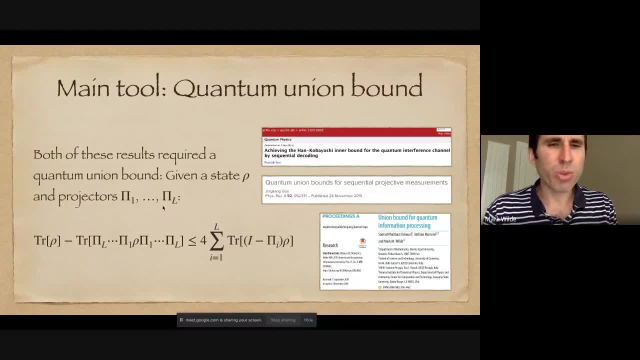 And it's what's called a quantum union bound. So it's this statement here, It's a quantum generalization of the classical union bounds. So the assumptions are that you have a state and a set of projectors- okay. So the assumptions are that you have a state and a set of projectors, okay. 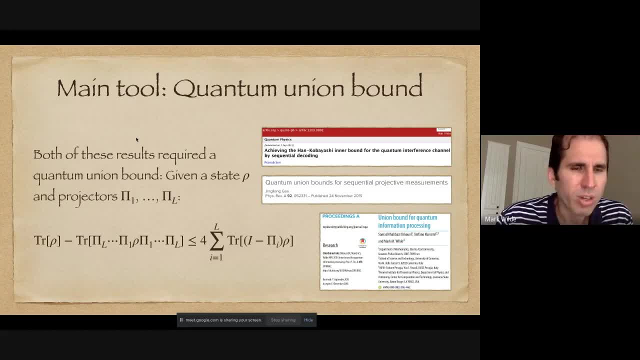 Each projector could be one measurement. outcome of a binary value measurement. Okay, Okay, so what you imagine is that you and you know each binary measurement is like a yes, no question, right, So you can imagine it being used in a context for decoding. 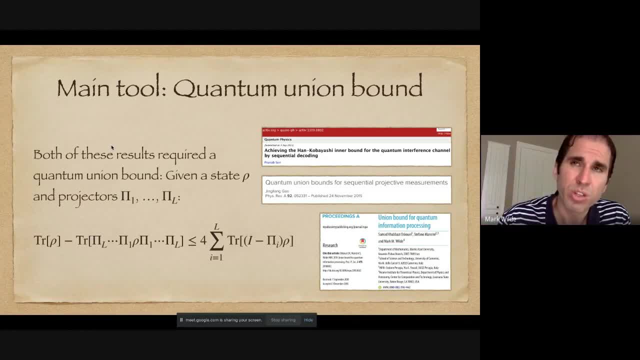 You would have a measurement to ask: was the first code word sent? Was the second code word sent? Was the third code word sent, All the way up for L code words, if there's L messages And this could be a sequence of yes or no outcomes, right, 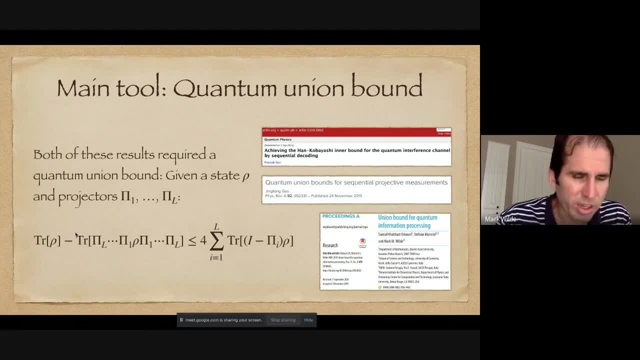 And so this expression right here. this is from the Born Rule of Quantum Mechanics. This is the probability of getting a correct sequence of outcomes from a set of binary measurements. okay, And so it's analogous to the classical union, bound as an intersection of events. 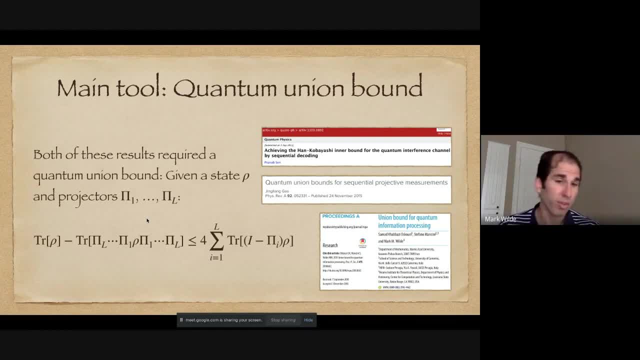 You know the probability that an intersection of events occurs, that all events occur. okay, So it's a quantum generalization of that. In fact, if the probability that the projectors commute, then the classical expression is a special case, All right, so this is like a success probability. 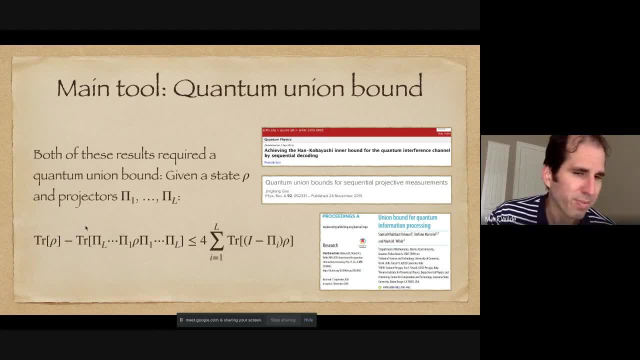 This: if you take one minus that, you get an error probability. okay, So the quantum union bound allows for is for bounding this error probability from above by the error probabilities of the individual events, of the individual projections, the individual measurements. Okay, 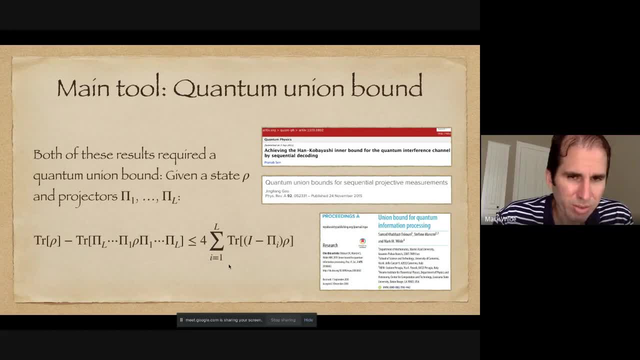 Exactly what you get with the classical union bounds. We need a factor of four. In general these projectors, they do not have to commute, okay, And so there was a recent paper. sorry I didn't list it here. There was a recent paper in the archive. 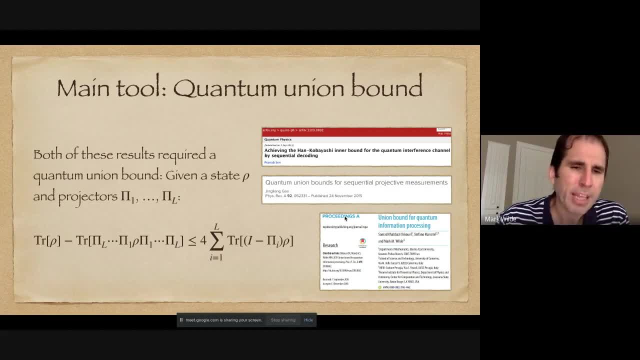 called Quantum Union Bound Made Easy, And they proved that this four is essentially necessary If you have many measurements than this. they proved that this is like close to being you know, this is like close to being zero. This is being saturated. 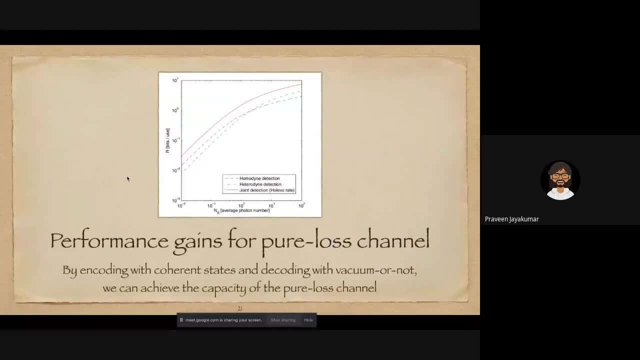 Okay, Excuse me, sir, you have 15 minutes left. 15 minutes, good. all right, I've been talking at a kind of slow pace, but you know, talking carefully about this classical capacity problem, So I'm gonna pick up the pace a bit. 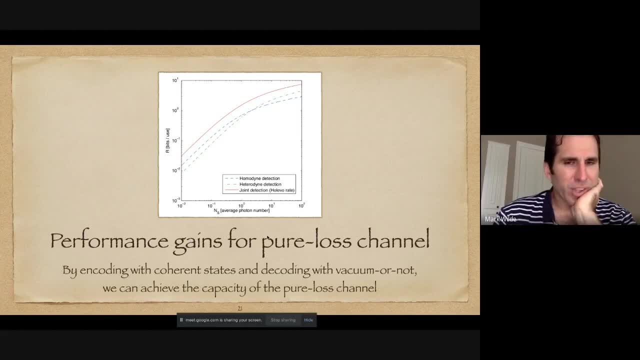 But one thing that I wanna show you is that there can be big performance gains for communication of classical information over a pure loss channel, right. So I'm gonna pick up the pace a bit. So I'm gonna pick up the pace a bit, But one thing that I want to show you is that there can be big performance gains for communication of classical information over a pure loss channel, right. 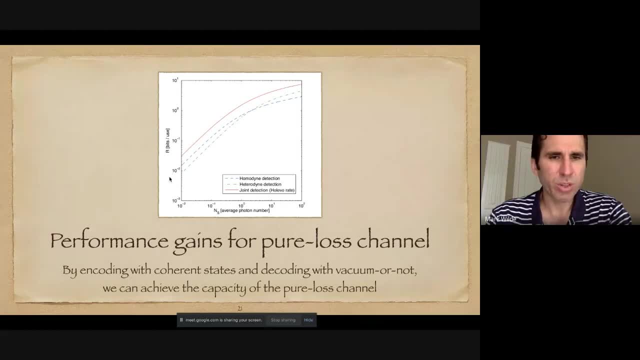 So what we're looking at here is rate in bits per channel use versus photon number at the input of a pure loss channel. So you imagine that your transmitter is limited to send a certain number, have a certain mean photon number And the quantum regime is when that photon number is low. 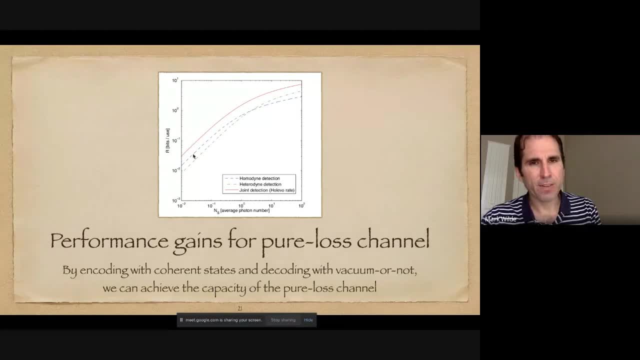 Okay, And what this is comparing is the rate that you can achieve with a collective measurement- is also called joint detection. That's the Hallevo information rate that we talked about previously, And these are traditional classical. these are the rates that you can achieve with the traditional classical detection method, called homodyne or heterodyne detection. 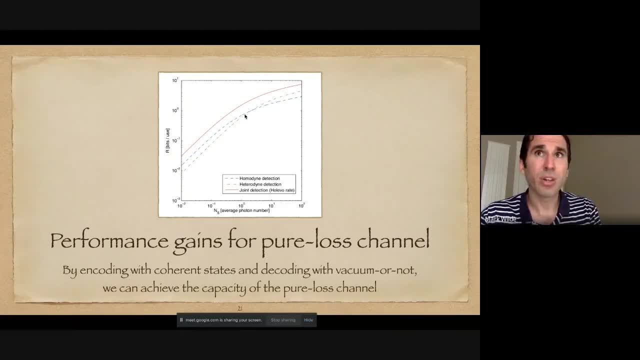 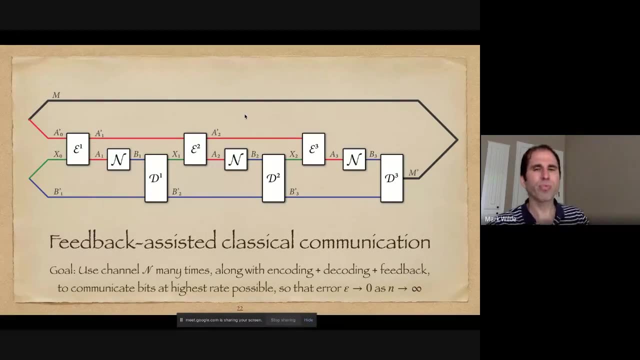 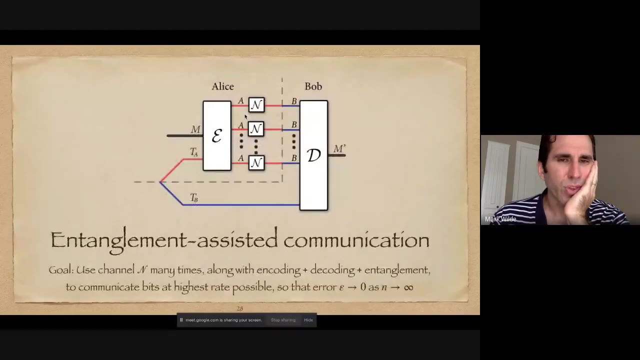 You can see that there can be big gains, you know, by using equivalence. So that's the quantum strategy. All right, I want to mention- I'm going to go ahead and skip this- Since the theme was entanglement. I want to talk about entanglement assisted communication. 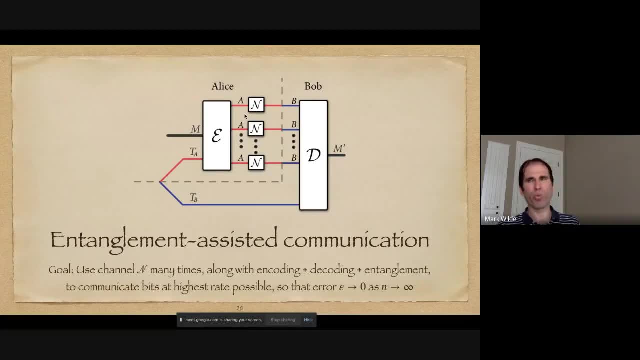 I'm going to talk about this scenario and I'm going to talk about one other that's relevant to quantum key distribution, And then I'll wrap up And I think I should get into time. Okay, So an entanglement: Entanglement-assisted communication. 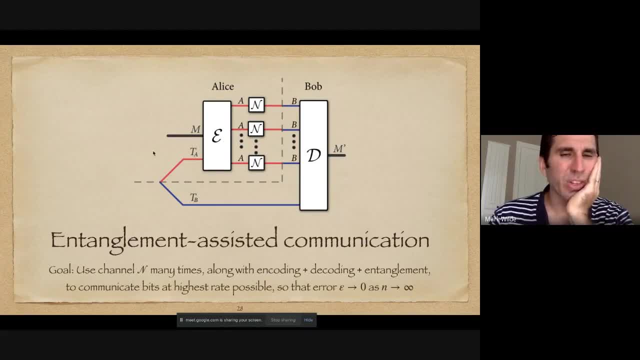 This diagram is a generalization of the superdense coding protocol. Okay, that's what we talked about earlier, So we assume that Alice and Bob are allowed to share entanglement. before communication begins, There's a message M that Alice would like. 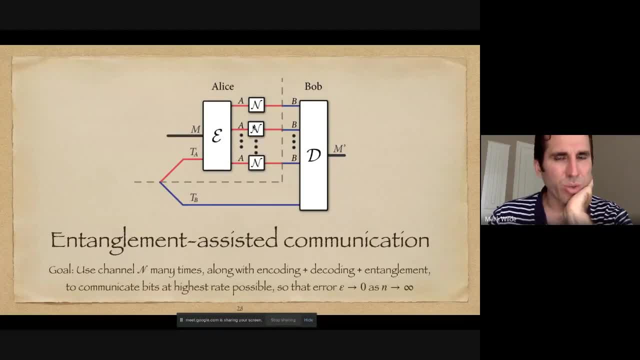 to communicate to Bob. They can use the channel little n times and then at the end Bob can combine his channel outputs with his share of the entanglement to perform a decoding And in general it can be a collective measurement okay. 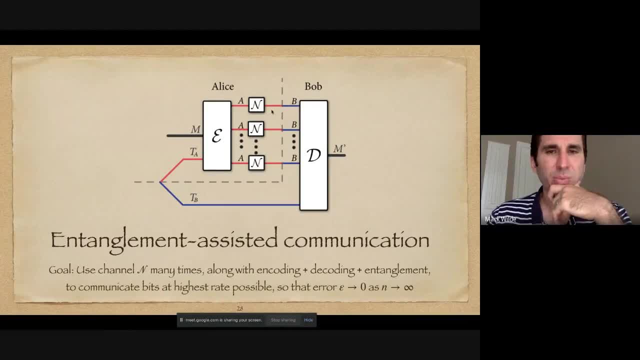 And the capacity is the largest rate of communication, such that the error tends to zero as the number of channel users gets large, and then maximized over all possible encodings, decodings and entangled states they could share. How does entanglement play a role? 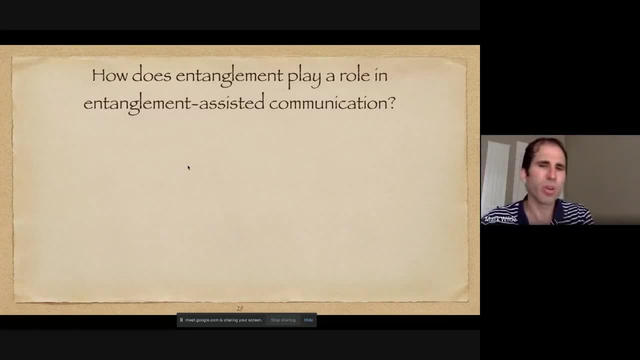 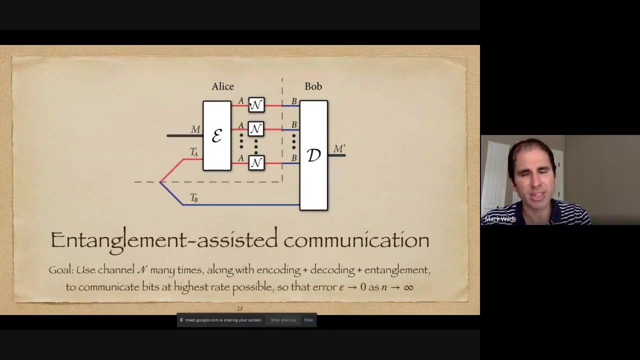 Well, we said it's a generalization of superdense coding. already you see that there's this entangled state and even if the channel has the property, that's called entanglement breaking. so that property is like with a single channel use. 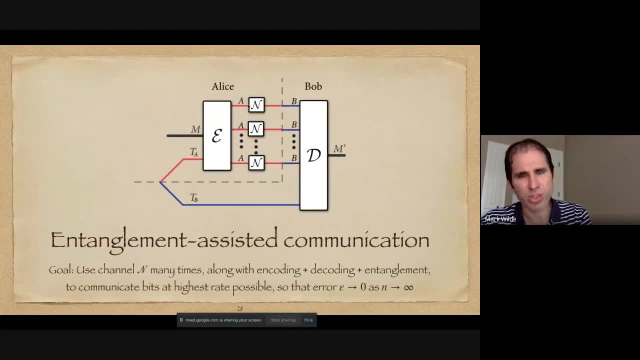 if Alice were to send in one share of an entangled state, then the resulting state is separable. It's actually known that even if the channel is entanglement breaking, they should have a share per se as a result breaking. having this entanglement assistance can increase the capacity okay, so that's interesting. 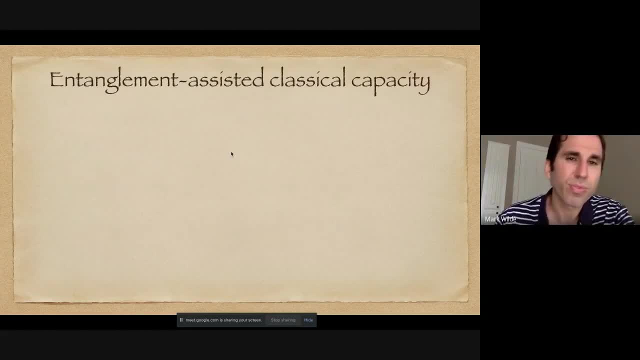 and quite useful. um, so what? what do we know about entanglement, assisted capacity? well, there's a very beautiful result. this, i would say, is the the nicest generalization of shannon's formula for the classical capacity of a classical channel. so this quantity is the mutual. 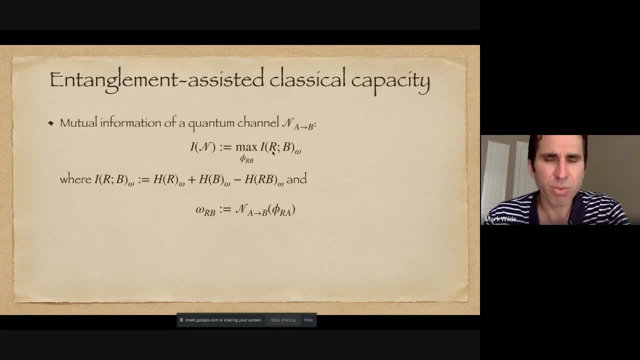 information of a quantum channel. previously we talked about halebo information. it's very similar, except we replaced the classical x with a quantum r, so now it's a true quantum mutual information between a quantum system and a quantum system. the quantum mutual information is defined the same way, but it's with respect to a different bipartite state. so we imagine: 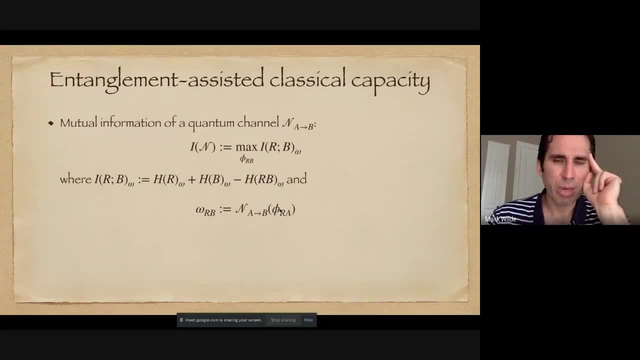 that alice sends in one share of a pure bipartite state, sends in the system a to the channel, the channel acts on, it produces a system b in the state omega rb. then if we evaluate the mutual information with respect to omega rb and maximize it over all inputs to the channel, that's the 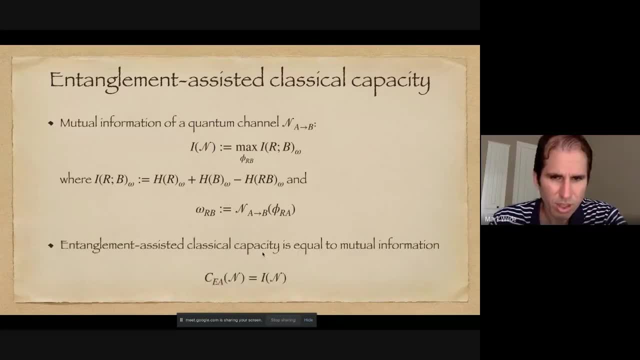 quantum mutual information of a quantum channel. the wonderful formula, the wonderful result proved by uh bennett, shore smolin, and that happily all in 1999, is that we have this formula for entanglement assisted capacity. so the entanglement assisted capacity is operationally defined. it's equal to: 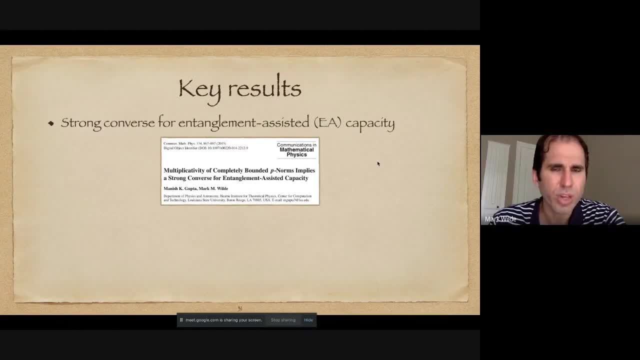 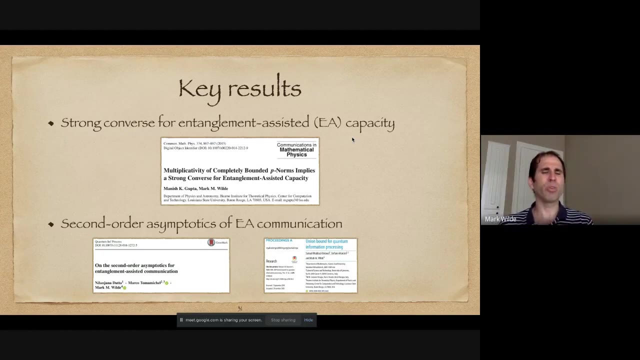 the mutual information. okay, um, these are just showcasing some papers that i've written on this topic. uh, one of them was with the student manish gupta. it's about, um, you know, he's a former student of lsu. now he's he's doing a postdoc in india. 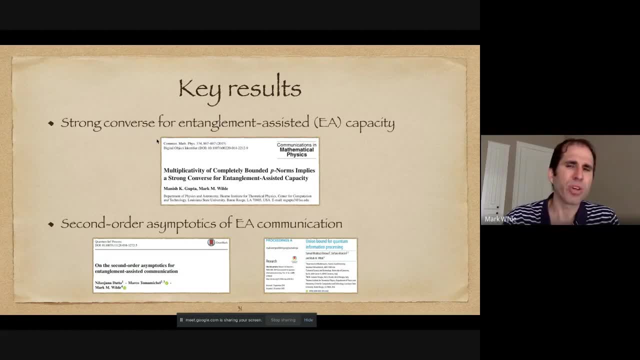 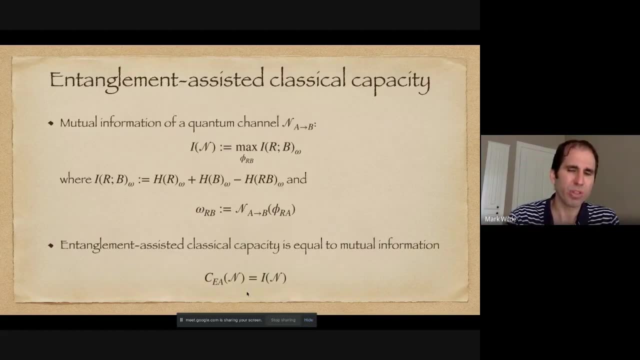 um, and we, we proved a strong converse for entanglement assisted capacity. this means that, uh, this mutual information formula is a very sharp dividing line between what's possible and what's impossible. the strong converse says that if the rate of communication exceeds the mutual information probability actually converges to one, you know. so it's like there's a there's a sharp dividing line. 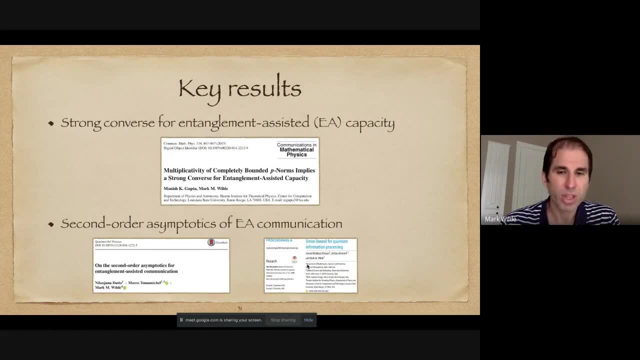 between, uh, what's possible and impossible. and then these are some other things that i've worked on: one with nalanjana data, who's originally from calcutta, and, um, these other collaborators, we're looking at something called second order asymptotics. i'm going to skip that right, let me. 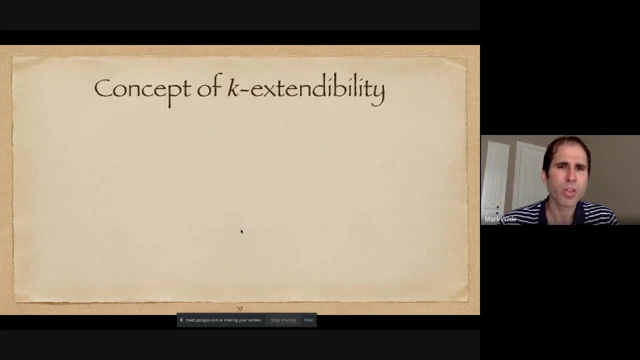 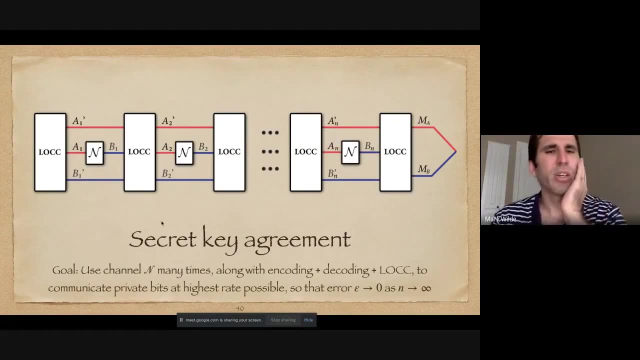 skip a bit. i want to talk about um. do you want to talk about this? okay, so this right here is a model of quantum t distribution. okay, this is like a information theoretic model of quantum key distribution. this is something that psychot guha and i and masahiro toka, masahiro takiyoka. 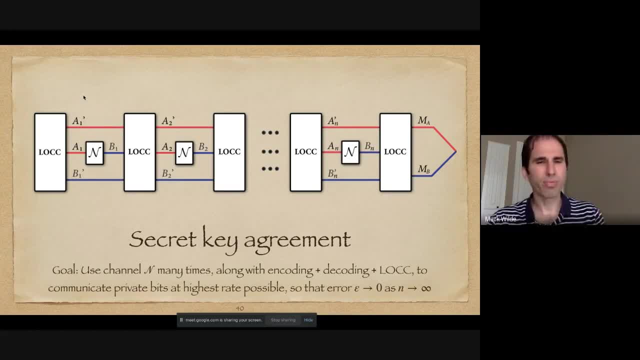 in 2013. we worked on, so we, we defined this model, find this model of communication as a model of quantum key distribution. So what is meant by it? in between every channel use, Alice and Bob are allowed to perform arbitrary local operations. in classical communication, The classical communication can be leaked to an. 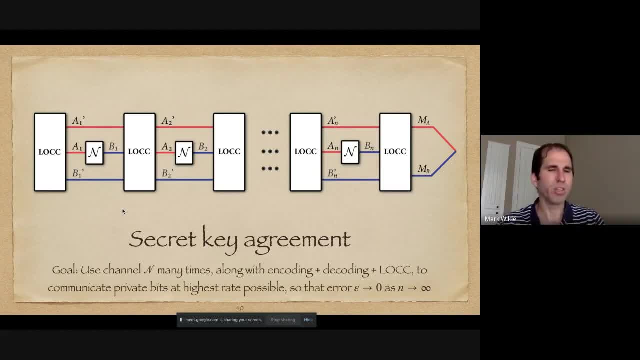 eavesdropper, so it's actually public classical communication. And there's a concept that I didn't talk about in so much depth. but every quantum channel has an environment. We saw that in the model of the thermal channel. We saw that all the photons that don't make 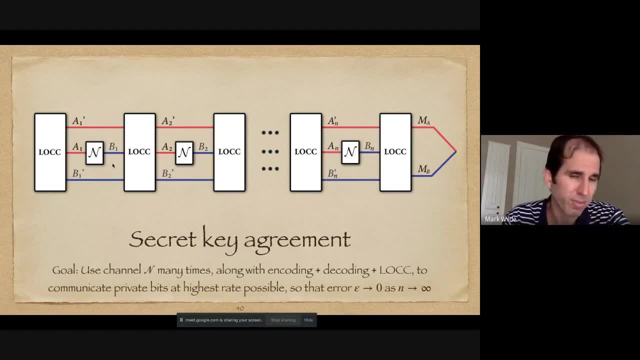 it to Bob, they go to the environment. So in this model we assume that the eavesdropper has access to the classical data being exchanged between Alice and Bob and the environment of every channel use. We assume that the laboratory of Alice and Bob are physically secure. Okay, So in between, 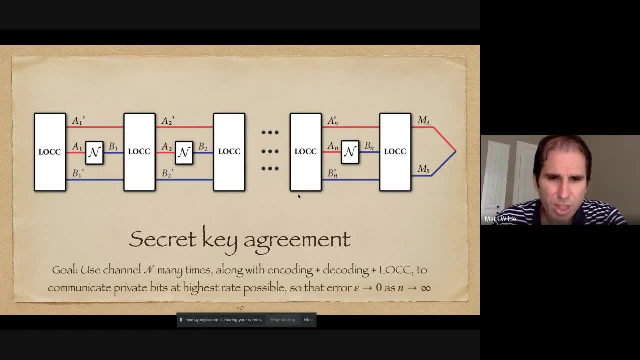 every channel use. they're allowed to do LOCC and they're allowed to use the channel little n times. The goal of the protocol is to generate a secret key, So the secret key is a secret key state. The secret key state is uniformly random, perfectly correlated and different. 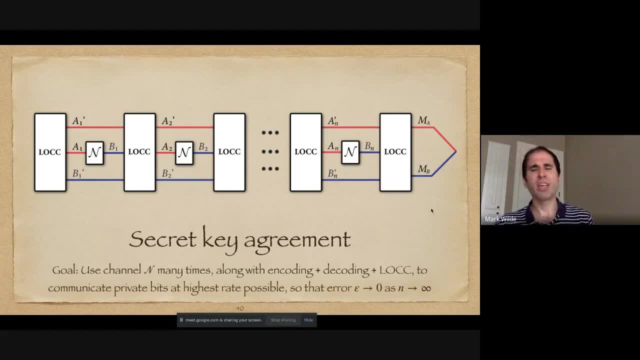 Independent of Eve. Okay, And then that's the ideal thing. But in practice, what they generate is an approximation of that. Okay, And what we call a secret key agreement capacity is the- you know, the rate at which private bits, the largest rate at which private bits. 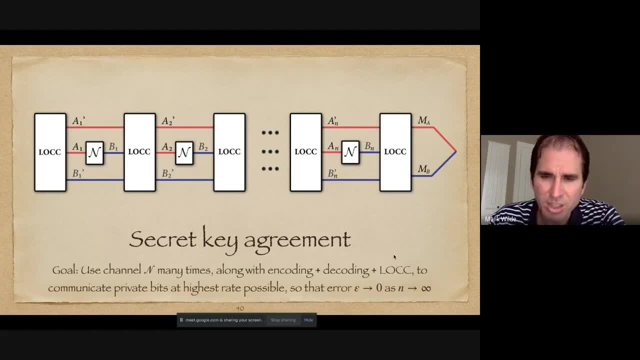 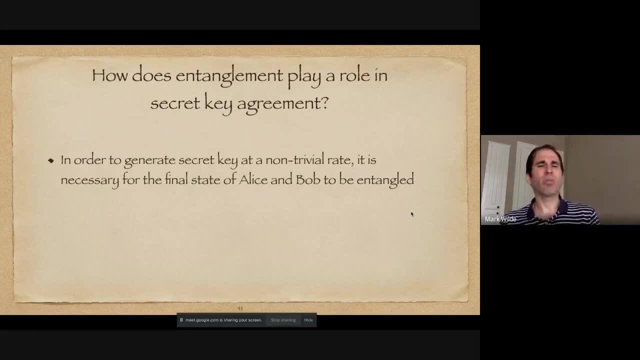 can be communicated, such that this approximation error tends to zero as the number of channel uses becomes large. Right entanglement play a role. What's known is that, in order to generate secret key at a non-trivial rate, the final state of Alice and Bob must be entangled. 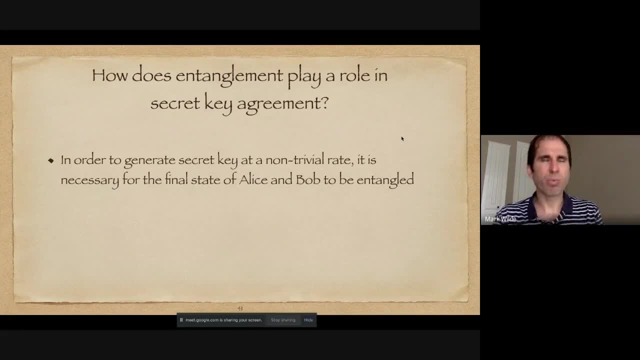 If it's separable, then you know, we saw with the separable form there's this classical data in the background, the P of X that we had in the original, the early slide, And if that X is known, then the state of Alice's and Bob's system. 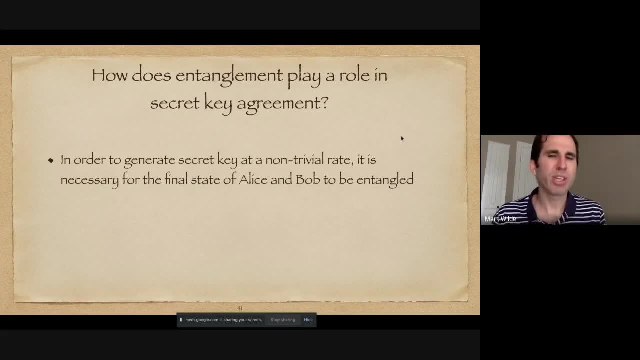 is a product state and it's impossible to generate a secret key from a product state. So in principle, if the protocol makes a separable state, the eavesdropper could have that classical hidden variable in the background. okay, So that's kind of the intuition for why it's necessary. 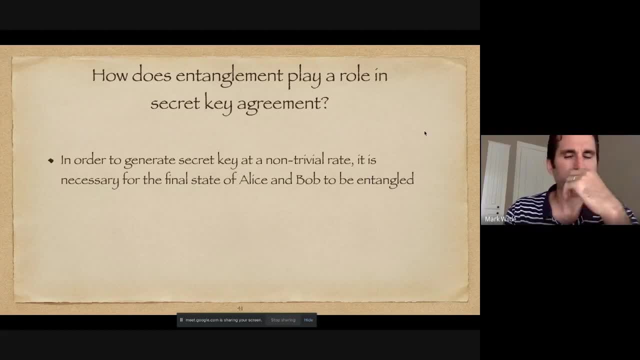 for the state at the end of the protocol of Alice and Bob to be entangled, Okay, And then another way that entanglement plays a role is that entanglement measures are useful as upper bounds and secret key rates. We talked about the interest in knowing. 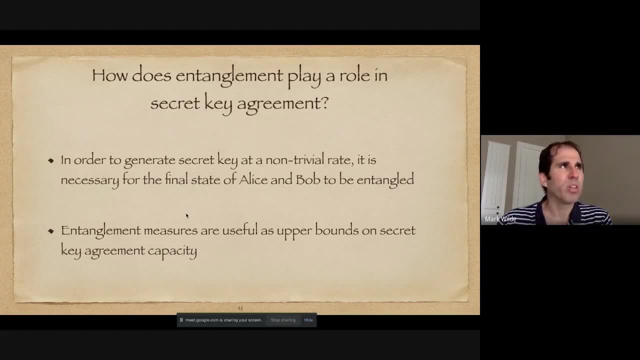 the fundamental limits of communication. Well, since quantum key distribution is such an important protocol, we're interested in knowing what is the largest rate you know at which we can do quantum key distribution securely, And so, to tackle that problem, you can use entanglement measures. 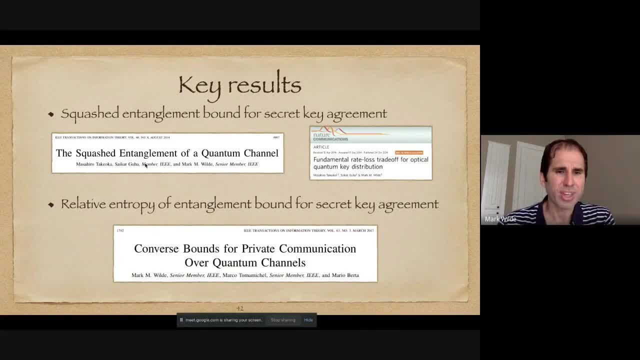 And so that's something I've worked on. This was with Saikat, and this paper was with two others, Marco and Mario, And in these works we showed how squashed entanglement, which is an entanglement measure based on conditional mutual information. 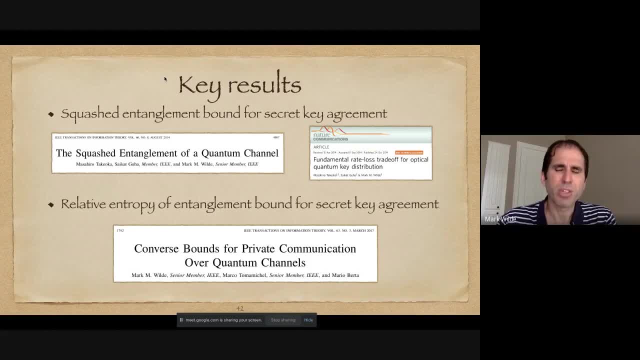 we showed how that gives an upper bound on quantum key distribution And then in a later work we showed how relative entropy of entanglement gives an upper bound on quantum key distribution And we showed a strong converse rate, showing, as a final point, distribution. 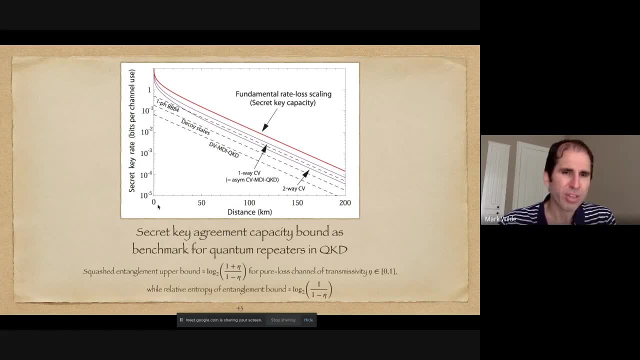 Okay, So this plot is showing you secret: key rate versus distance. So for the pure loss channel, the transmissivity parameter that you can calculate as a function of distance, You know, there's for a fiber optic cable that's characterized by something called an absorption. 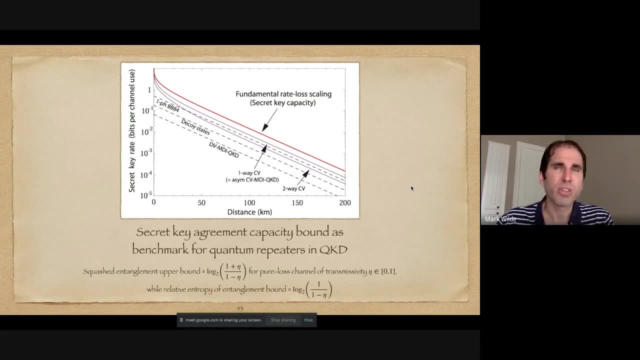 the transmissivity decays exponentially with the with the distance. and so you know, there's a there's, there's a direct mapping between the transmissivity and the distance. and so in this plot, since experimentalists or, i think, the general public would be interested in like 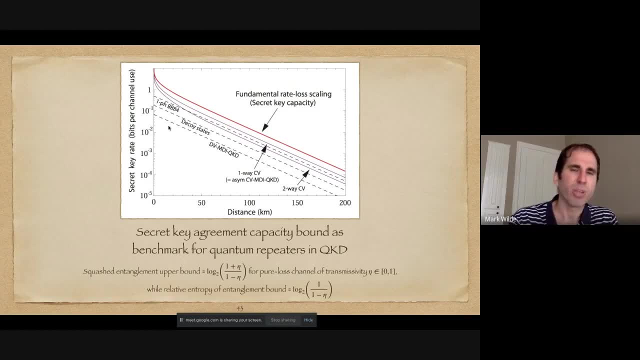 uh, over what distances you can do qkd. this plot is interesting, so what it's showing is the rates that a number of protocols can achieve that are like some well-known protocols, and then this is showing the fundamental limit. okay, squash entanglement gives you this upper bound. 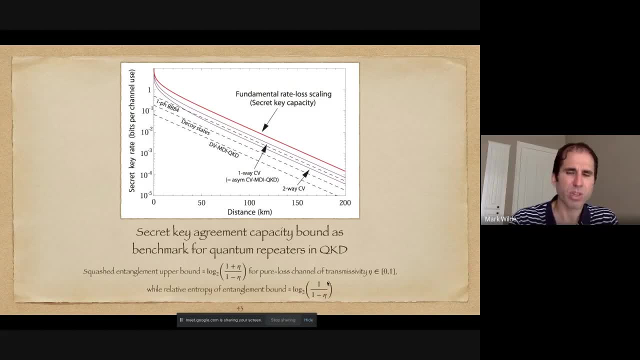 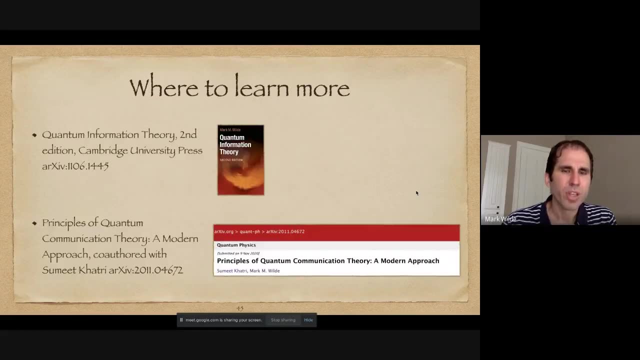 relative entropy of entanglement gives you this upper bound. i don't know if i'm going to say much more than that. all right, um, i'm wrapping up now. um, this is the book, uh, that i wrote in 2011 and put in the archives. 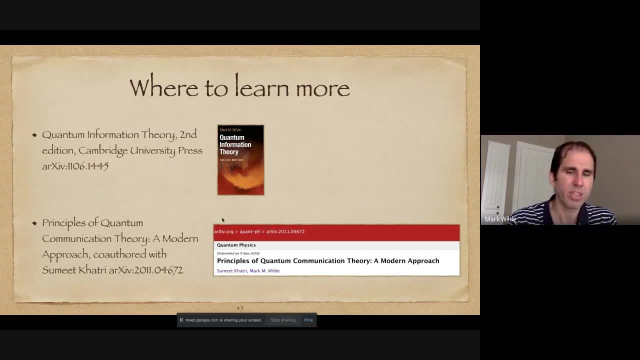 and there was a second edition published in 2017.. this is a recent book that sumit and i we're still writing it. it's a book in progress, but we put what we have on the archive and there's a lot of content there. this book first focuses on 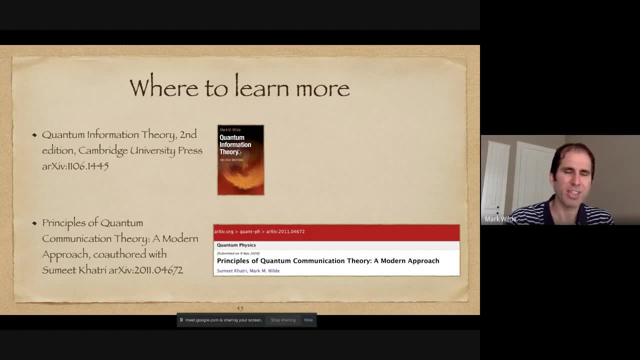 von neumann, entropy and concepts like typicality and typical subspaces. this book focuses on renny entropy, what's called one-shot entropies, and connections to hypothesis testing and it. you know, this book kind of summarizes everything that was happening in quantum shannon theory before around. you know, 2010, and then this book focuses on 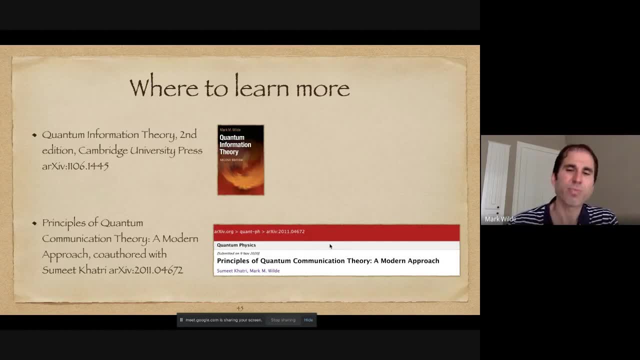 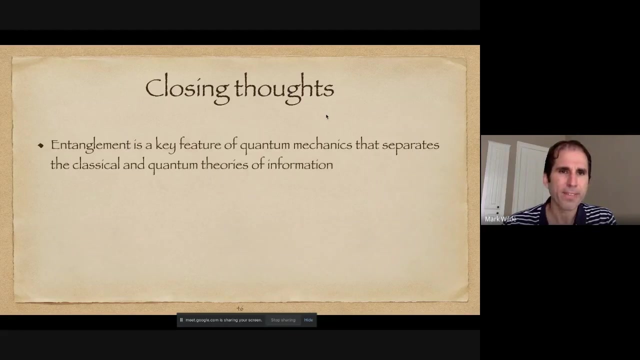 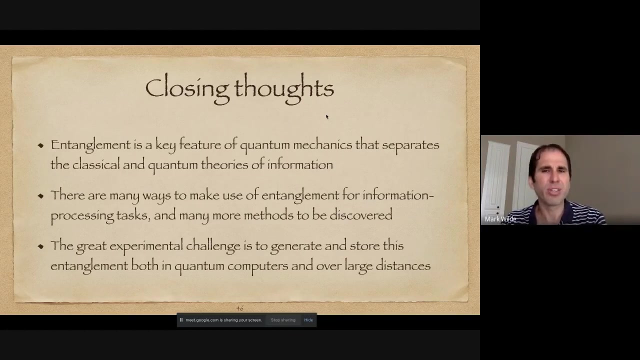 everything that's been happening in the past decade. okay, i also gave a lecture series on entanglement for the she quantum organization, which is an organization founded by a woman in india. it's meant to, um, support, you know, women pursuing, uh, quantum information science. okay, so, wrapping up, entanglement, this was the theme of the talk. i was showing you how it it is a. 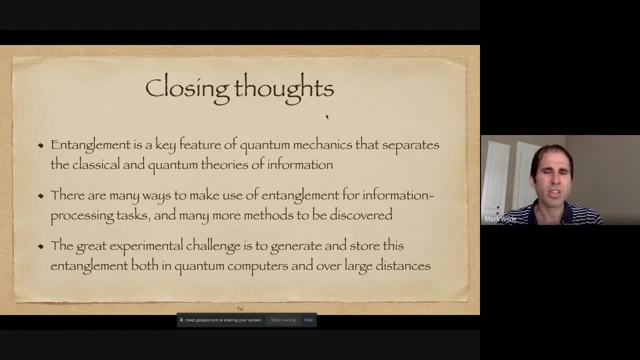 you know feature of quantum mechanics, that is, a strong separation between classical and quantum theories of information. we talked about many different ways for making use of entanglement. we talked about super dense coding, teleportation, the, the chsh game. we talked about classical capacity, entanglement, assistant capacity. we talked about secret key agreement. what i didn't talk about, 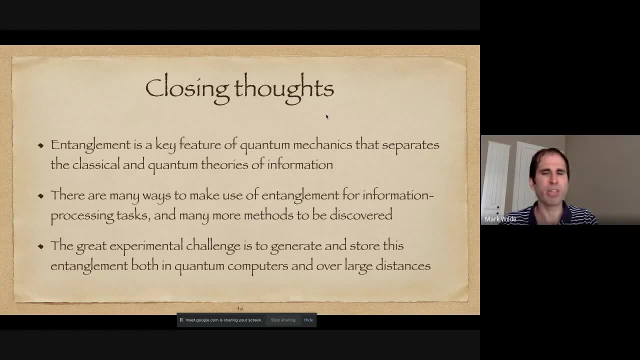 is feedback assisted capacity, quantum capacity. those are other kinds of capacities and it's really a big experimental challenge to generate and store this entanglement. but, um, we're seeing remarkable progress. you know, we i talked about the loophole free bell test that was conducted. that kind of thing is necessary for large-scale quantum networks. and then also, uh, the 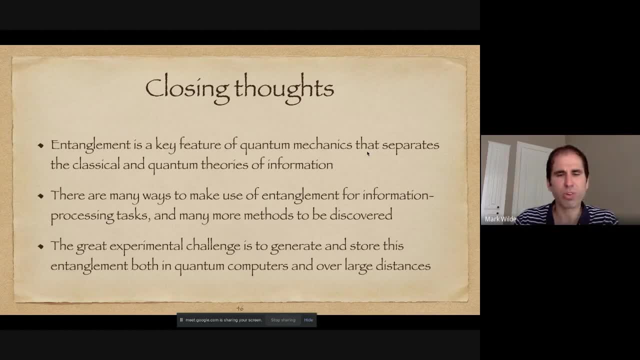 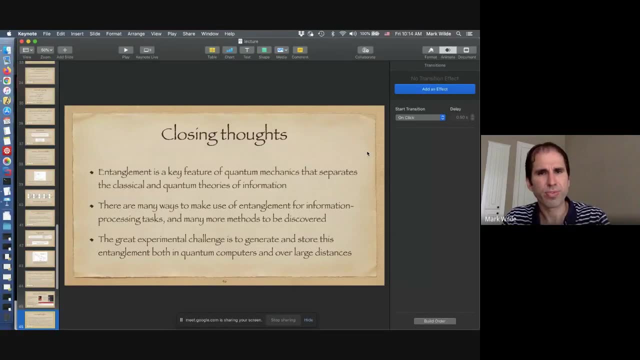 ability to generate entanglement is important for quantum computation. with that all in mind, thank you. thank you very much, professor, for a wonderful talk. i'm sure everyone found it as useful as i did. uh, we will take any questions right now, if anyone has, so you can leave them in the chat box or unmute yourself. 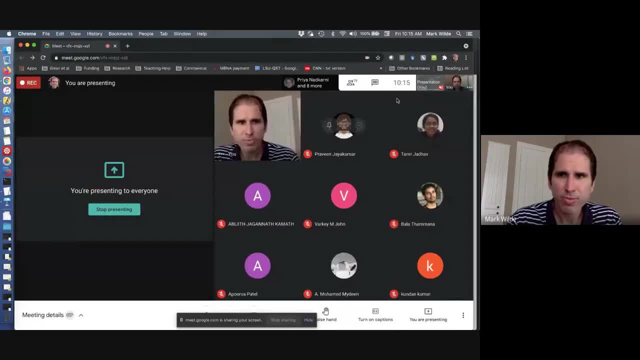 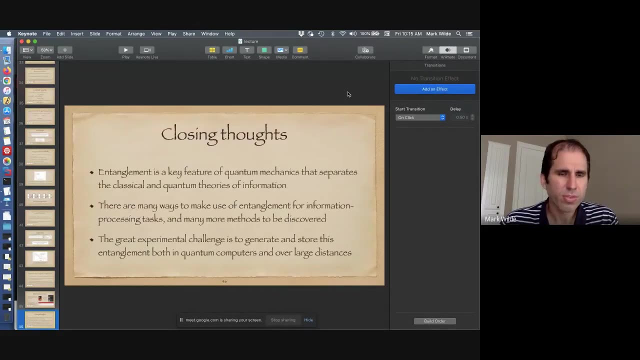 oh, should i go to the chat box? uh, it's fine, i'll take a look, okay. okay, um, um, good morning, professor mark. uh, my name is priya. uh, yeah, my question is like: on one of your slides it was mentioned that entanglement, assisted communication is like 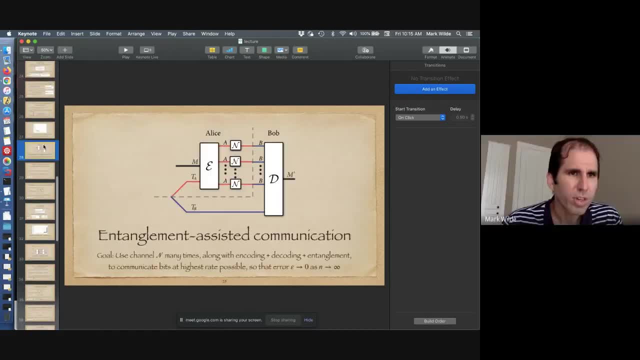 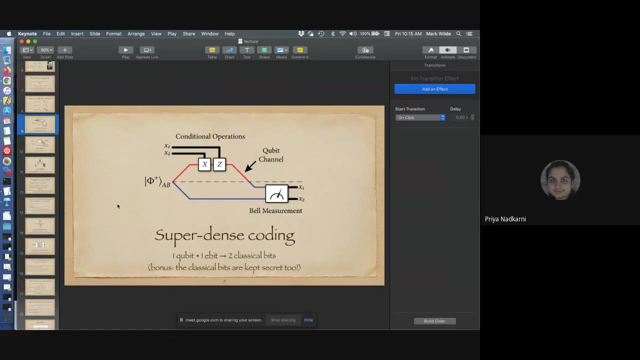 a generalization of superdense coding. yes, yeah, so, uh like uh, super dense coding involves uh like, uh, basically encoding uh classical information in quantum states. so, uh, in entanglement assisted communication. isn't the information also quantum in nature? isn't the what uh? information also quantum in nature? oh, um, so so the goal of 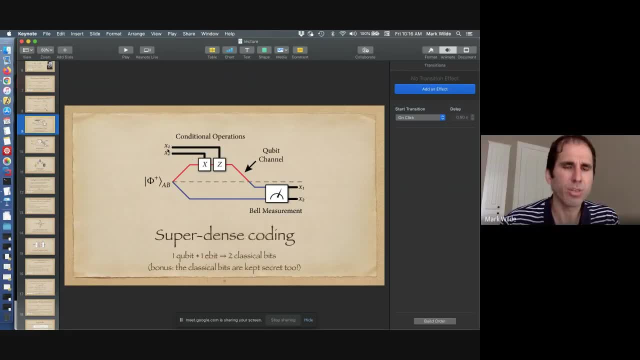 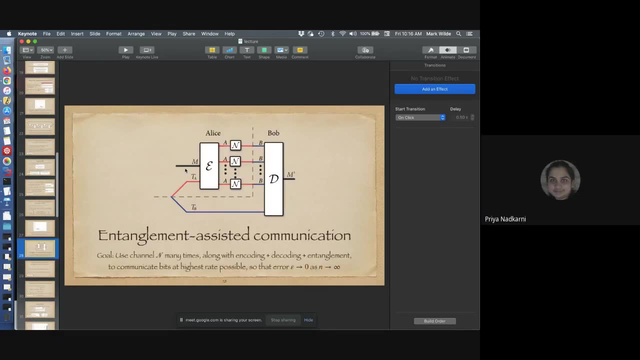 super dense coding is to send these classical bits right and when entanglement assisted communication. we're still trying to simplify, okay, so the message m is still a classical message, is it? yes? however, um, there is a version of entanglement communication where you can try to send quantum information. 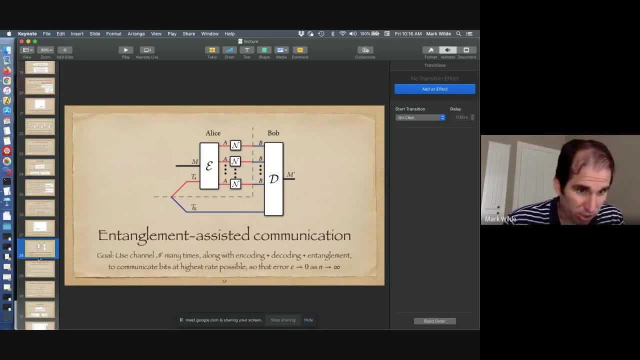 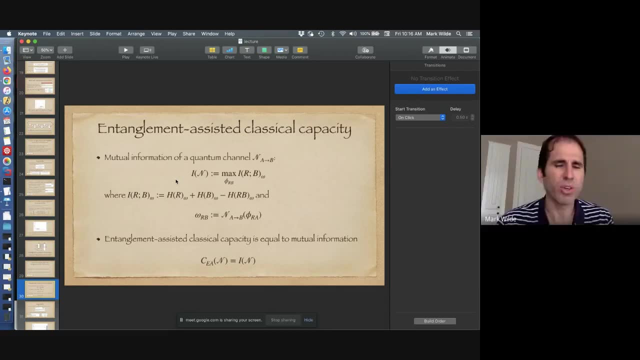 i didn't. i didn't talk about that, but it's an interesting question and, due to the connection between teleportation and super dense coding, it's known that the entanglement assisted quantum capacity is half the mutual information. okay, nice, okay, yeah, yeah, thank you. thanks for your question. uh, next, uh, i, i have a. 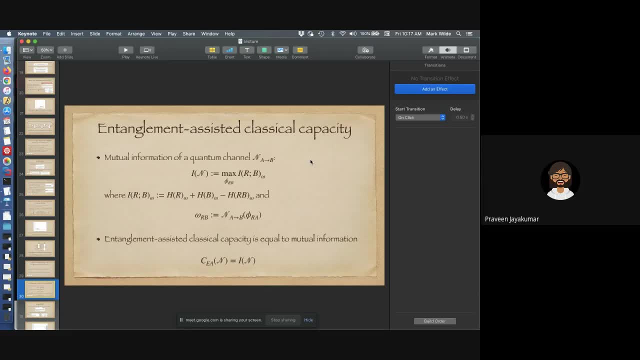 little question of my own, uh, rather a general question, uh, with regard to entanglement measures. uh, so, uh, i've come across some entanglement measures which tries to quantify, say, for more than two systems. yeah, uh, just speaking about a measurement of entanglement between more than two systems, make any sense, or 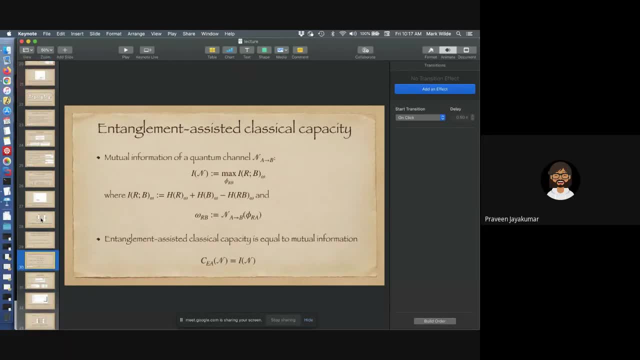 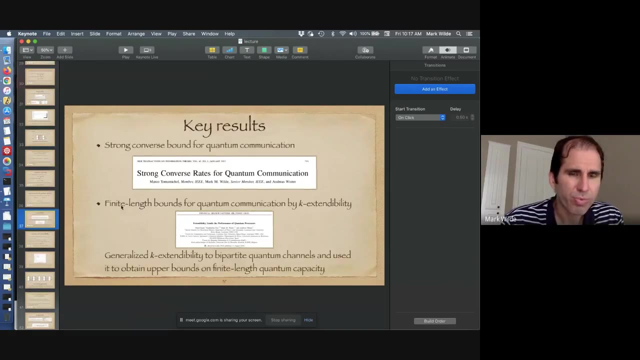 right as of now, they seem to be designed for particular purposes, to quantify for particular purposes. so, uh, is it right to think about a notion of entanglement between more than two systems? definitely, um, so that's a that's a good question and that is relevant for uh. 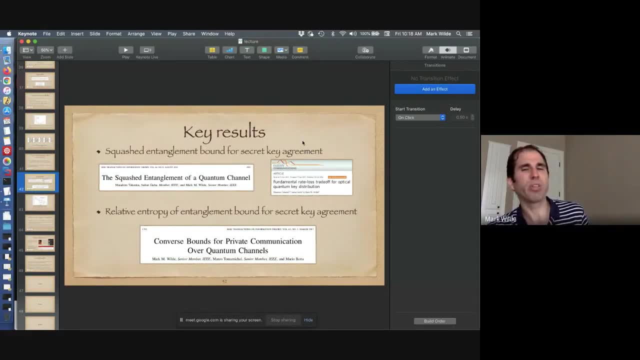 multi-party secret key agreement. you know, there's generalizations of quantum key distribution where you're trying to create secret key between multiple parties. um, there's a multi-part type squash entanglement and there's a multi-part type relative entropy of entanglement, and both are useful. so, um, 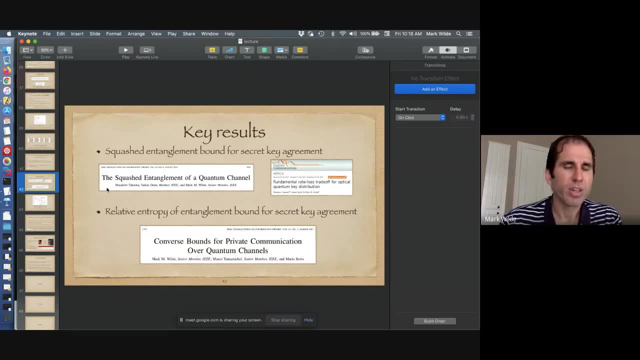 i mentioned kaushik stace, adrisan in masahiro takioka. we wrote a paper about multi-part type squash entanglement and using as the bound for secret key agreement over broadcast channels and uh. we've also written papers about multi-part type relative entropy entanglement. 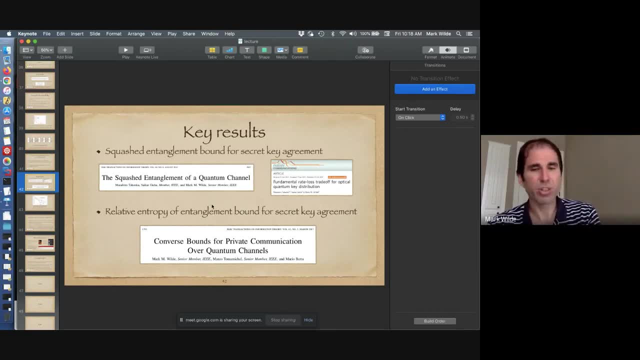 um, and that was also with masahiro and kaushik. so if you look up my name with uh, kaushik and masahiro, you'll find those papers. um, i could. i could send them via email if you'd be interested. oh, thank you, professor. that would be useful, um. 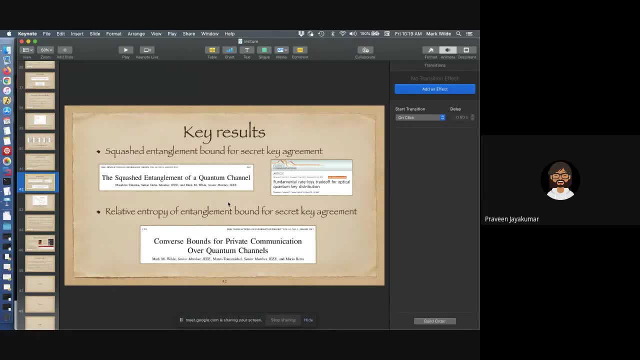 so, uh, so i'd like to thank uh professor mark weill for this amazing talk. uh, and, on behalf of ieee comsoc society of iaac, i'd like to present this uh play now to you as a token of our appreciation for taking out the time from your busy schedule. deliver such information. 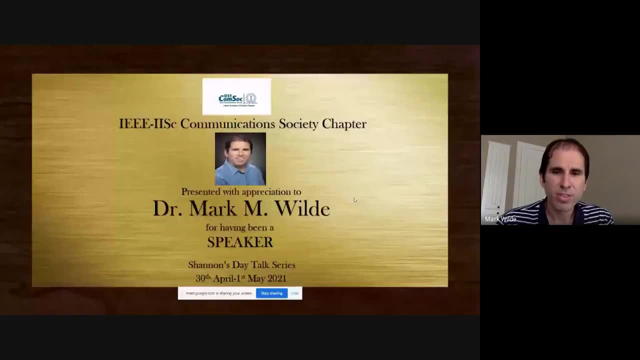 thank you. oh, very nice, thank you.